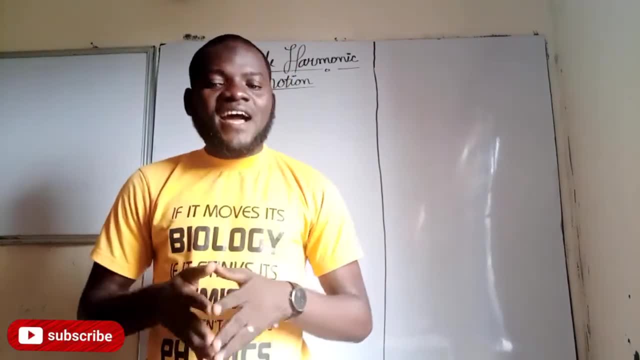 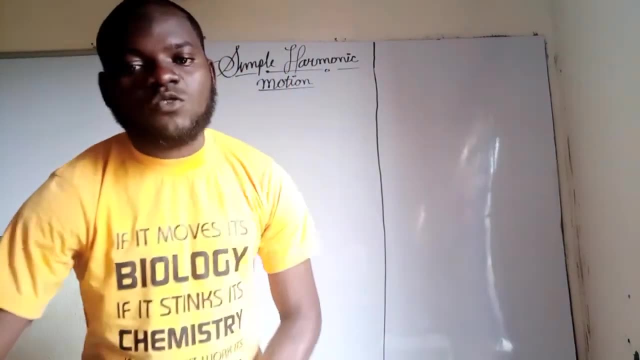 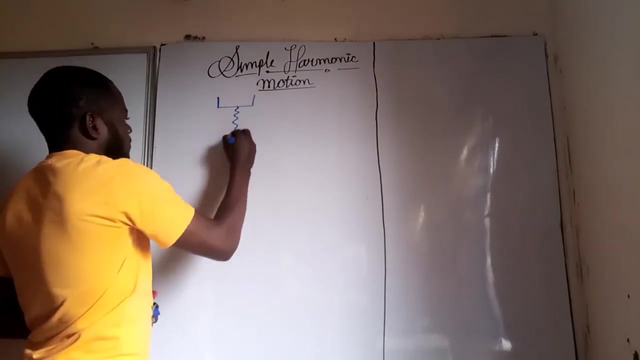 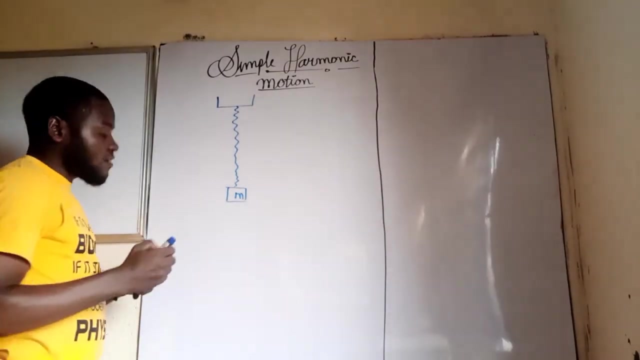 under the simple pendulum. But in this class I want to talk about the mass-spring system. Now let's see what we call a simple harmonic motion. If I have a string like this, So I have a mass attached on the string and the equilibrium position of the string is here: 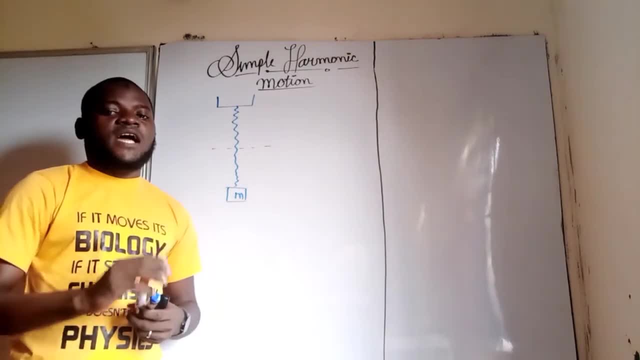 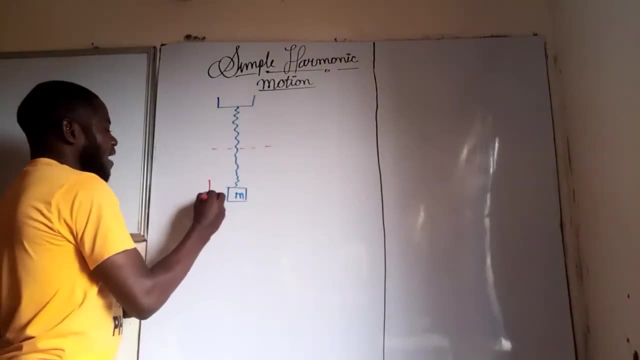 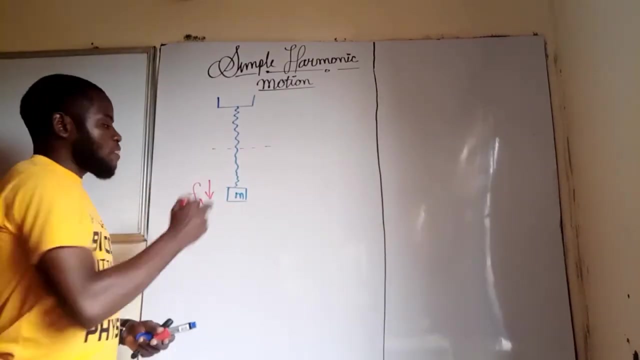 Now let's pay maximum attention so that we understand what we call a periodic motion. Now, when I apply force to this body, the applied force is taking the body downward. Before releasing this mass, there is a certain force, known as the restoring force, that wants: 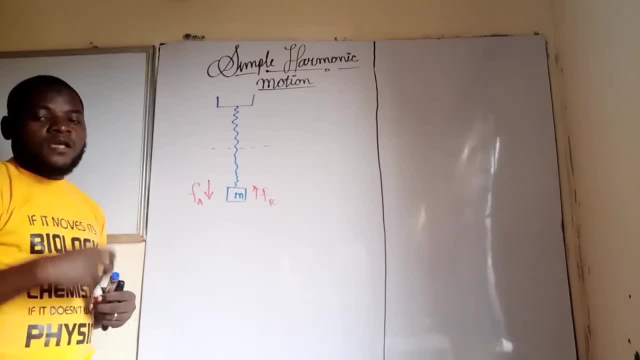 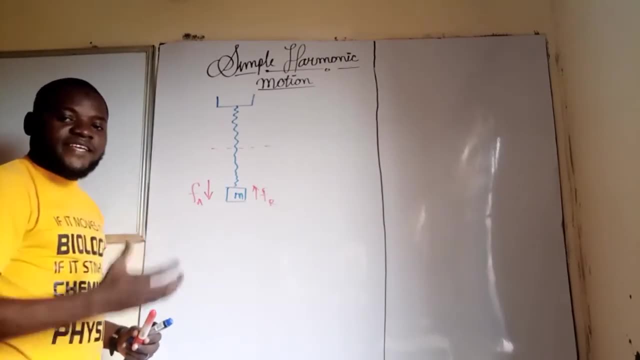 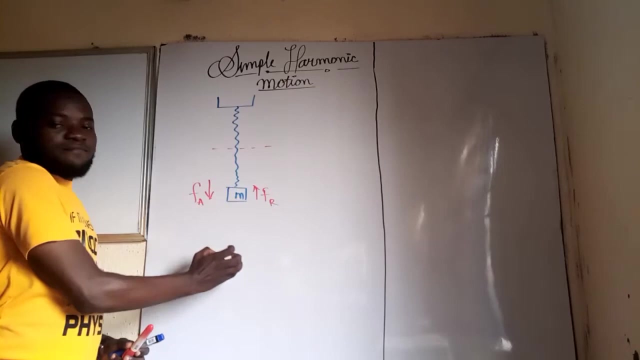 to take this body back to the equilibrium position. You know the applied force is taking the body away from the equilibrium position. The restoring force is ready to take the body back to equilibrium position Now, by the time I release this mass, the restoring force is going to take the body. 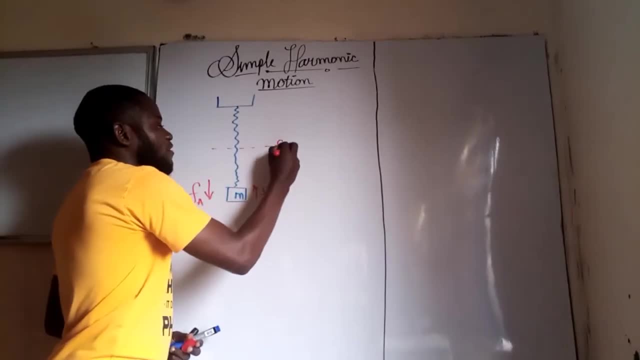 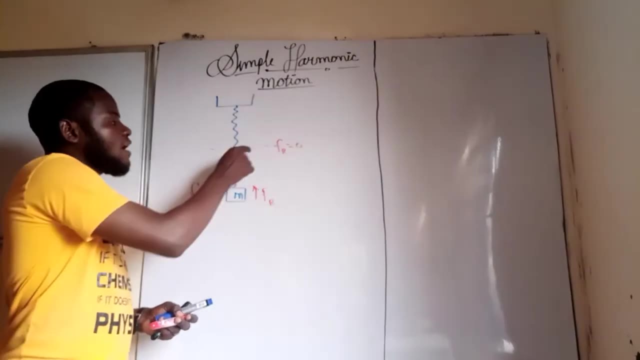 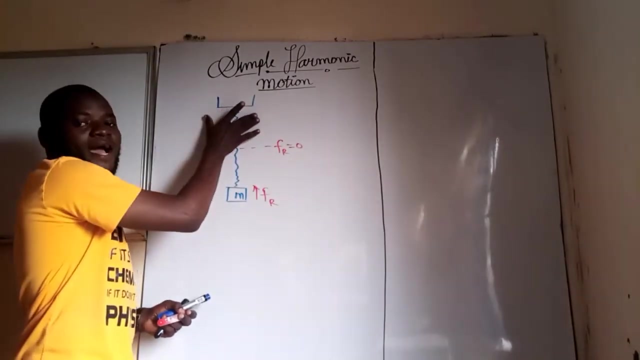 back to equilibrium position. and once it gets to equilibrium position, the restoring force becomes zero. But because this body has a mass and it also has velocity, momentum of this body is going to push it backward. When it pushes beyond the equilibrium position, the restoring force is 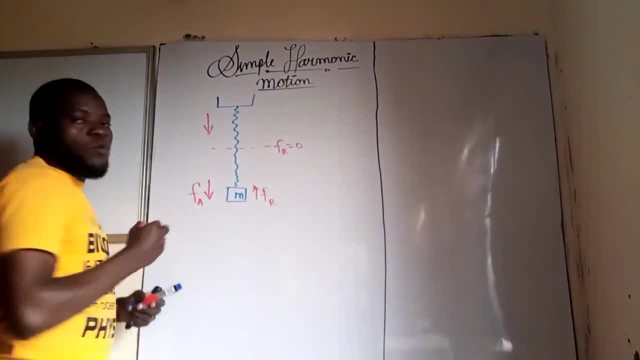 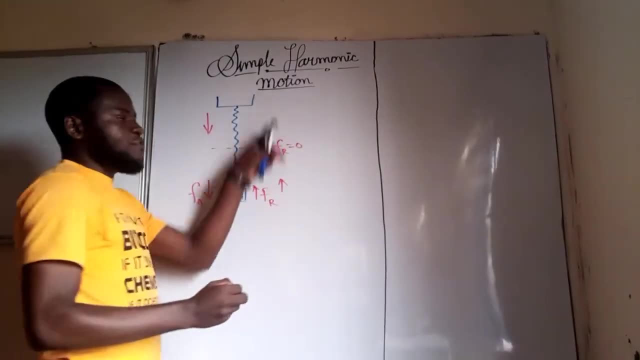 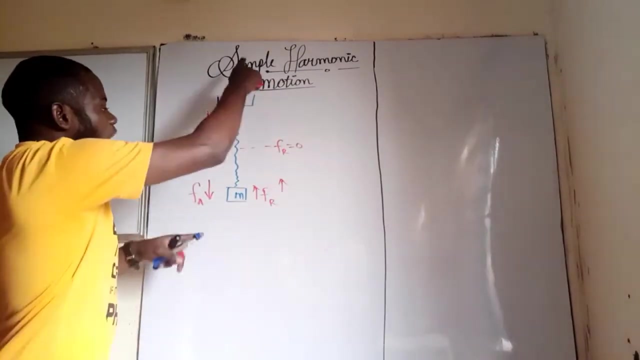 going to build up again to push the body downward. So when the restoring force pushes downward, it's also going to what Build it upward again. So when it pushes upward again, it's still going to push it backward. The toe and front movement is what we call the periodic motion. 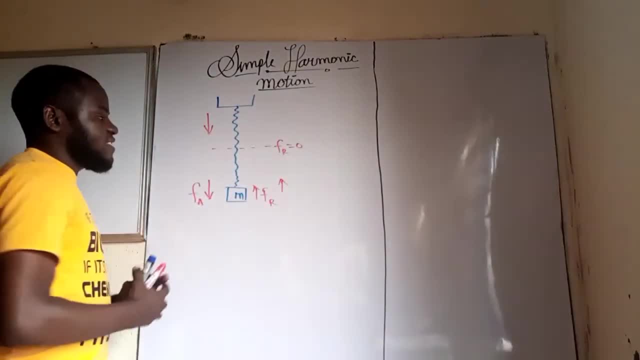 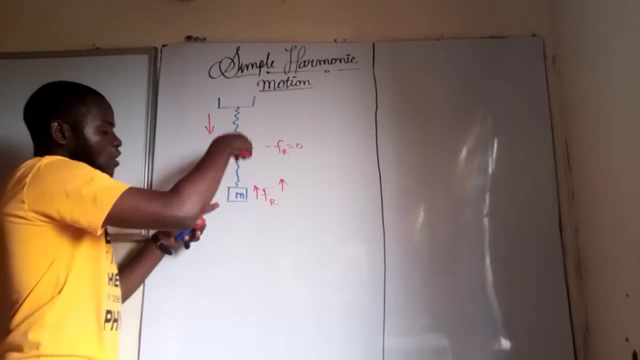 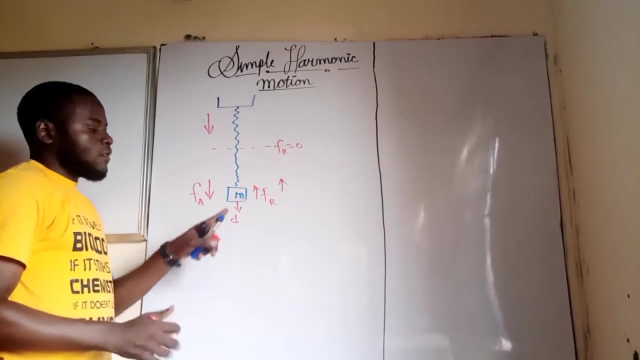 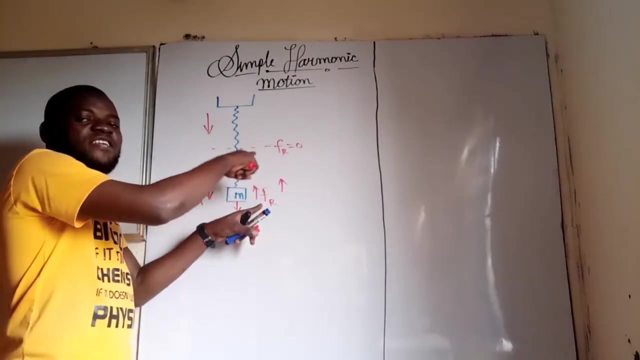 So now let us understand something about this body. now, if i apply this force on this particular body, the body is pointing in the downward direction, which simply means that the displacement vector is facing downward and the restoring force is facing upward. automatically, the restoring force is moving in opposite direction to the displacement vector, as we have that. 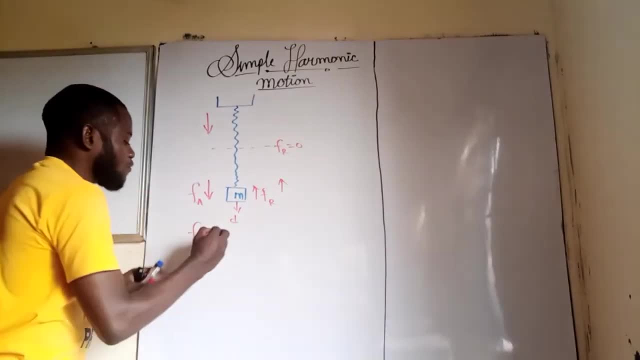 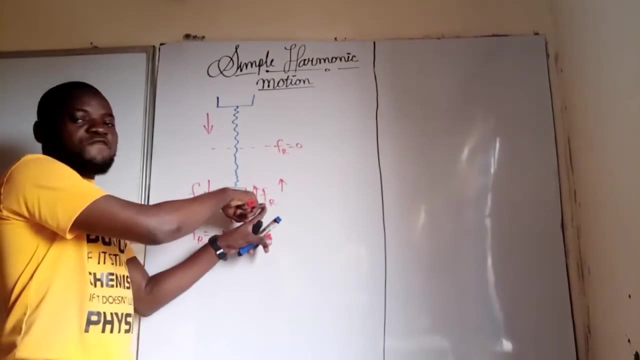 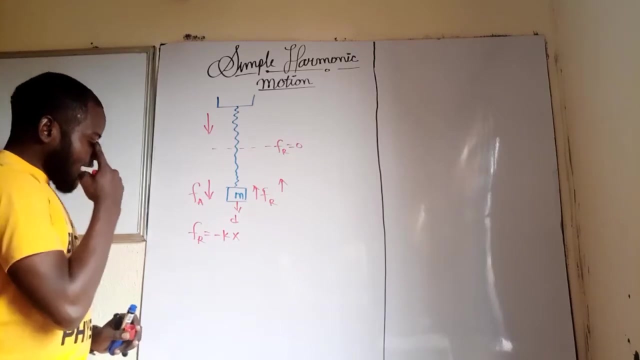 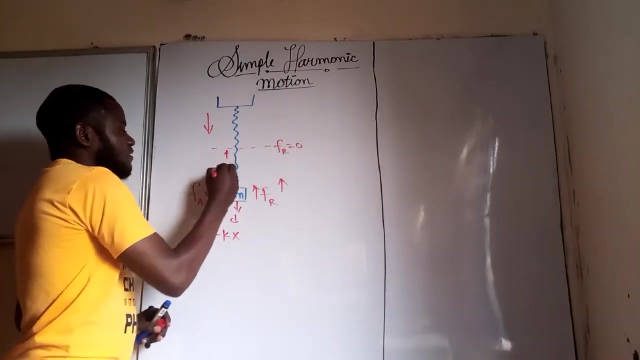 f, which is the restoring force from hook's law, to be negative. kx. the negative is to tell you that the restoring force is moving in opposite direction to the displacement vector. now let's get something clear here. what is the significance of x? x is said to be the displacement from the equilibrium position to the current position. 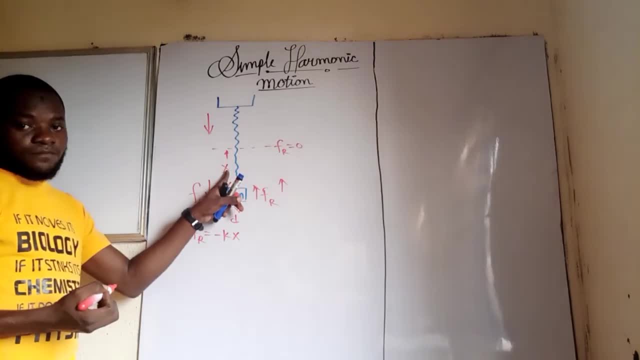 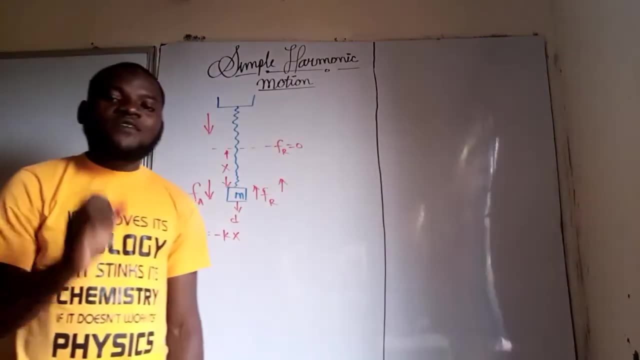 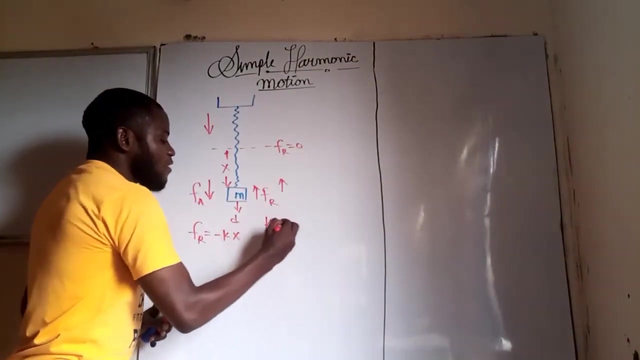 in other words, we call this one extension. now, what is k? k is force constant. first constant simply means a unit force that will cause a unit extension on the string. now let's take, for instance, that the k, which is the first constant, is 20 newton per meter. 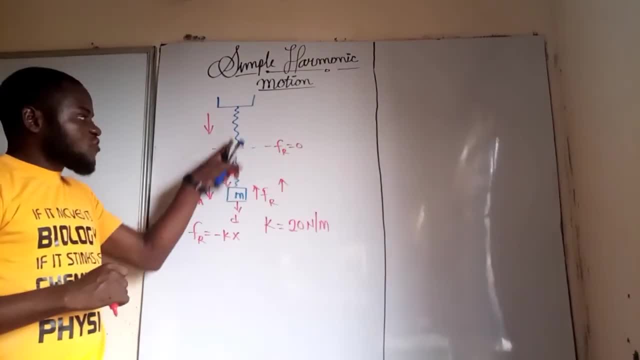 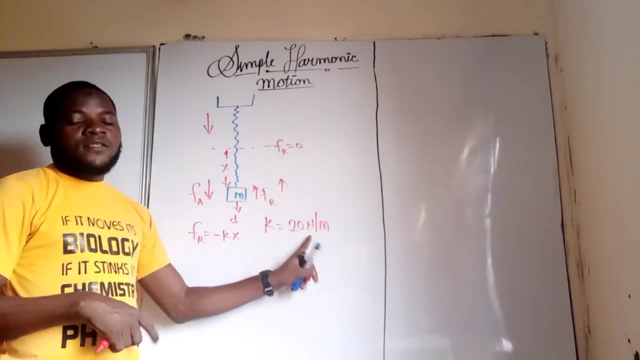 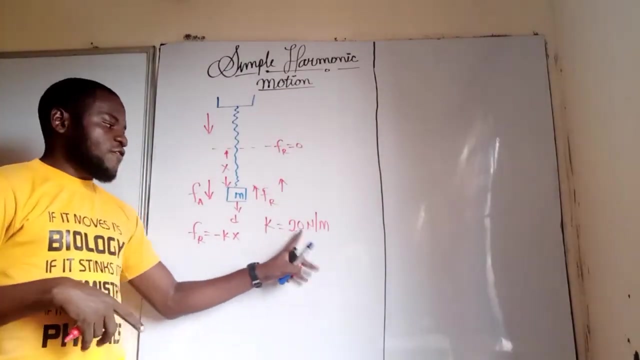 what this simply means is that for us to what stretch this particular string, or to compress it by one meter, we need a force of 20 newton. for you to compress it by one meter or you extend it by one meter, you need a force of 20 newton if you have to double the extension or the compression. 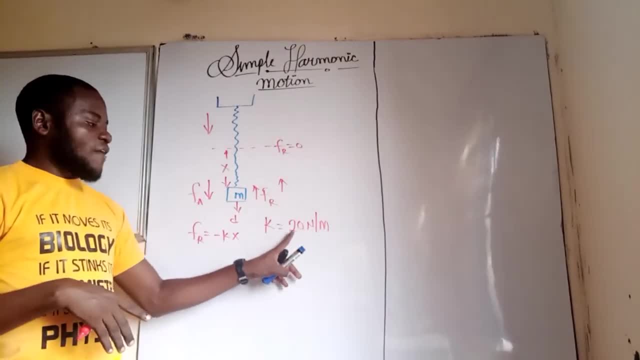 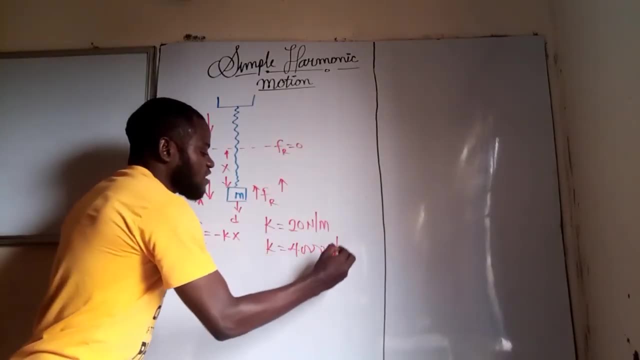 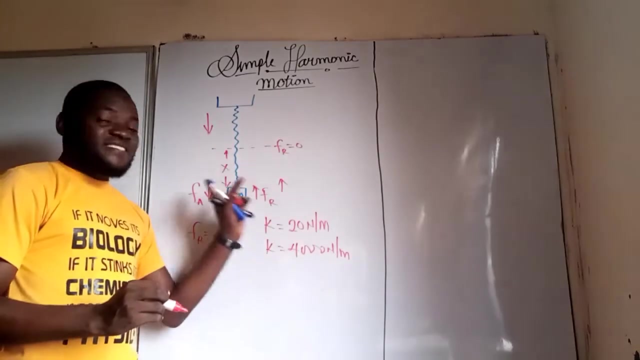 you need a force of what? 40 newton, that is. you also have to double this. now, if i now have that, the string is about 4 000 newton per meter. this is a very high word steepness. that is, if i will compress the string, whose first constant is 40, 4 000 newton per meter. i need a 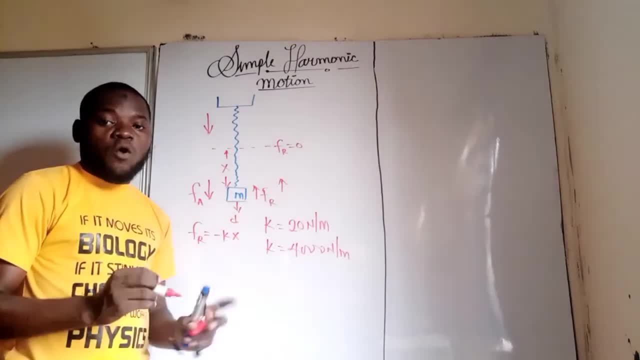 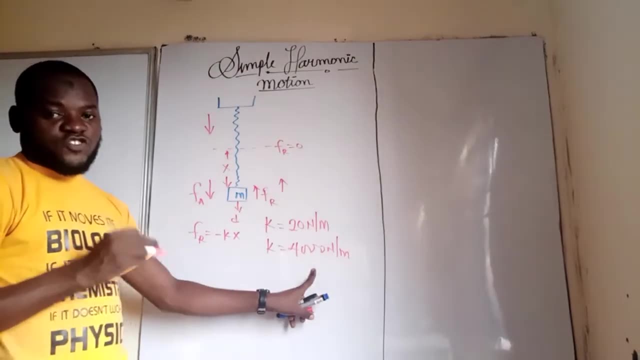 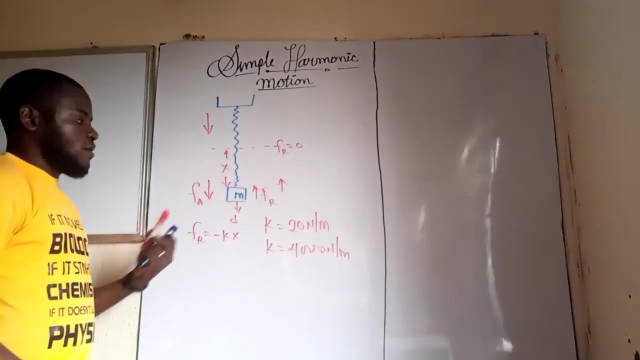 force of 4 000 newton to compress it by one meter or to extend it by one meter. hence you will see that this is a stiff string and this one is a long string string. okay, class now. let us now discuss something else regarding this particular 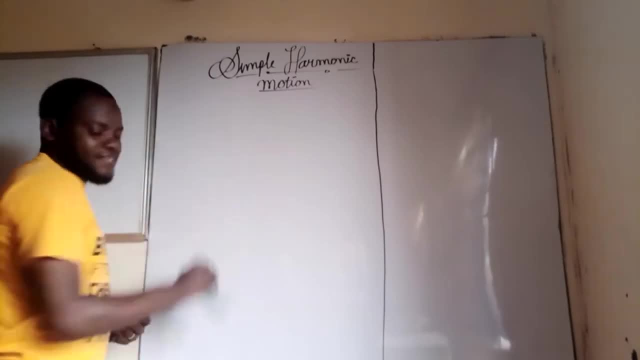 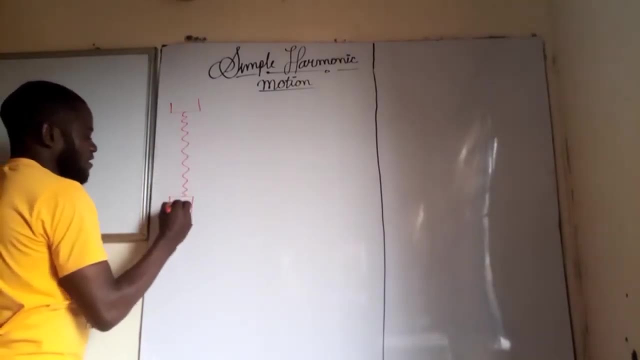 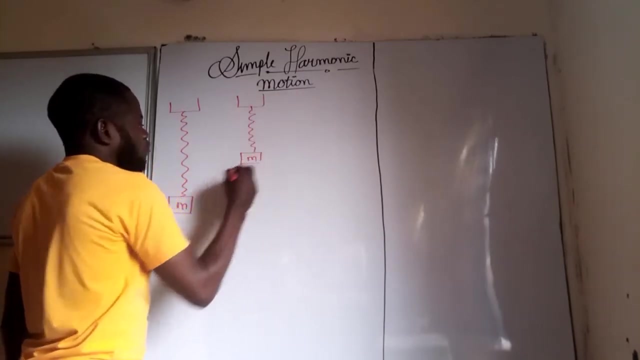 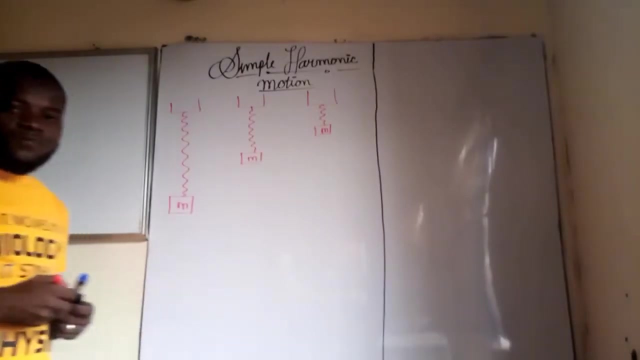 motion which were regard as mass string system. so if I have this, let's say: I have this and this is mass n and I have this, this is also mass n and I have this and this is mass n. now let's say: this is the equilibrium position let me use 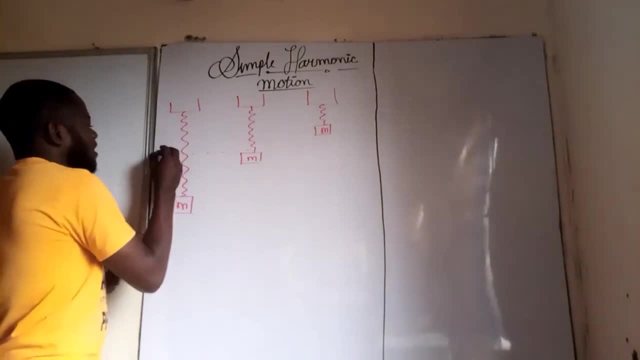 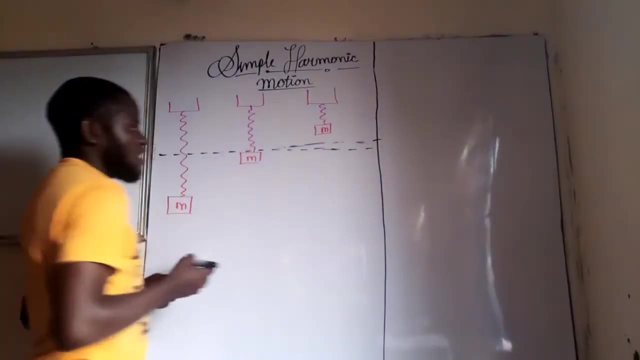 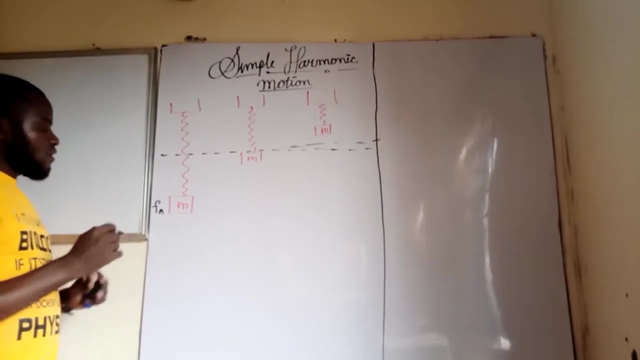 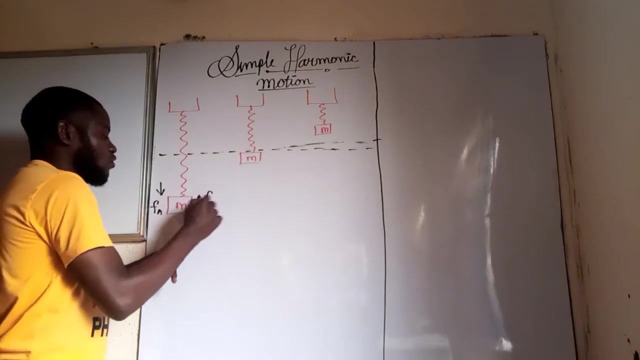 another column for better understanding. if this is the equilibrium position of the string, if this is the epilibrom position of the string, when I apply force F a to this body, the force is pointing downward. okay, and a force is ready to take the body back to the epilibrom position. that 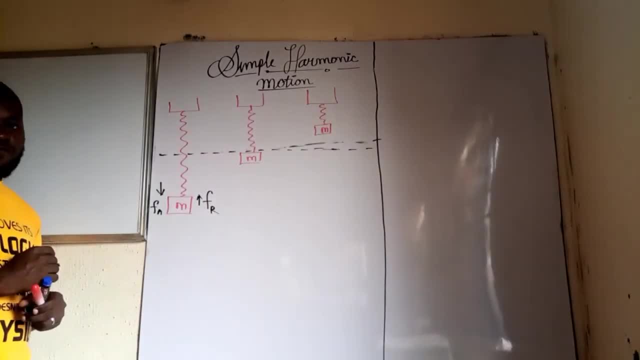 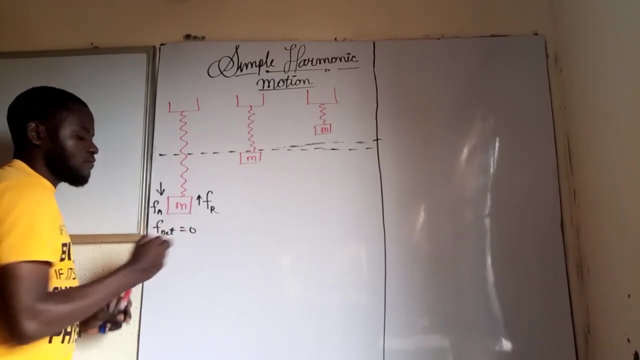 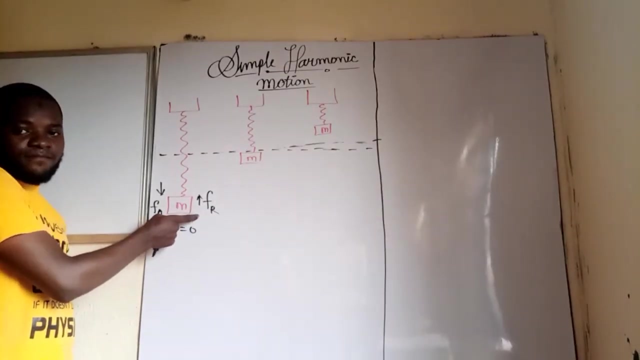 force is the restoring force. now, watch, as at this time that I'm yet to release this body, the total force on this system, that is, the net force on the system, is zero. why? because the applied force is equivalent to the restoring force at this moment. now, by the time I release the body, the applied force said: 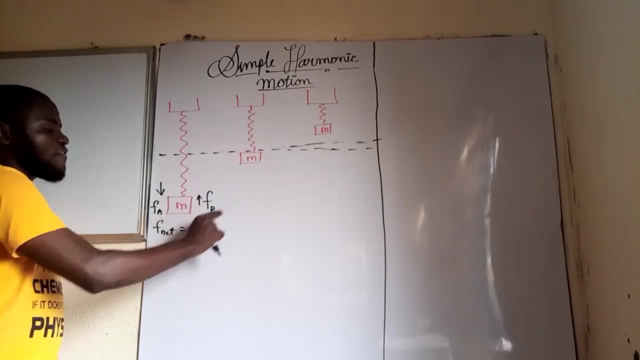 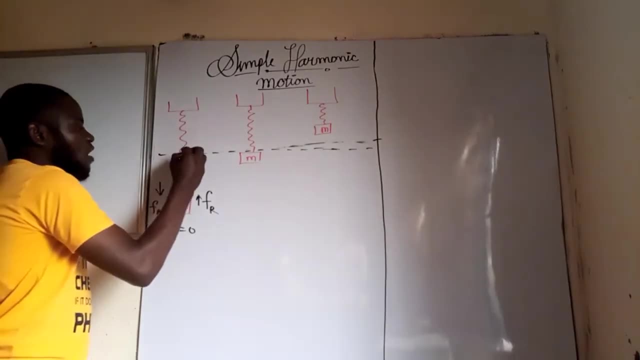 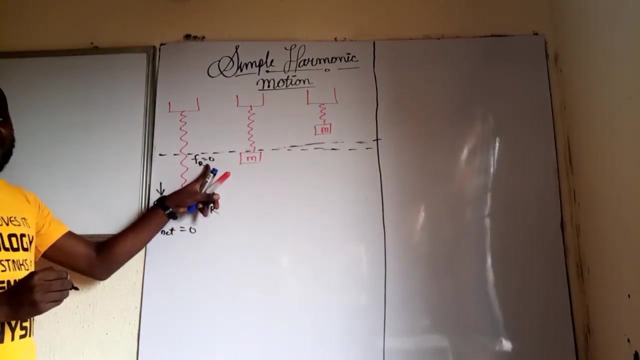 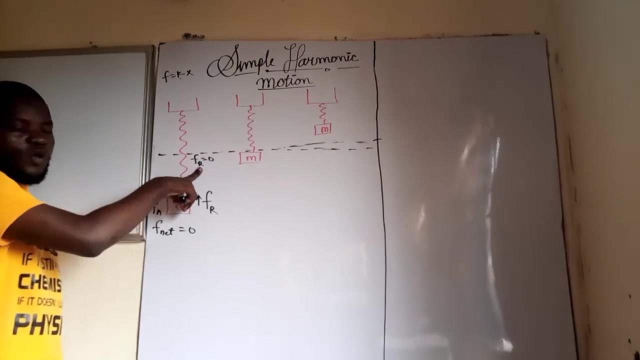 to disappear and I'm going to have my restoring force only to take the body back to equilibrium position. so when the restoring force get back to the epilibrom position it becomes zero. why? because the displacement X is equals to zero and you know the restoring force is K X 0 times k. give us 0 that. why this? 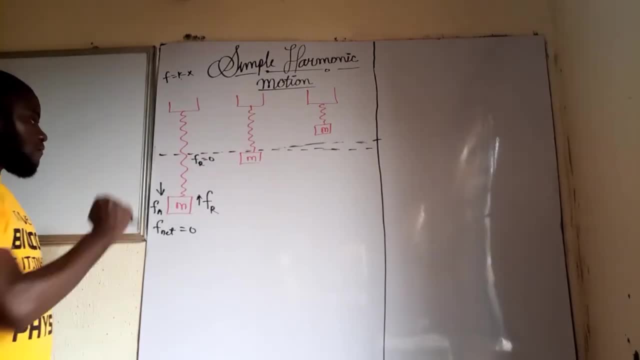 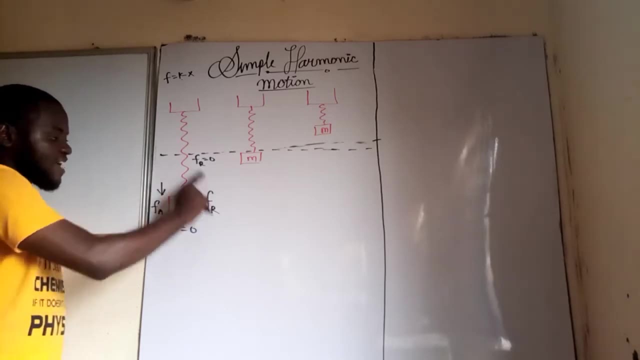 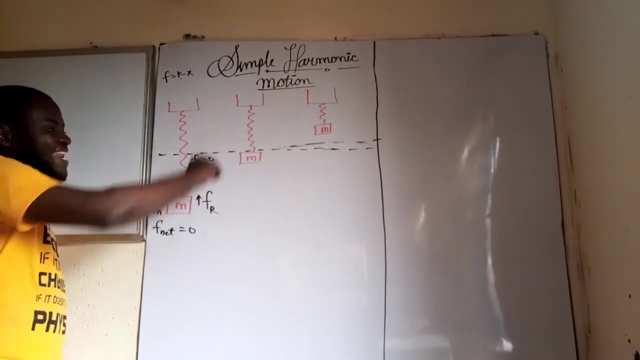 is 0 here. now. watch by the time this body becomes 0. that is, before I release this mass. the O of the force in it is equals to 0. when I release the mass, the applied force will disappear. the total net force on this system is going to be the restoring force. when the restoring force 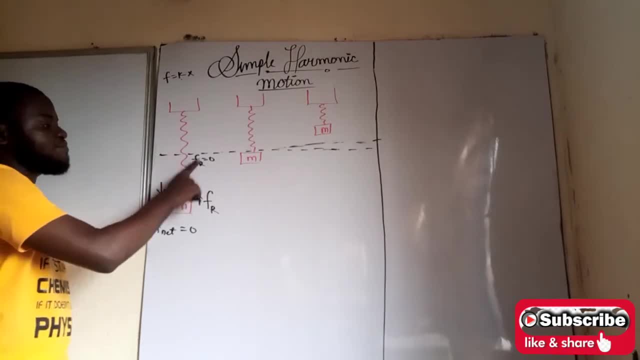 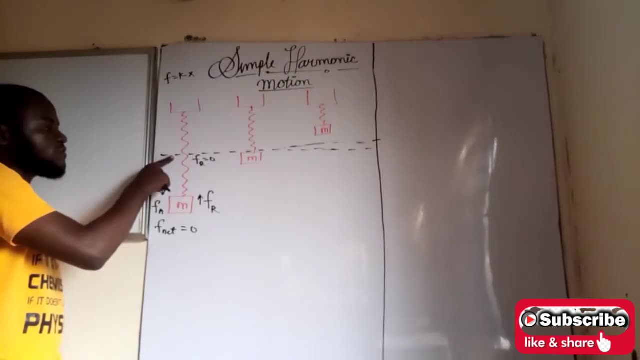 gets to the center- that is the equilibrium position- it becomes what? Zero. Then momentum is going to take the body, because the force is already zero. Momentum is going to take the body from this equilibrium position to compress When the body compresses this force. 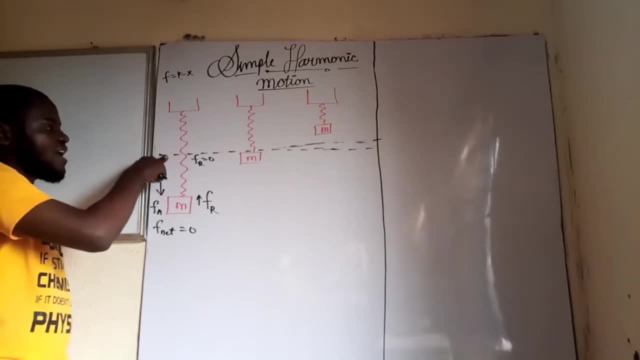 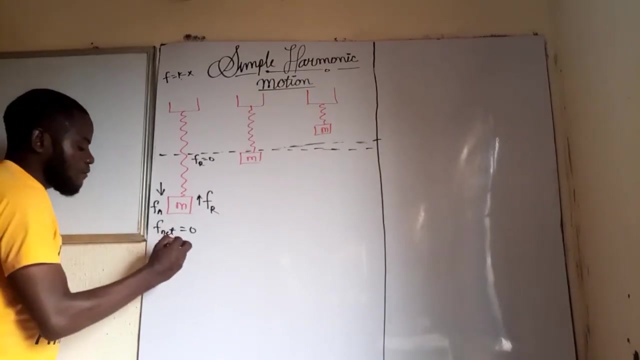 is set to build up again, to push the body towards the equilibrium position again. So if this should be the case, at this point we have that our displacement is maximum. When displacement is maximum, we call it what Amplitude. Now you will agree with me that 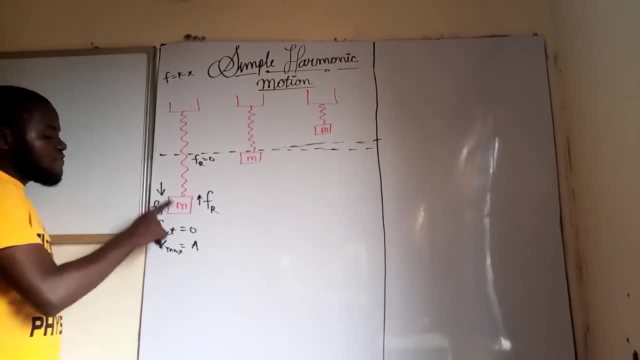 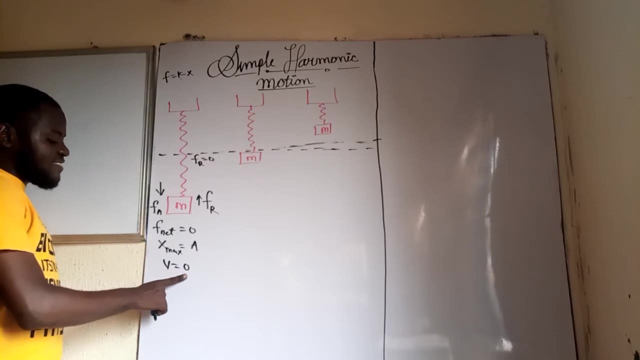 initially, when we have not released this body, the velocity of this body is zero. Are we together? If the velocity is zero and we have our displacement to be maximum, our amplitude, our angular velocity, should be equal to zero And we have our displacement to be maximum. 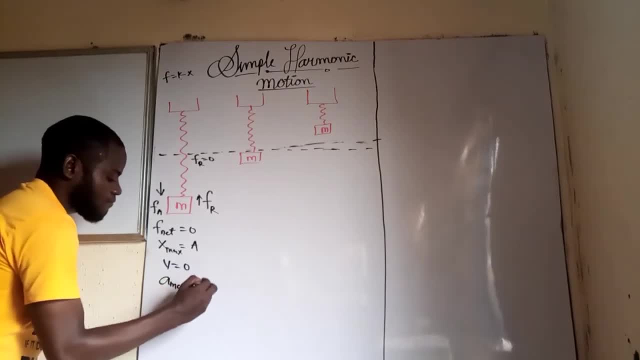 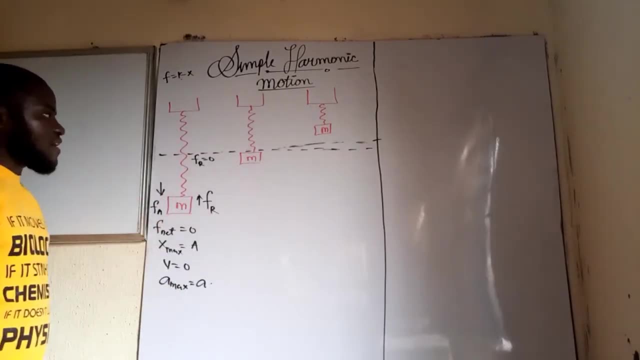 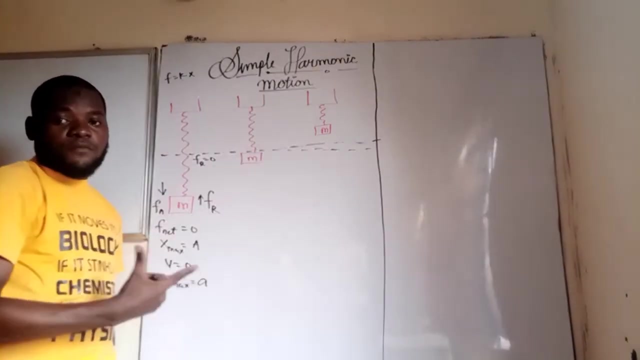 when we have not released this body, the velocity of this body is zero, So now we have to place. acceleration would also be maximum. are we together? if we are together, let us move down to the second body, whereby the body is at equilibrium position. the second body is at equilibrium right. this one extend, that is, we stretch this one. 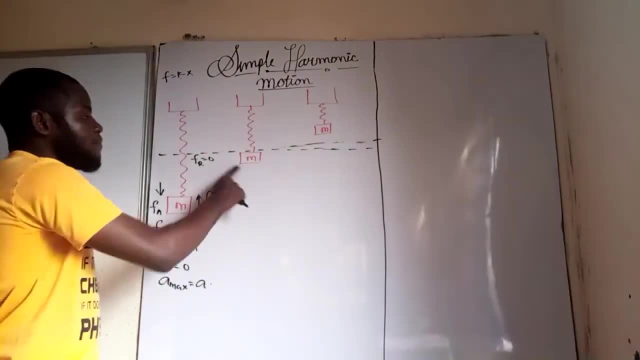 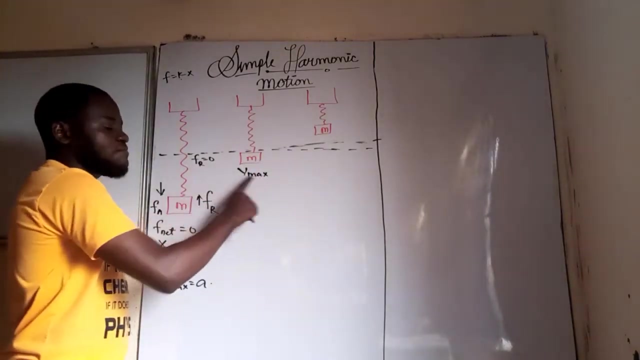 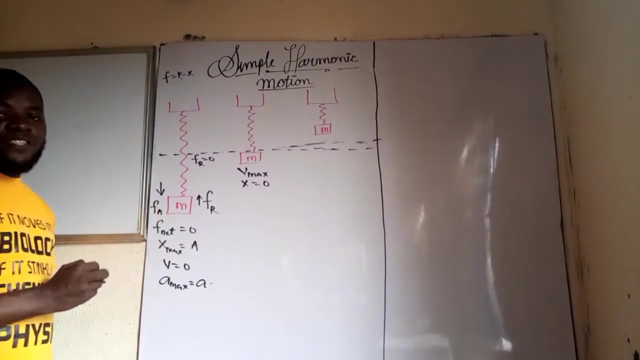 and this one is at equilibrium. at the equilibrium position, remember, the restoring force has provided a velocity. now the velocity of this center is set to the maximum. if the velocity is maximum at this center, then we are going to have our displacements to be zero. if displacement is zero, acceleration is. 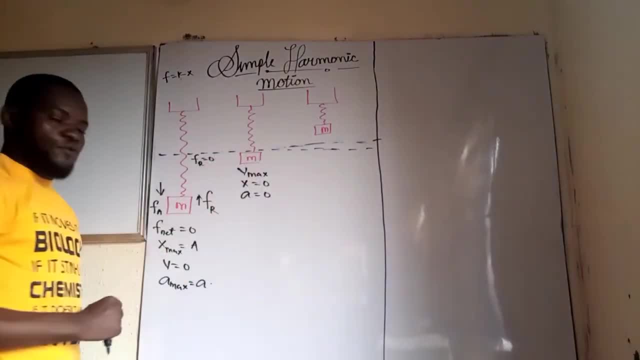 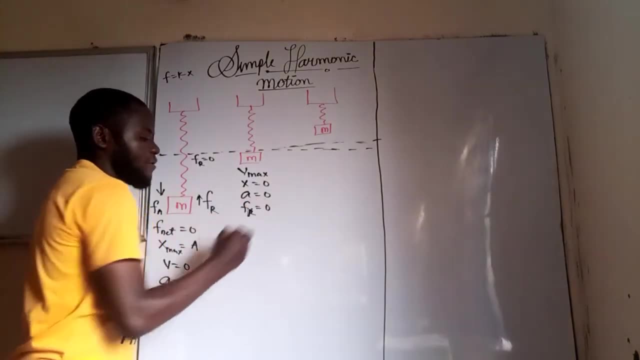 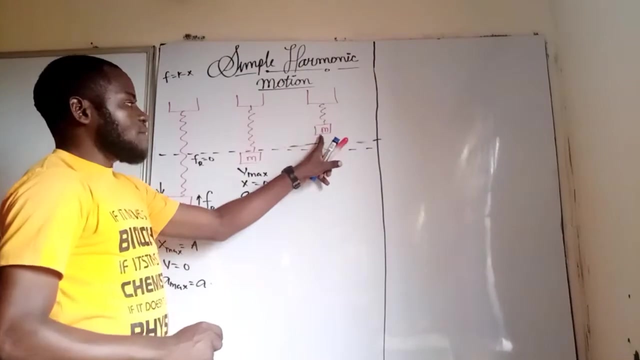 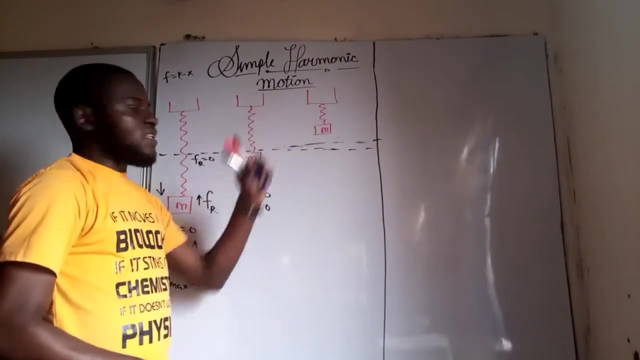 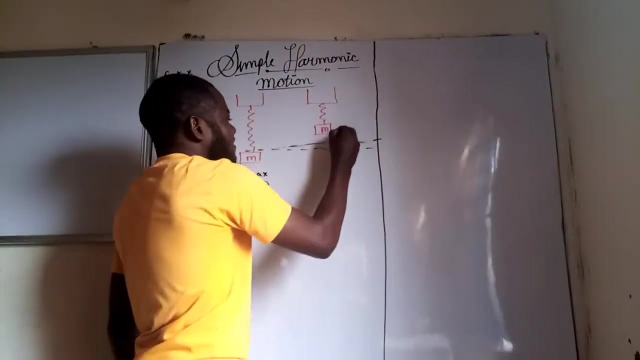 also zero at this equilibrium position. remember, our restoring force is also going to be zero at the equilibrium position now when the body compress. by the time the body compress, remember it is the momentum that cause the body to compress. when the body compress completely, the restoring force is set to build up again to push the body downward. hence our x at this place. 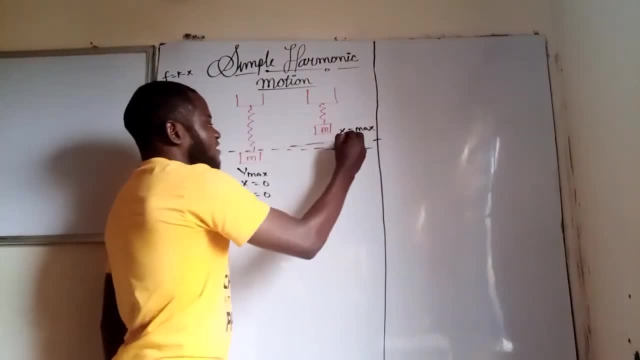 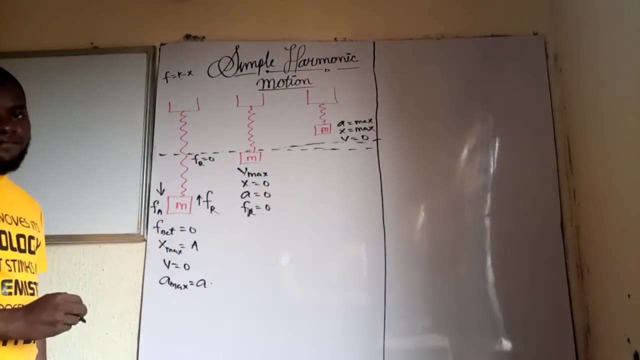 is also maximum and our velocity has become what zero is. we also have acceleration here to be maximum. so if this should be the case, we can then talk about the energy of this system. remember your kinetic energy is a function of velocity. so we have kinetic energy to equal 1 over 2 m. 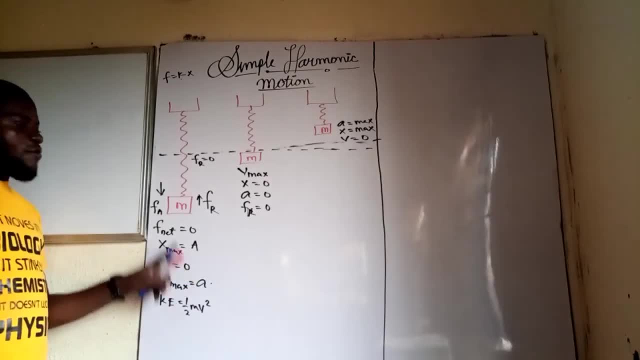 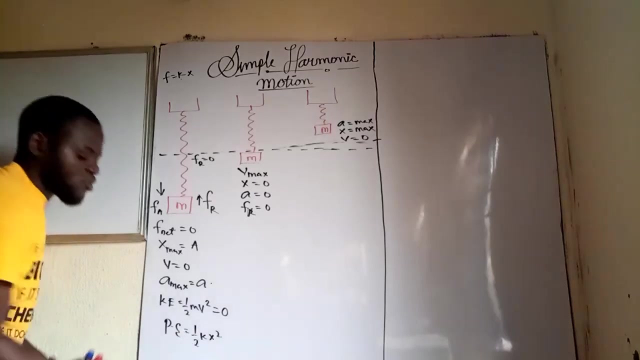 V square. now, if V is equals to 0, at this point kinetic energy is set to be zero, and if x is maximum, we have our potential energy at this point to be 1 over 2 K x square. so it means that potential energy is present here, while 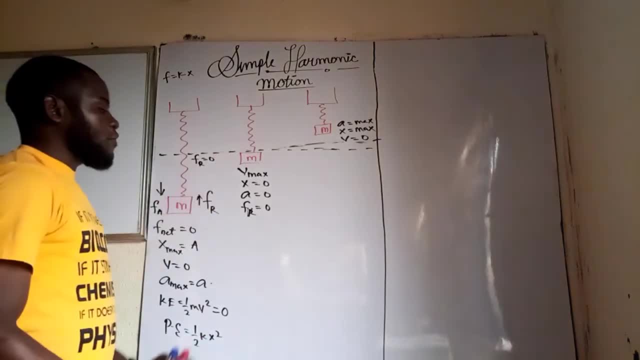 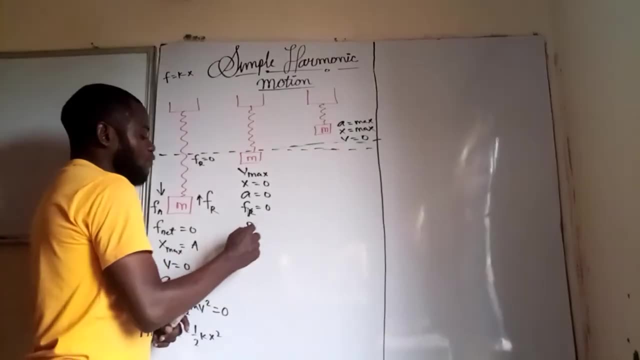 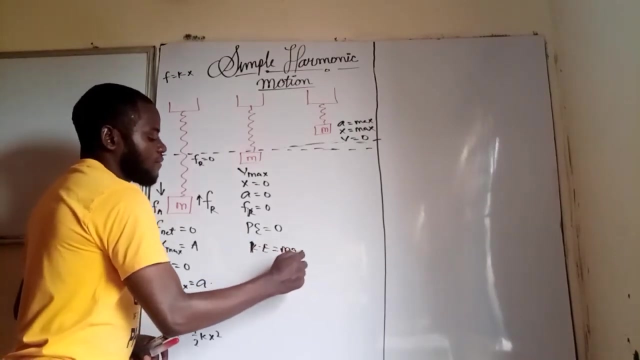 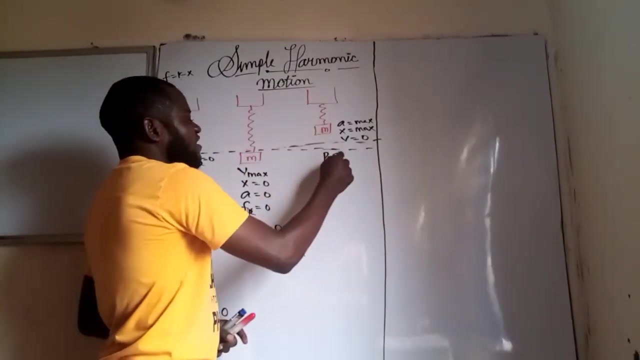 kinetic energy is zero. now, at the equilibrium position, the displacement is equals to zero, but we have our velocity to be maximum. hence potential energy is zero, our kinetic energy to be maximum at the equilibrium position. and here, when the body fully compressed, potential energy is maximum, kinetic energy is zero. so 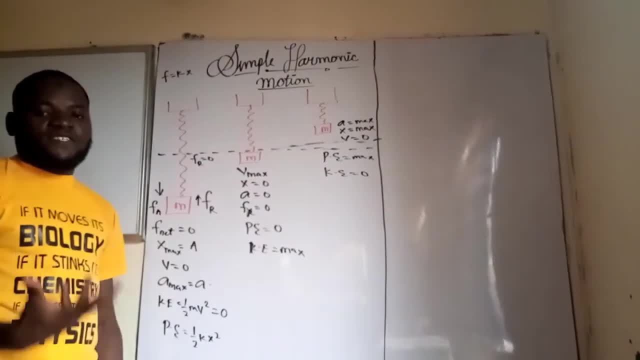 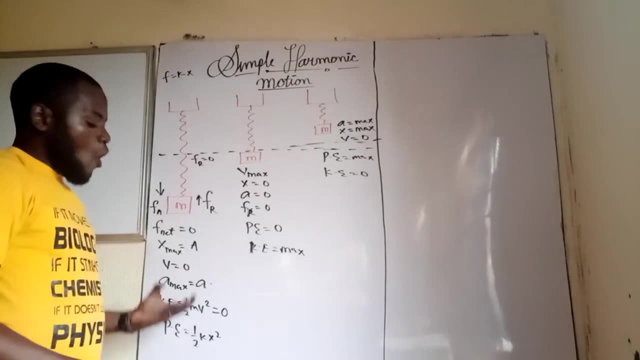 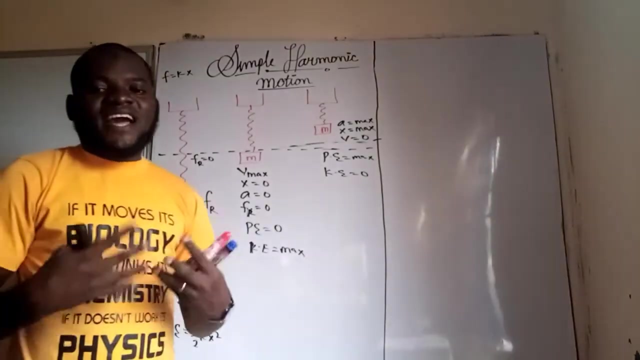 with this we can talk about the total energy of the system and what to be the total energy of the system? the total energy of the system is going to be the summation of the kinetic energy and the potential energy, which is then going to equal to mechanical energy. remember, when X is maximum is equal to the 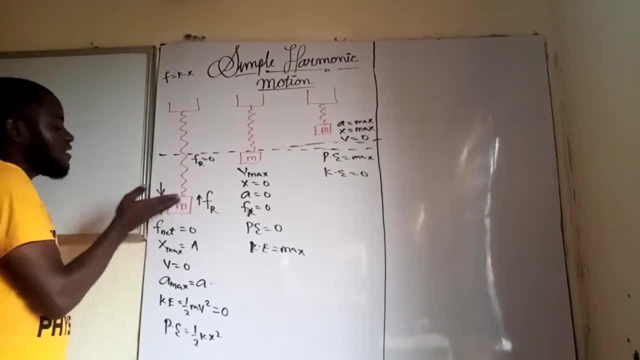 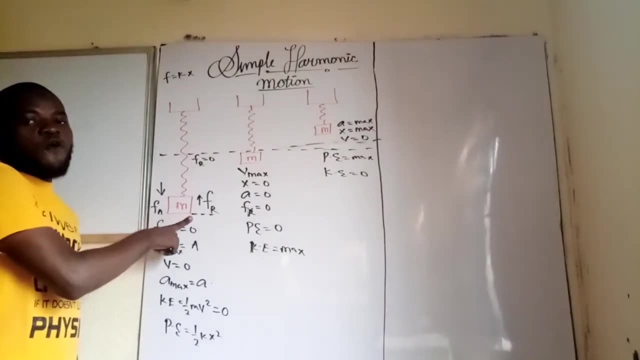 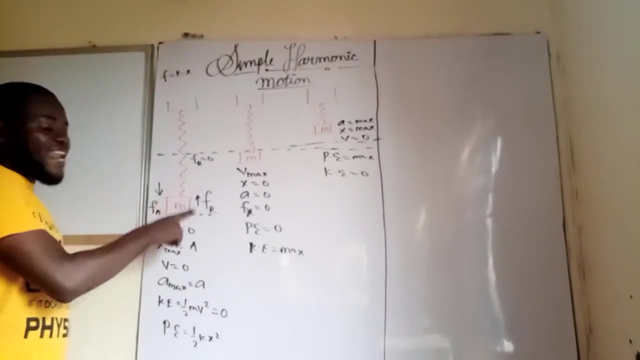 displacement by the time you release the mass. if this is the points at which you release the mass, this body will never get to this point again. if the law of conservation of energy is what is conserved in this place, you, that is, if energy is conserved there and the law of mechanical energy holds in this. 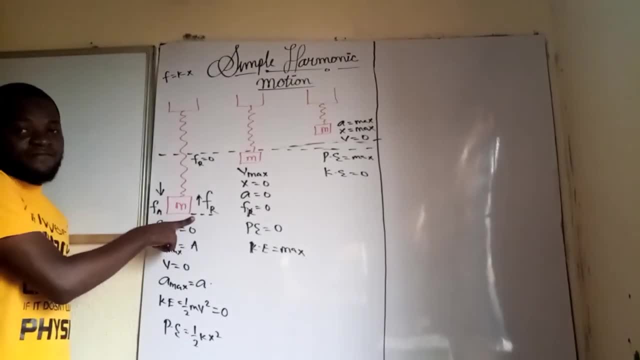 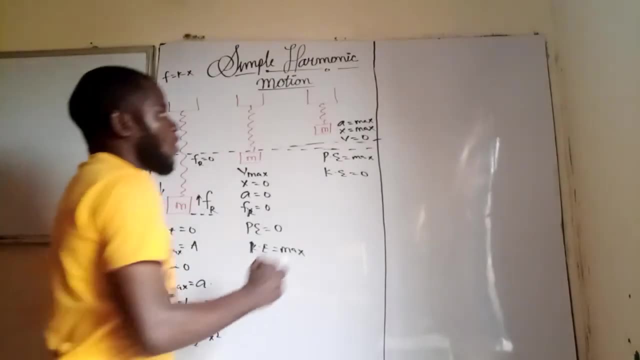 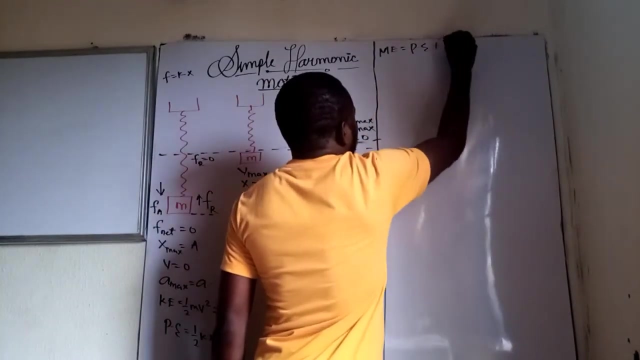 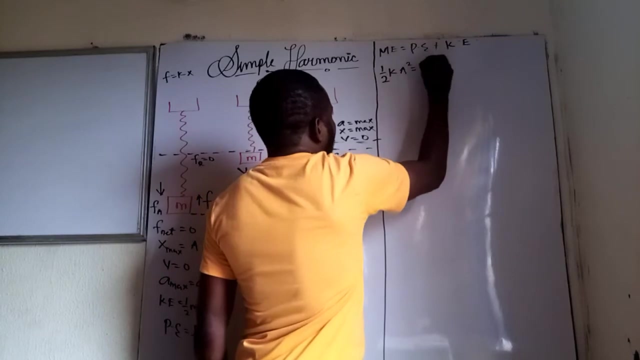 particular place. this body will not get to this point again. hence our mechanical energy is a function of amplitude. so we have that mechanical energy which is equal to potential energy plus the kinetic energy. so this will be 1 over 2 k a squared. potential energy is 1 over 2 kaj squared plus 1 over 2 mb squared. let's call this: 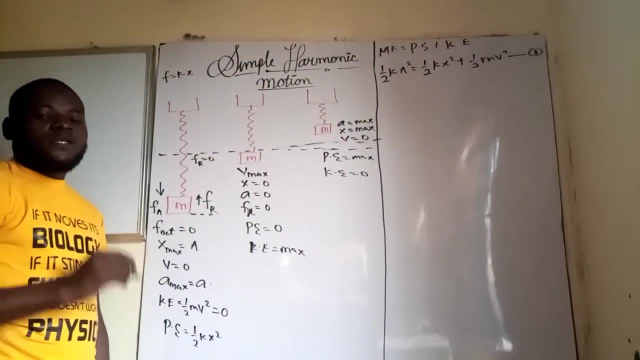 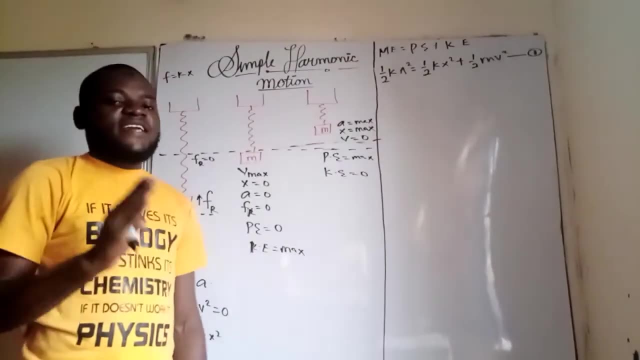 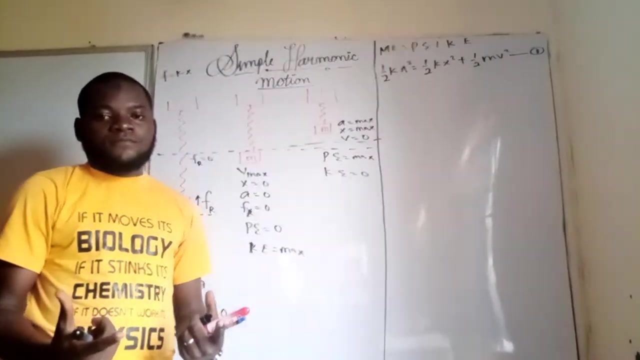 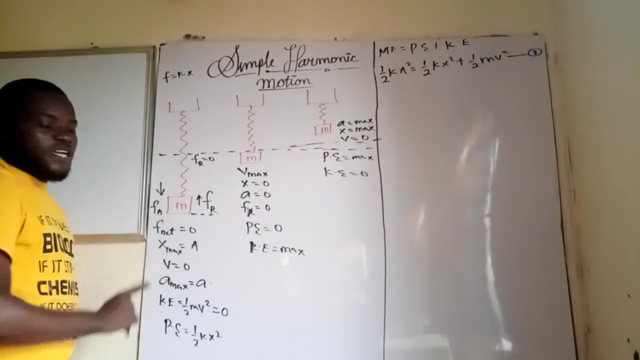 equation 1. now, let us now understand what happened at every instance. because if friction is not what involved, the mechanical energy of the system tends to be constant. so at this point, when x is maximum zero, the velocity is equal to zero. is, when X is maximum, the total energy of 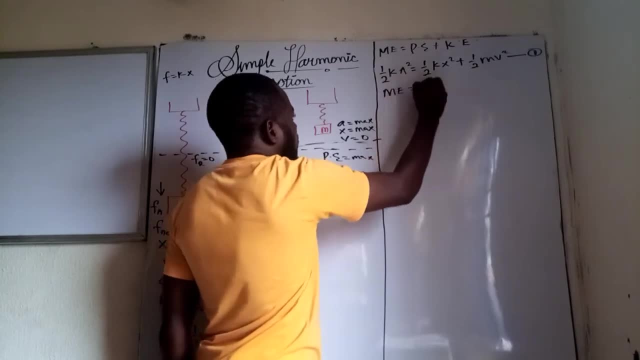 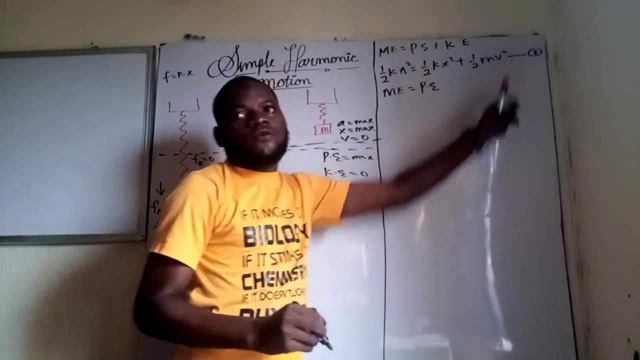 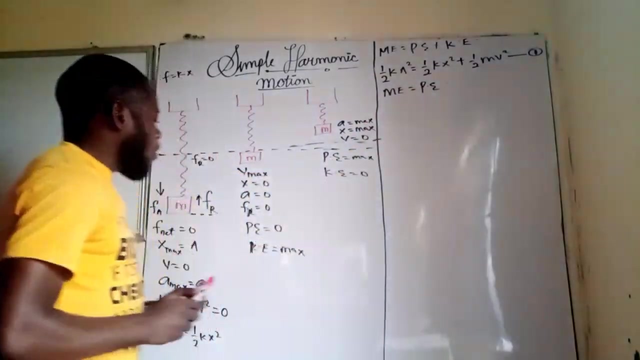 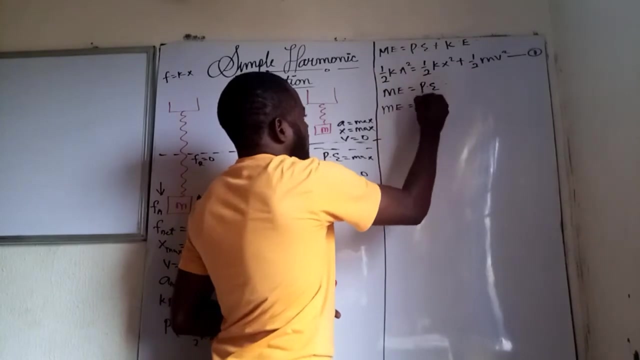 the system will mix mechanical energy to equal potential energy, because by the time you put zero here, this kinetic energy becomes zero. so when X is maximum, mechanical energy is equals to potential energy. now, when V is maximum, X becomes what zero is: mechanical energy is equal to kinetic energy. so let us note that. 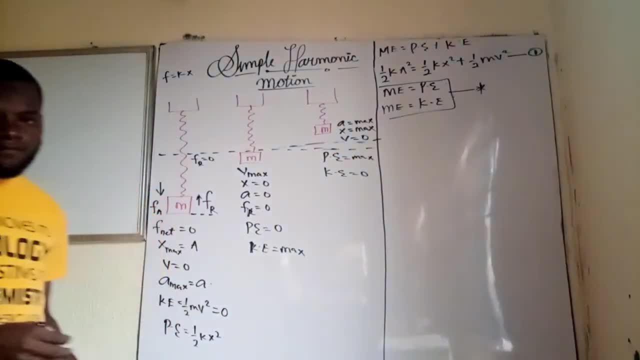 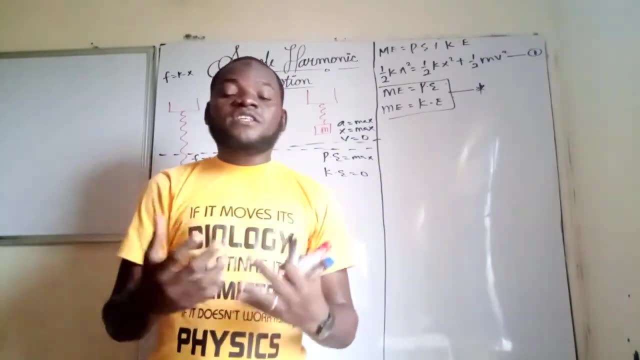 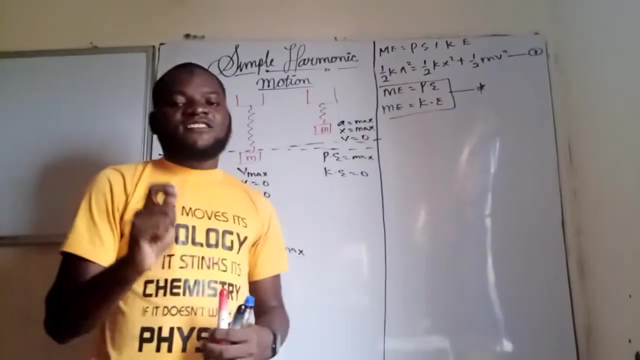 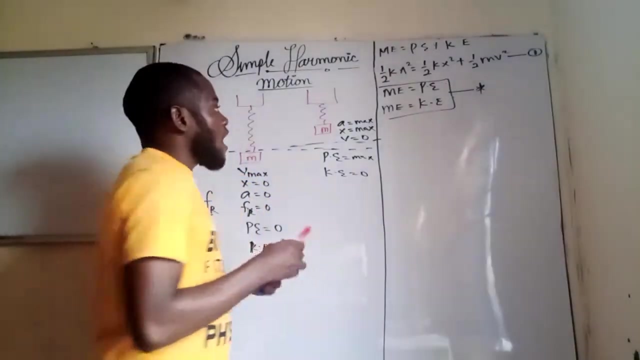 and call this equation star. now, you might now have interest to know the maximum velocity of this particular system. how can we get the maximum velocity? remember, when the velocity is maximum, the displacement is equal to zero, which is the maximum velocity of the system. so the maximum velocity of the system is equal to zero, which means the body is at. 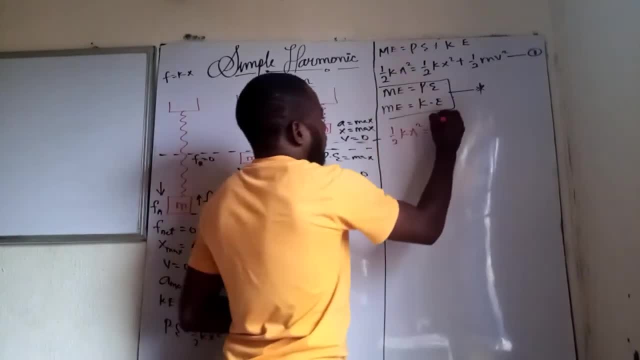 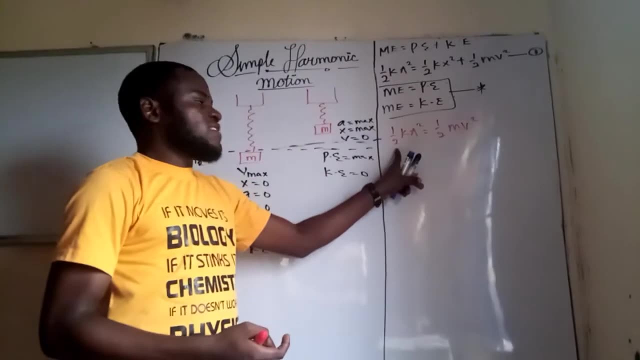 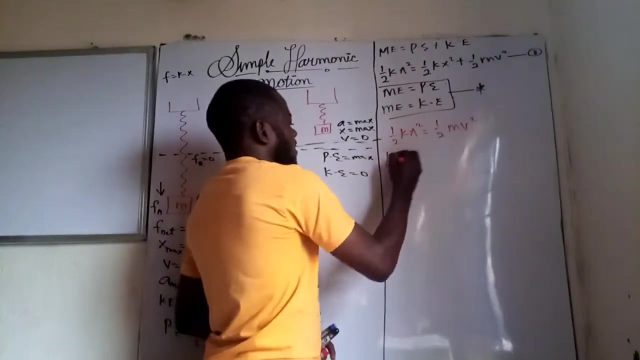 equilibrium position and I'm going to have this to be 1 over 2 k a square, to equal 1 over 2 m v square. so if I multiply both side by 2, 2 times 1 over 2 is going to give us 1, 1 times. this will give us k a square and this will also 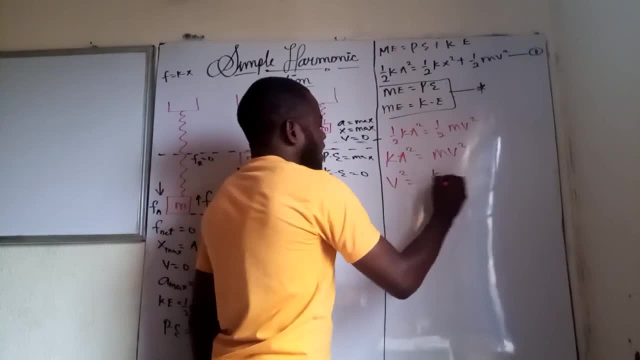 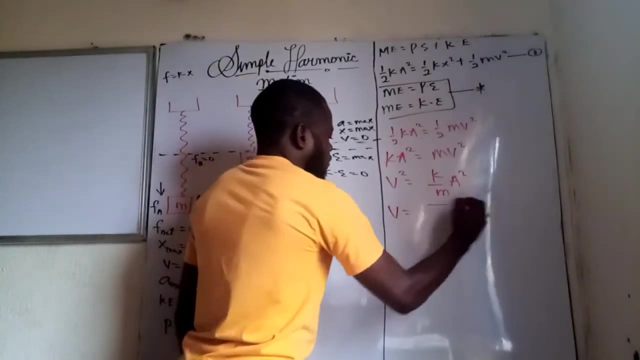 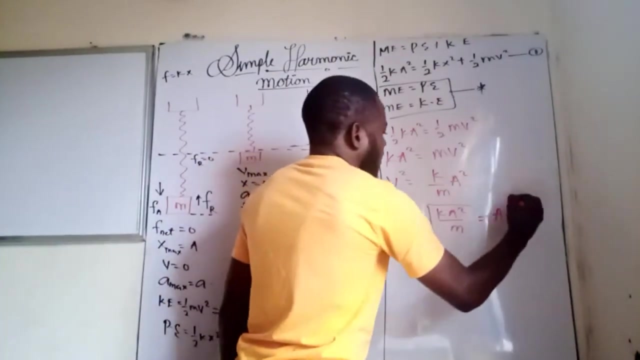 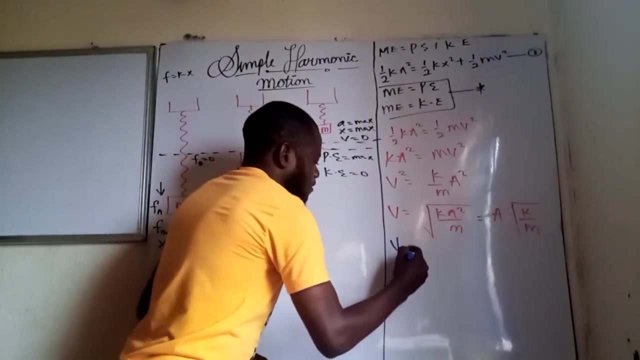 хence i have that v square is k over m a square, so i take the square root of both side. v is equal to the square root of k. a square over n and this is equal to a square root of k over m. hence our maximum velocity, the velocity mags, is equal to a root k over m. emo to Saints in the mark is equal to a drinking bar x k over m la. 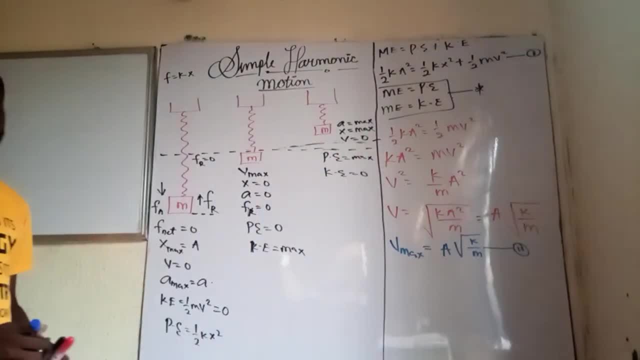 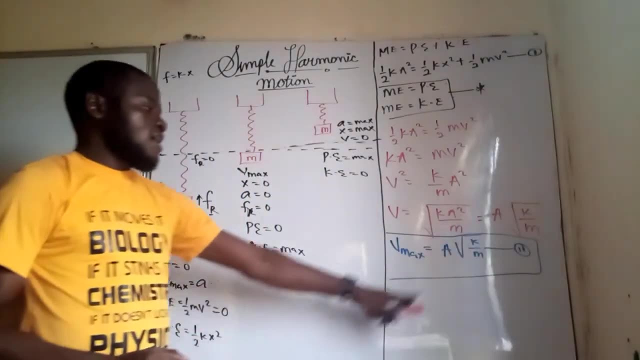 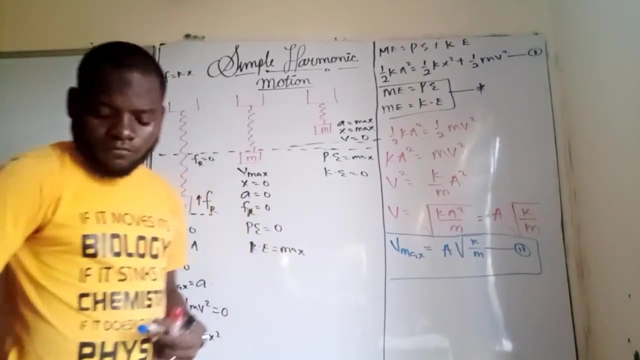 m. Let's call this equation 2.. So if you are looking for the maximum velocity of this system, the maximum velocity is amplitude times the square root of the spring constant divided by the mass. Now we might not be interested to know the maximum velocity, but 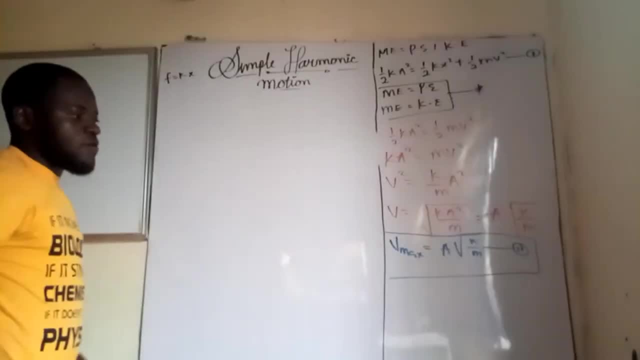 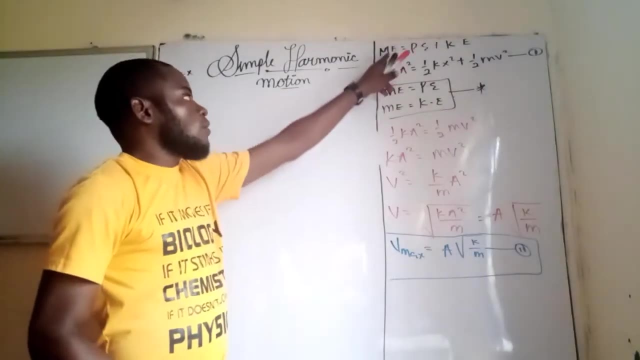 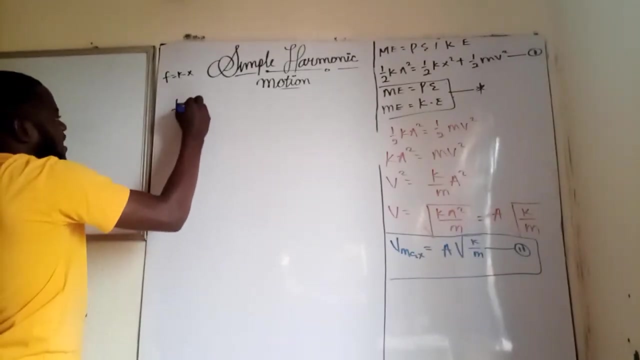 we want to know the velocity at every instance. How can we get that? Now let's see That is. the velocity of this time around is not maximum. Now let's go back to the initial equation, that is, equation 1, where we have 1 over 2 k, a square to equal 1 over 2 k x. 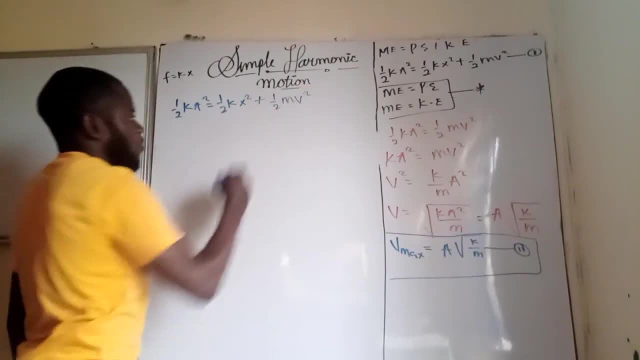 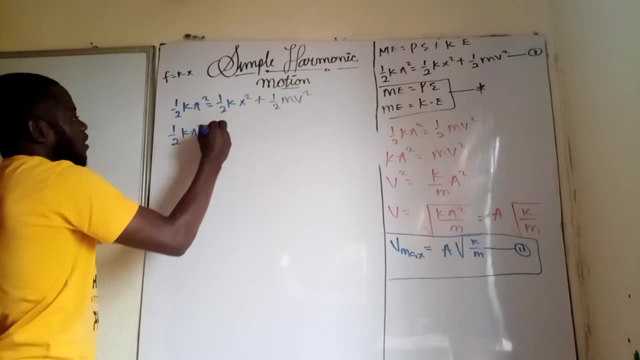 square plus 1 over 2 m v square. At this point, take this one to the other side. We have 1 over 2 k a square, minus 1 over 2 k x square, equal 1 over 2 m v square. Now let's see. 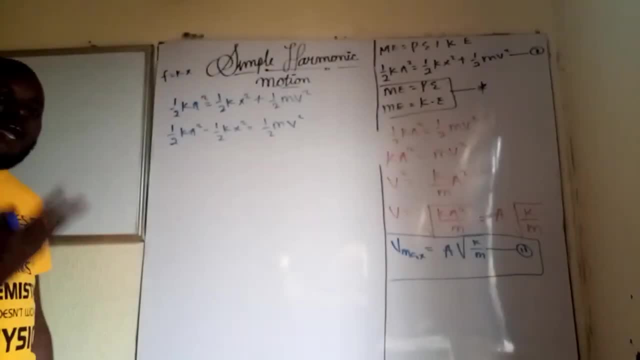 what we have here. We have 1 over 2 k a square, minus 1 over 2 k x square, plus 1 over 2 m v square. Guys, if you multiply it through by 2, we are going to have that k a square minus. 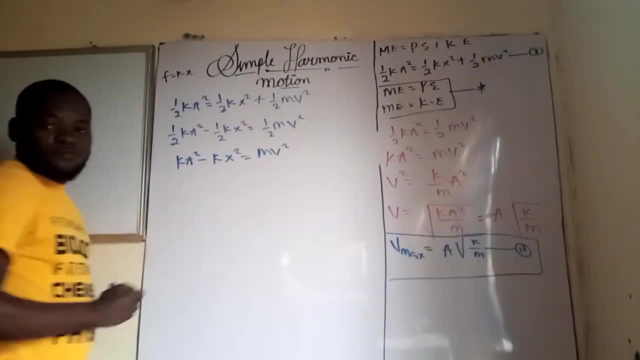 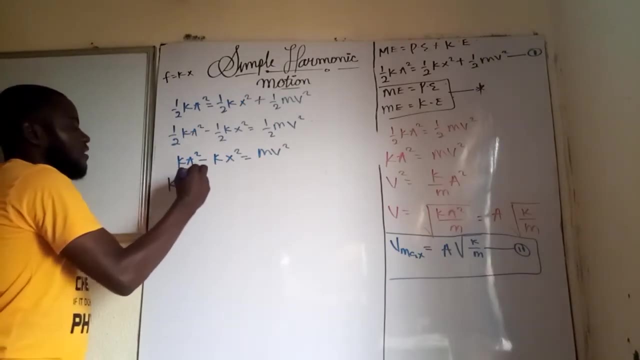 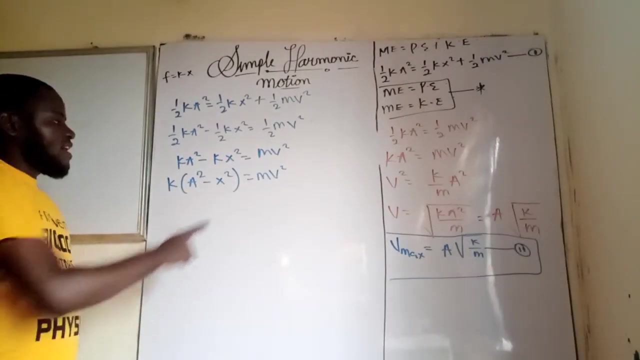 k x square equal m v square. Now, if you look at this, k is common. If I factorize it out, I have k into a square minus x square equal m v square. If this should be the case, divide both sides by m. 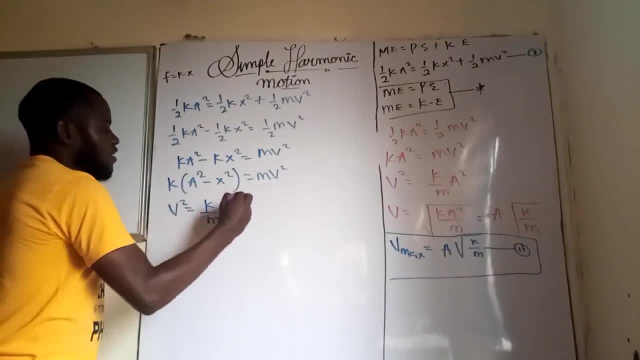 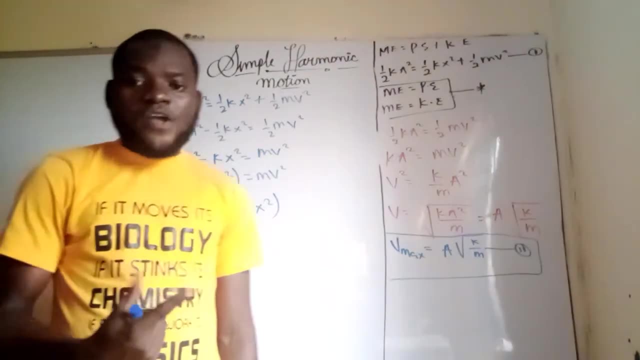 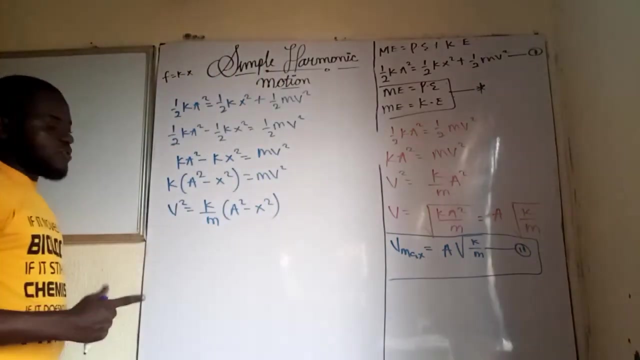 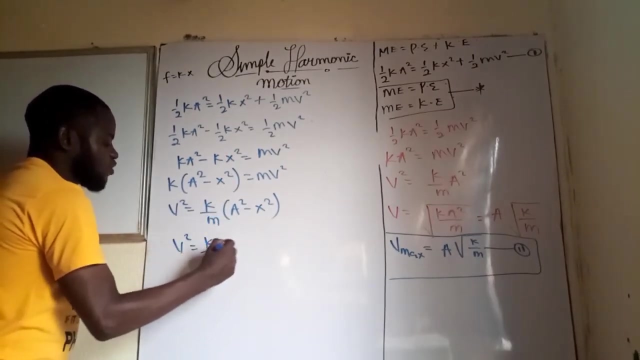 v square equal k over m into a square minus x square. Now let us try to write this equation in form of what? as a function of the maximum velocity. So if we are going to do that, let's factorize out a square. If I factorize out a square here, I will have k over m into 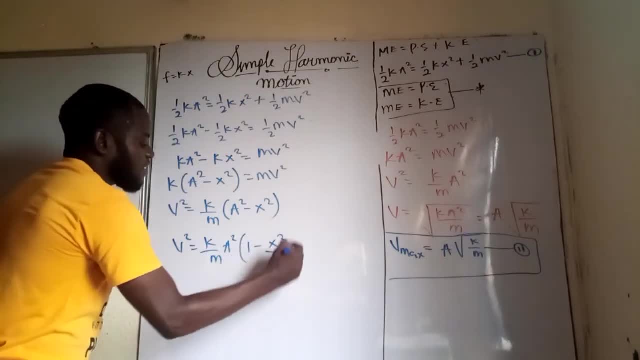 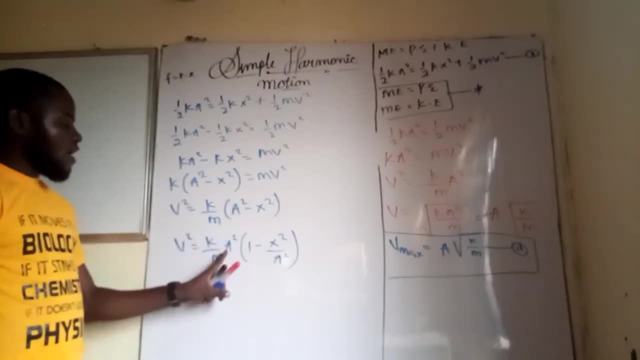 a square 1 minus x square over a square. Mathematically, if I open this bracket back with a square a square times 1, I have a square: a square times x square over a square. This a square. we cancel this, So we have. 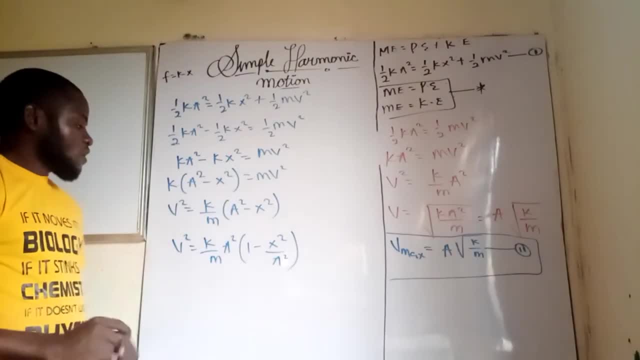 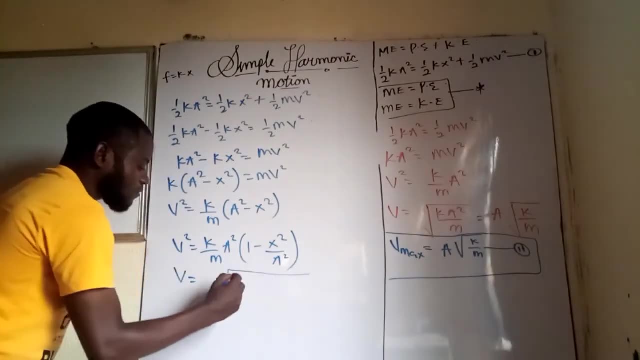 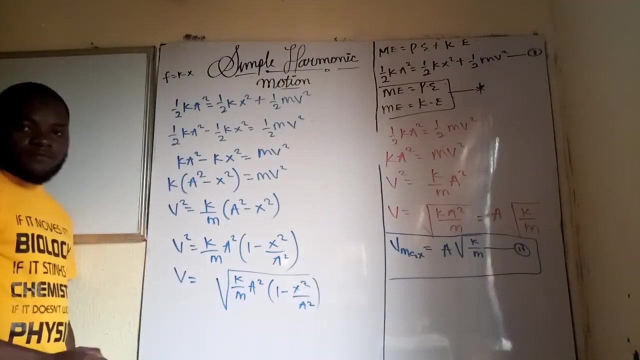 this back. So we have not done anything wrong mathematically. So if I take the square root of both sides, v will become the square root of k over m- a square into 1 minus x- square over a square. You can split what you can split this square root. If I'm going to split the square root, 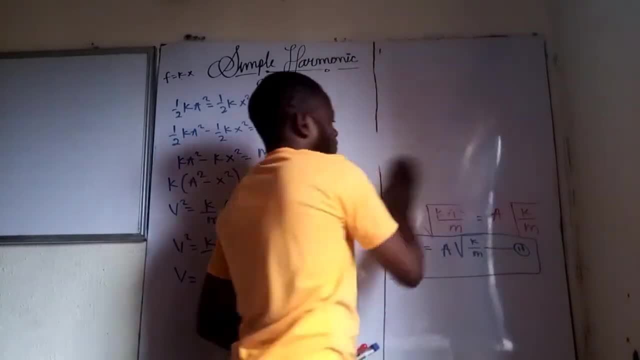 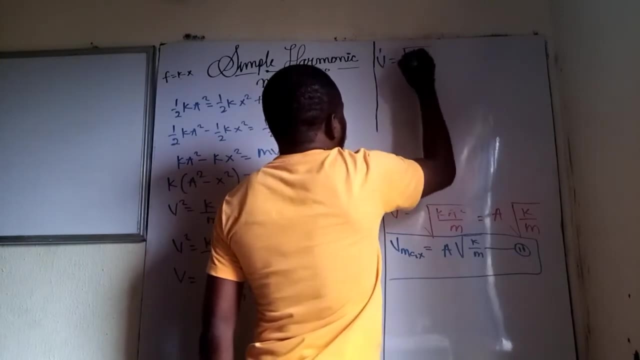 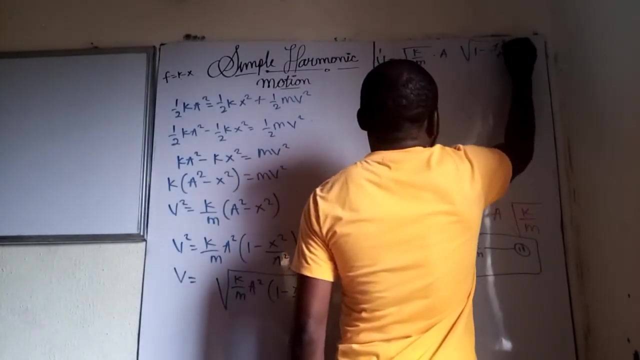 I'm going to have something like this. So I'm going to have that: v is equal to the square root of k over m times a, then the square root of 1 minus x square over a square, And if you look at this, this is the same thing as the maximum velocity. 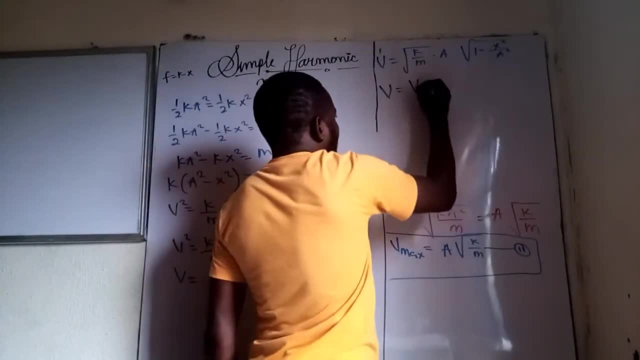 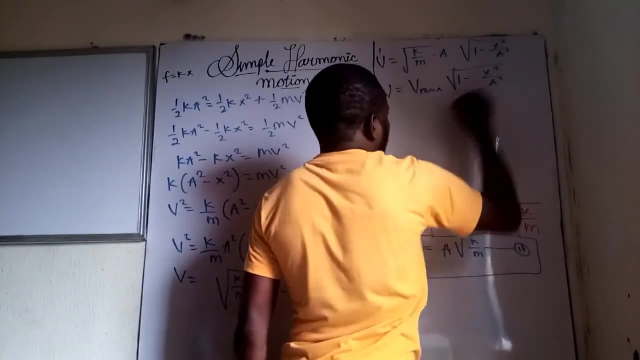 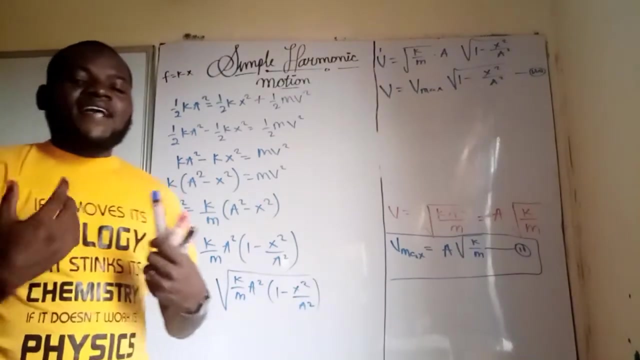 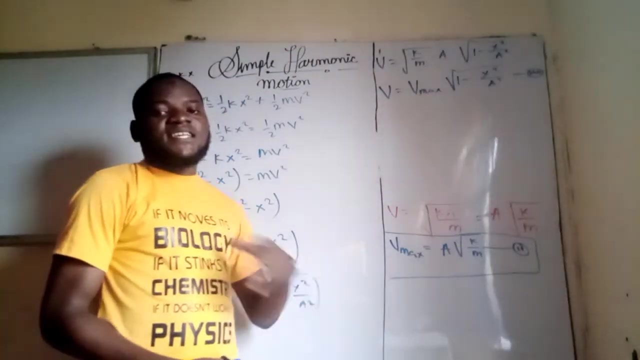 Hence the velocity at every instance is maximum velocity times the square root of 1 minus x, square over a square. And this would be our third equation. Okay, What about the acceleration of the body? We have understand how to calculate for the maximum, what Maximum velocity and velocity at every instance. 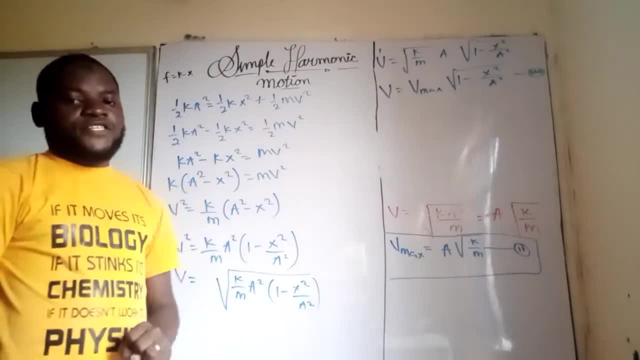 Now, how can we then calculate for the remaining velocity? How can we, by the way, calculate the velocity at every instance? What will our y? What will our y and y? What will our the acceleration to calculate? for the acceleration, we recall that the 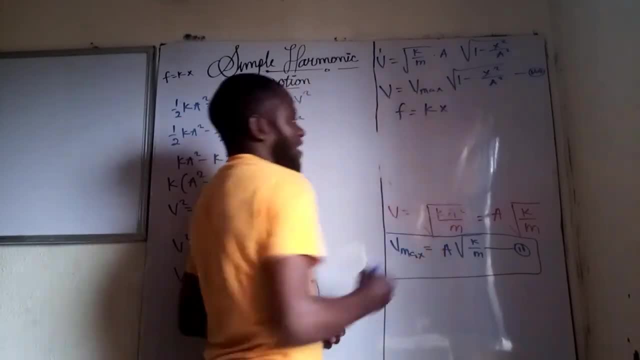 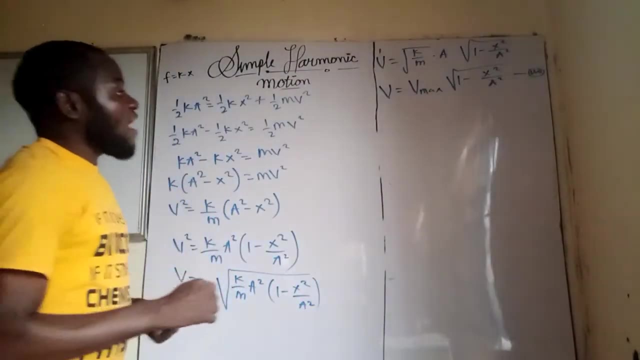 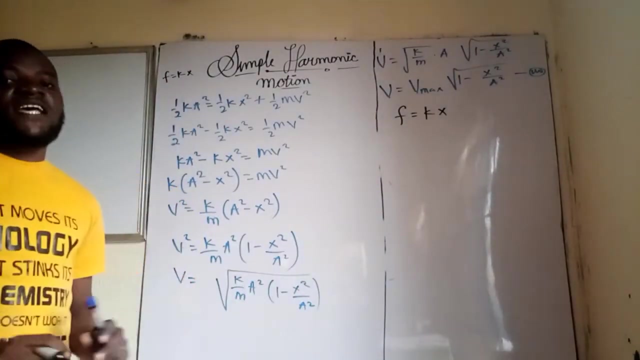 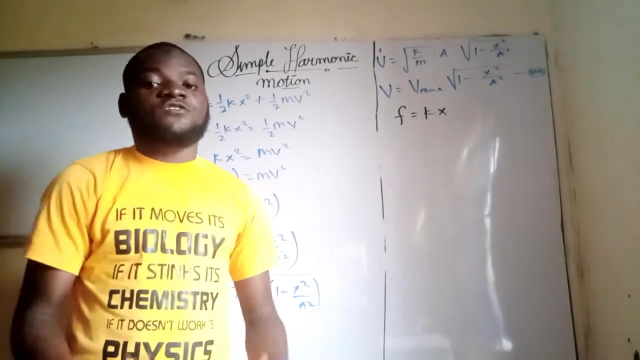 restoring force is equal to kx. okay, let me make this another color so that we can see it clearly. if I have that, restoring force F is equal to kx. let's forget about the negative sign now. so we are considering this, remember. the negative sign is just to tell you that it's moving in opposite direction to the 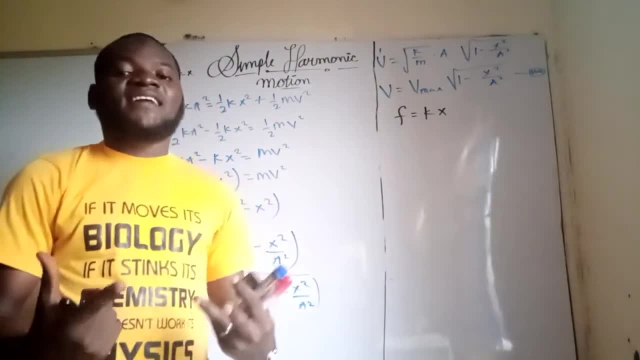 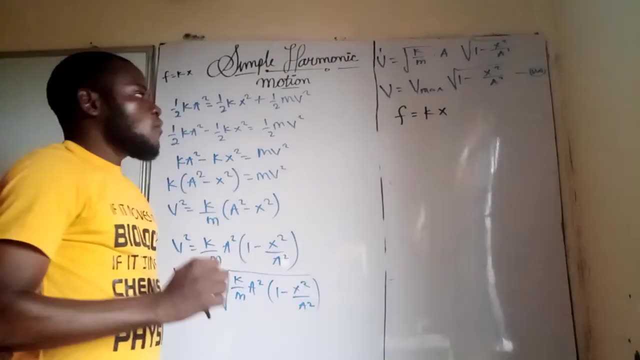 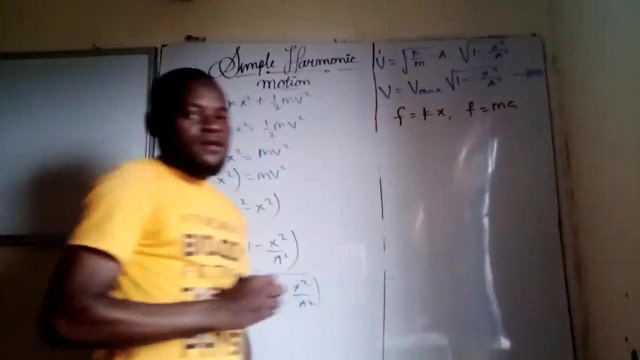 displacement vector. it's not that maybe it's affecting the magnitude, but to tell you the direction in which is facing. now, if F is equals to kx, we also have from the second law of motion that F is equal to ma. so this and this would equal to. 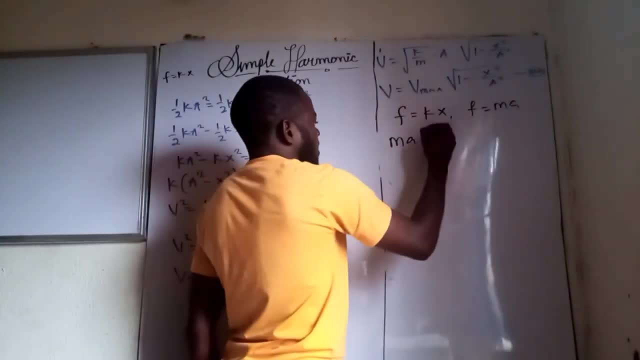 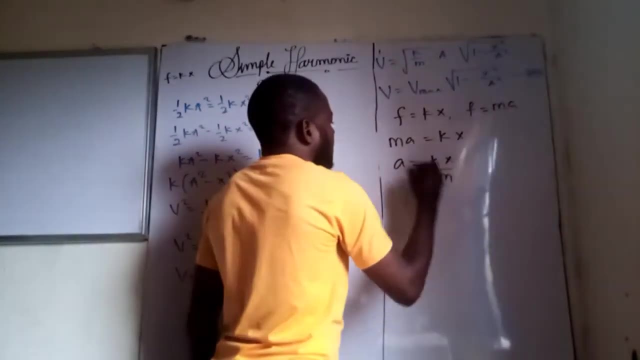 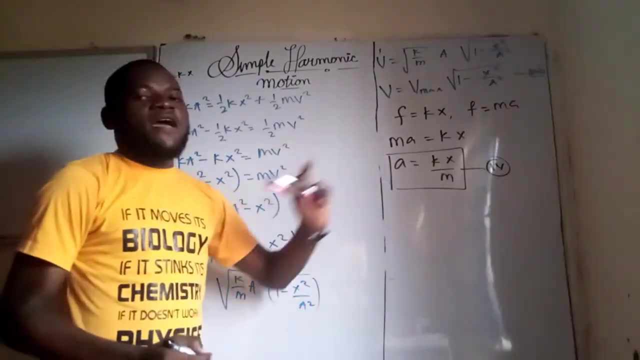 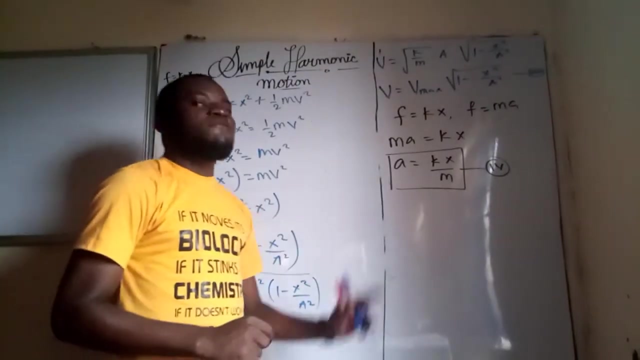 each other. I'll then add that ma is kx and a is said to be kx over M, and this would be our equation, for this is acceleration at every instance. so if you want to calculate for the acceleration of the body at every instance, we have this. but what of maximum acceleration? acceleration is. 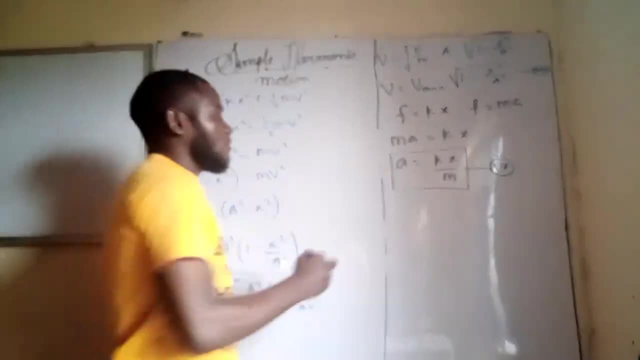 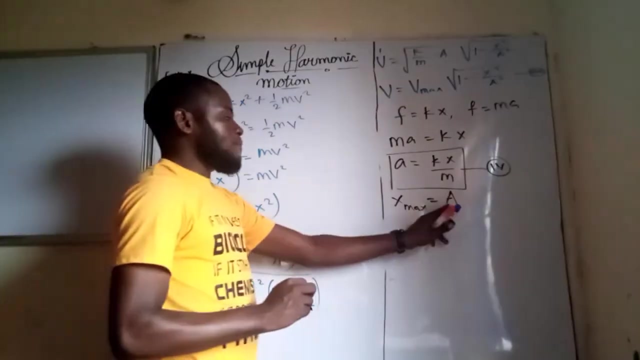 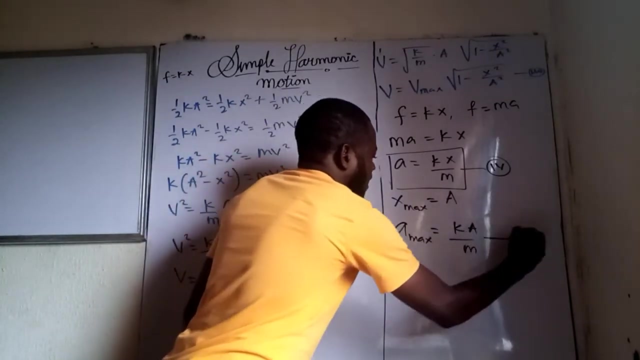 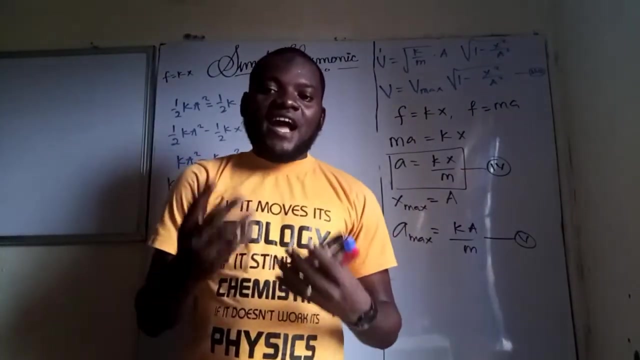 said to the maximum, when the displacement is maximum. and when the displacement is maximum is equal to the amplitude s. if I put this in place, of this maximum acceleration is k a over m, and this is equation five. now you will all agree with me that we can calculate for the velocity of the body the. 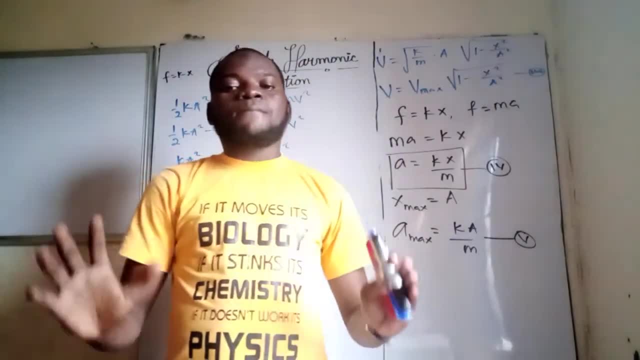 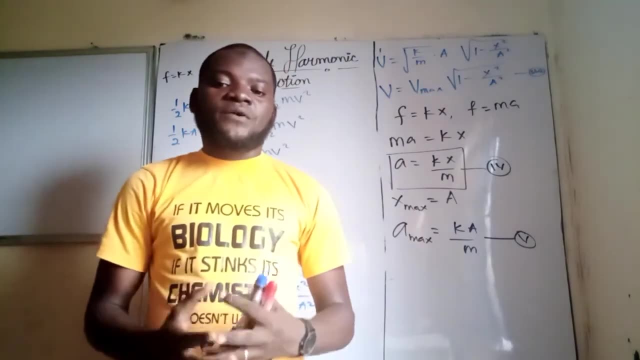 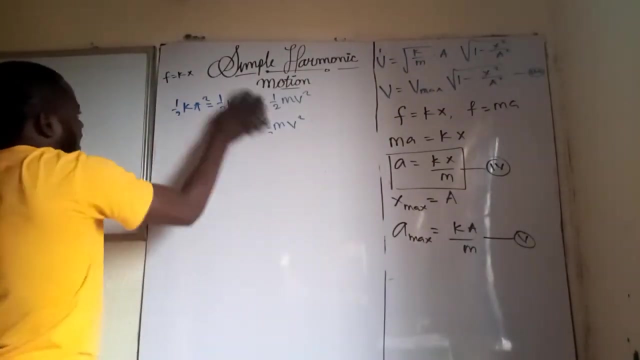 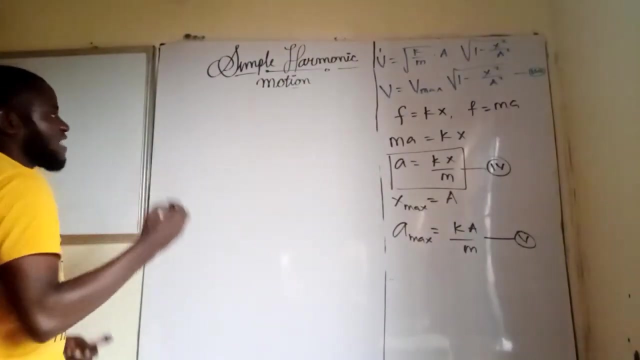 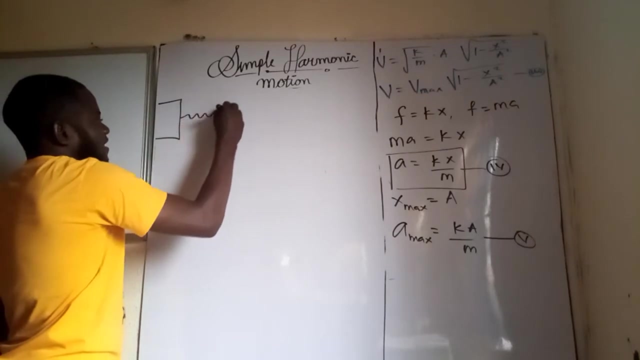 maximum velocity, acceleration at every instance. a maximum acceleration. okay, if that should be the case, let's talk about the period and frequency of this body. at this point in time, i would like to consider the string to move in horizontal for better understanding of this. let's say we have an horizontal wall and the string is like this: 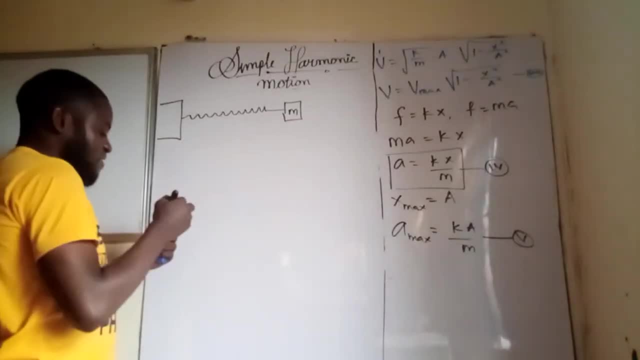 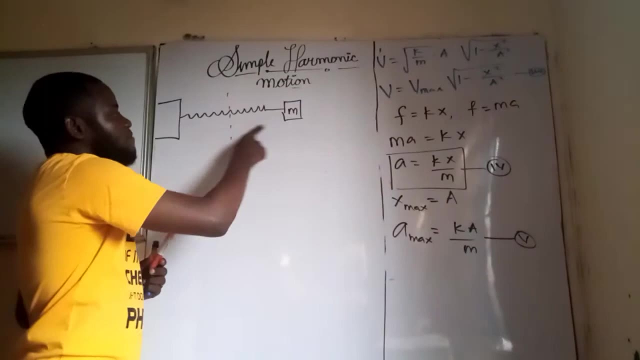 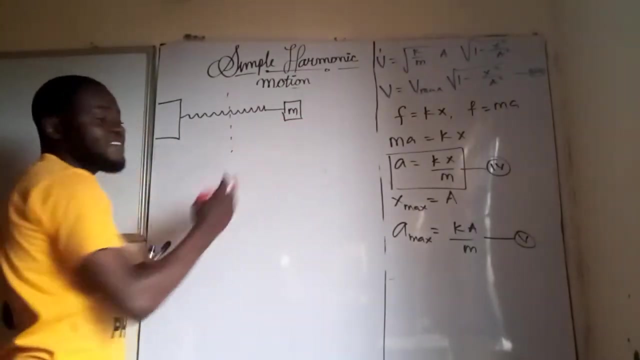 are we together? yes, now, if this is the equilibrium position of this body, by the time this body move from the equilibrium position down to this place, that is okay. let's take, for instance, now that you've released the body, the body will move from this point back to. 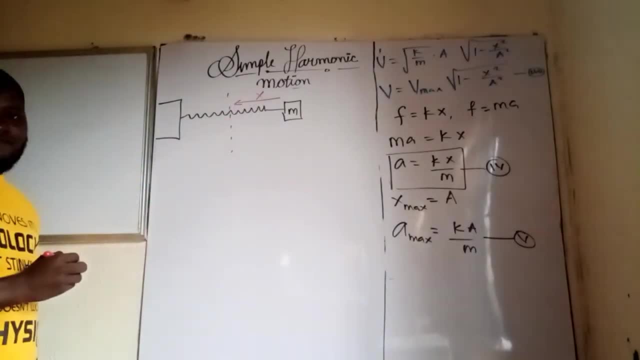 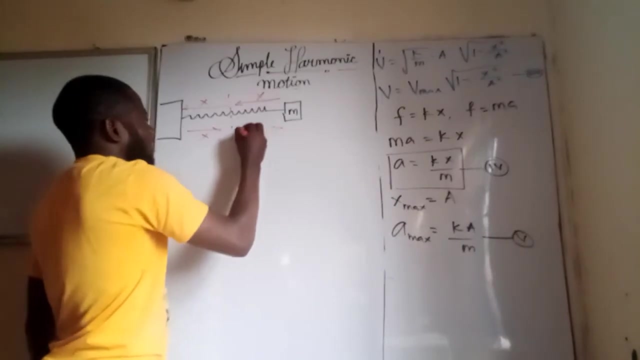 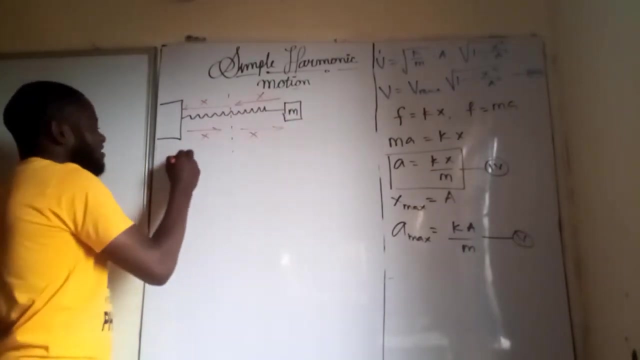 the equilibrium position. let's see, that is x. from yet of this place is going to move again. that is x, and from here it's going to move down to this place. that is another x. from here it's going to move down to this place. we have another x, hence the total distance covered by this body distance. 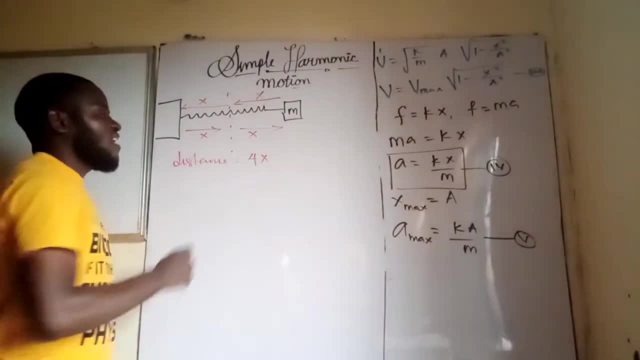 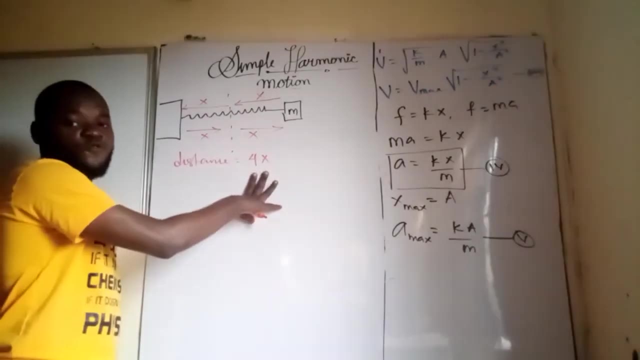 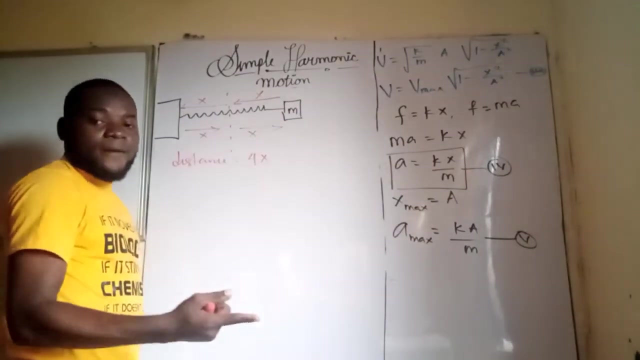 is going to be 4x. remember, a distance is a scalar quantity, so direction is not considered here. that's why this is equal to 4x. forget about the direction now. Now, if x is maximum, it's equal to the amplitude, right? 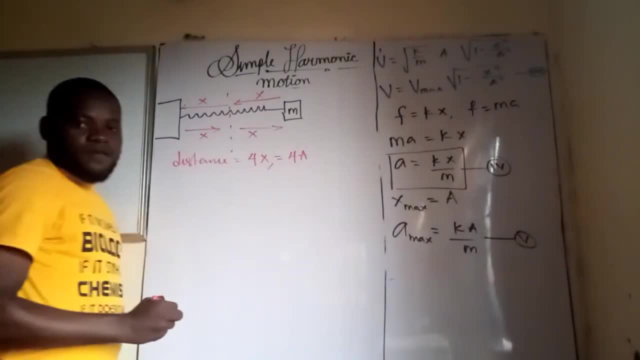 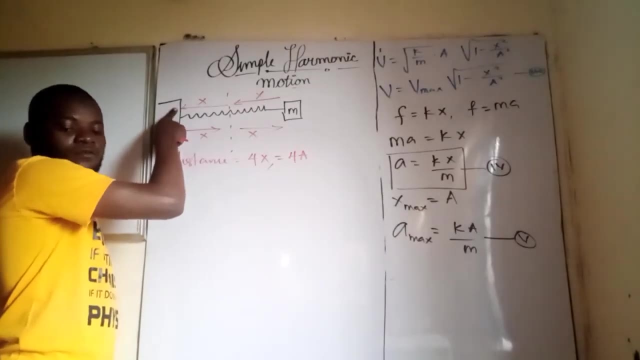 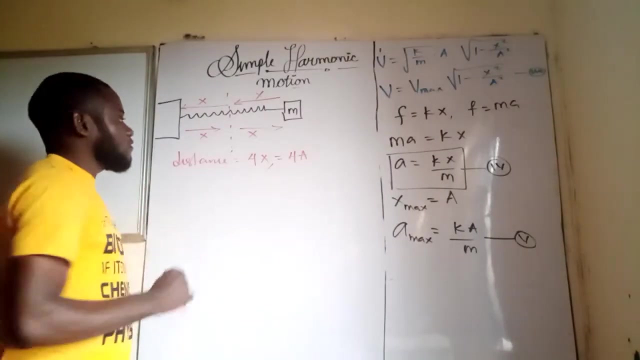 Hence distance is equal to 4a. Now, when the body moves from here down to this place, that is what Half circle. And when the body moves from here down to this place, that is another half circle. Half circle plus half circle, that gives us a complete circle. 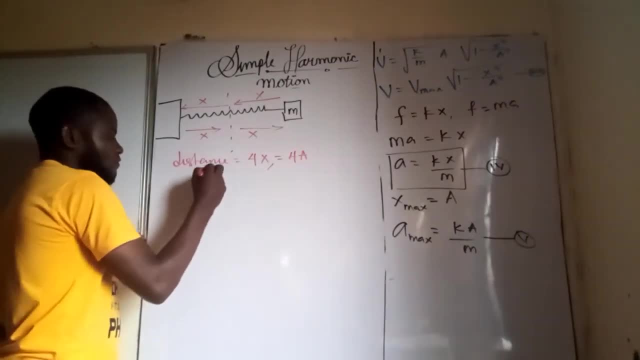 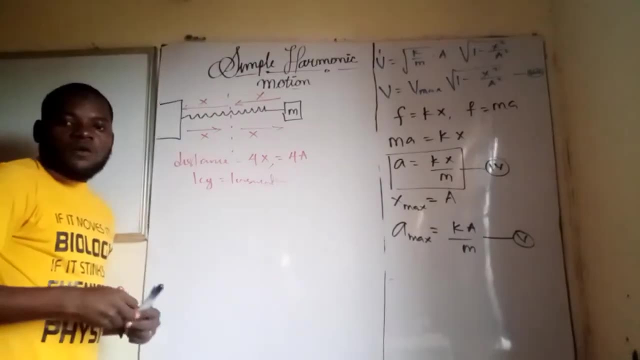 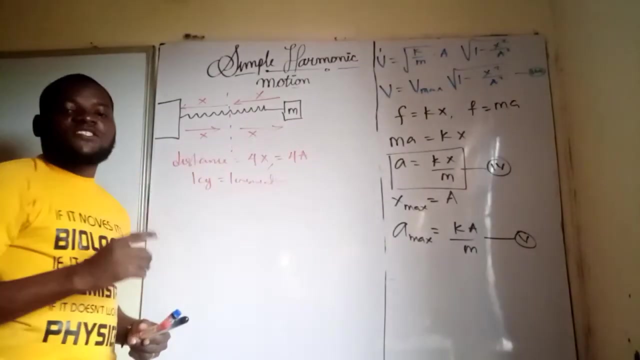 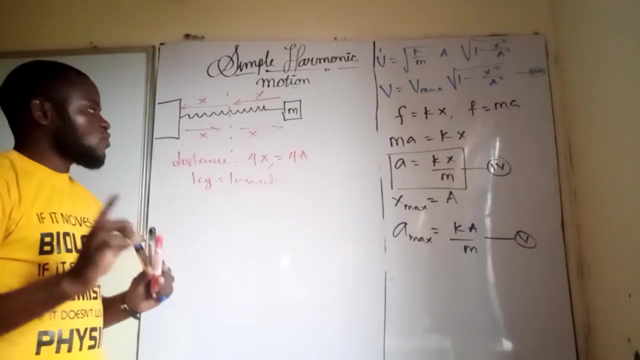 So one circle is equivalent to one oscillation. So when I say one oscillation, that is the toe and throw, When the body moves like this toe and throw, that is when the body has one oscillation. Now the body has what? 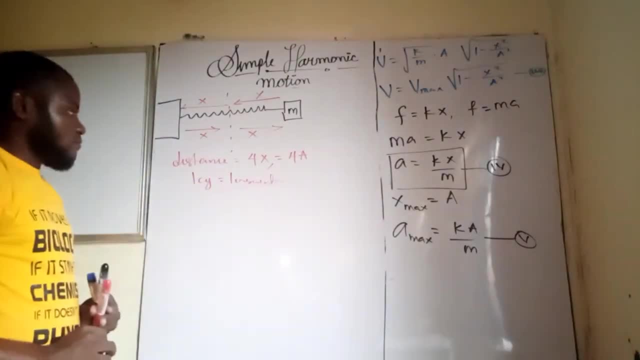 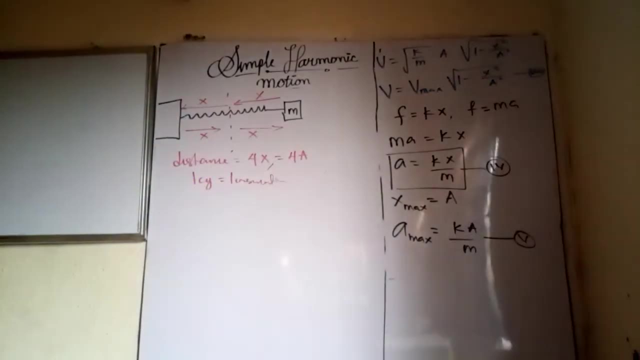 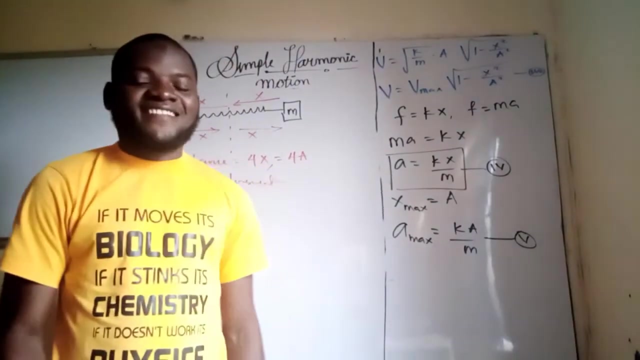 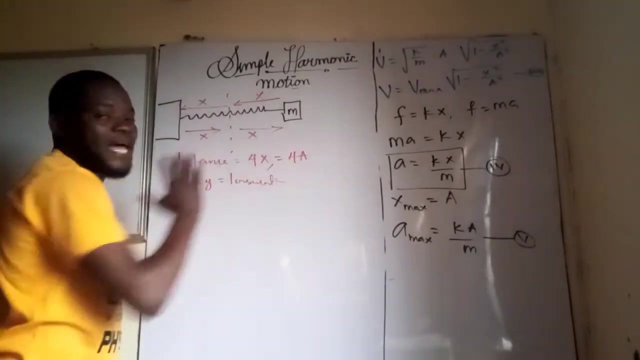 One oscillation Now. What is period and what is frequency? Be right back. Yeah, I'm back. I'm very sorry if my camera is doing that, So now let's quickly look at it continuously. Now. one circle is when this body moves toe and throw like this. 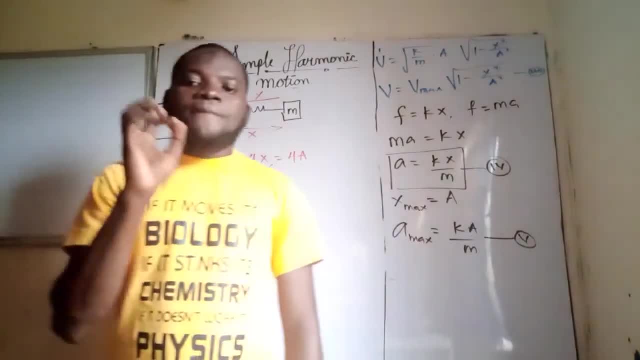 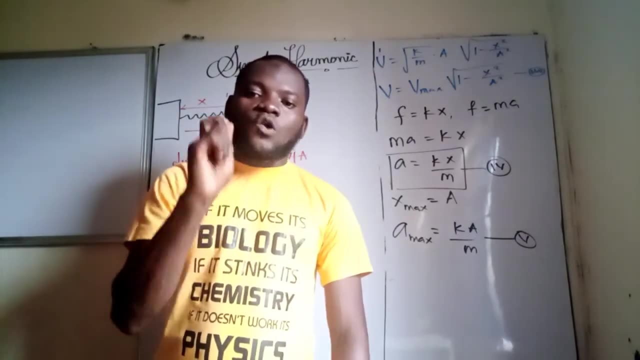 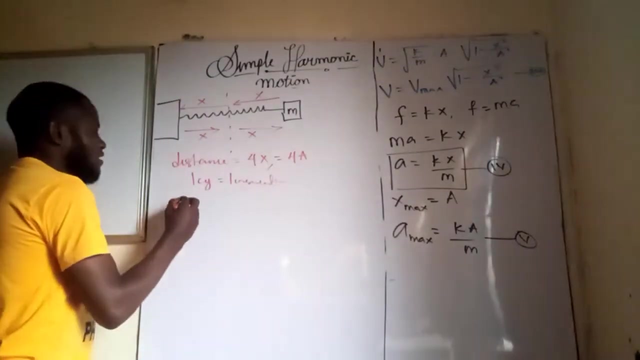 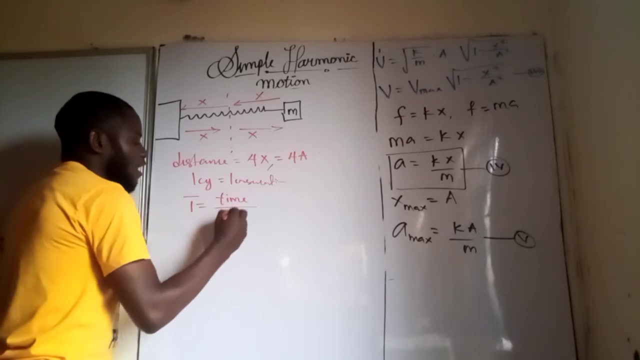 It has complete one oscillation. And what is period? A period is the time taken to complete one circle. A period is the Time taken to complete one circle. So if the time taken to complete one circle is period, Hence the period is going to be the time taken divided by the number of cycle. 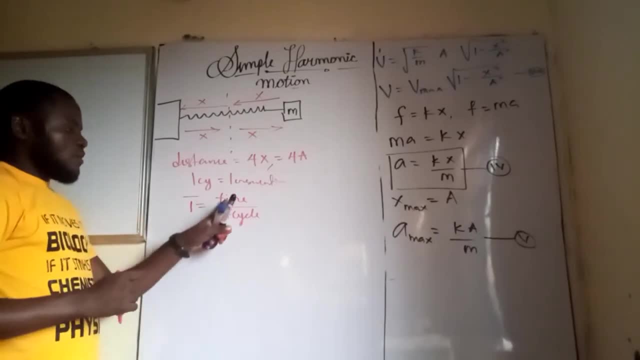 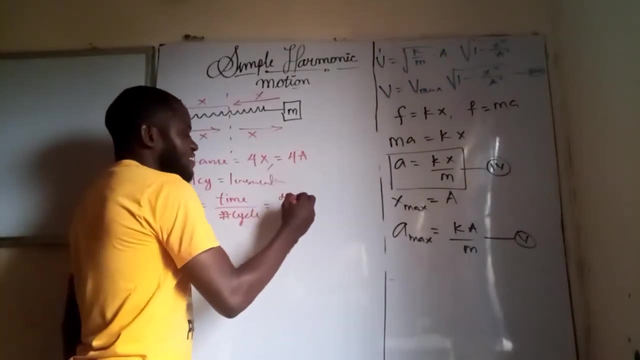 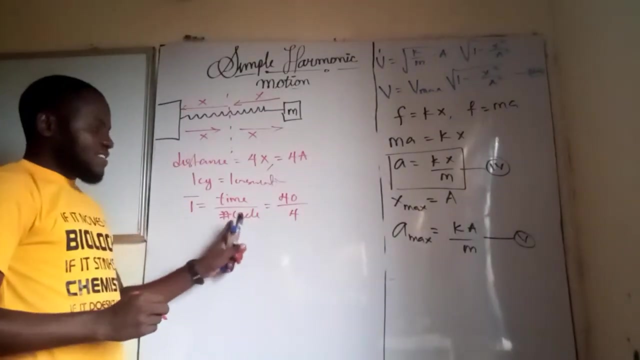 So let me put this as hash. So the time taken divided by the number of cycle will give you period. Let's take, for instance, that you have what 40 seconds For you to Count four oscillations. So if you count four cycles for 40 seconds, what is going to be the period? 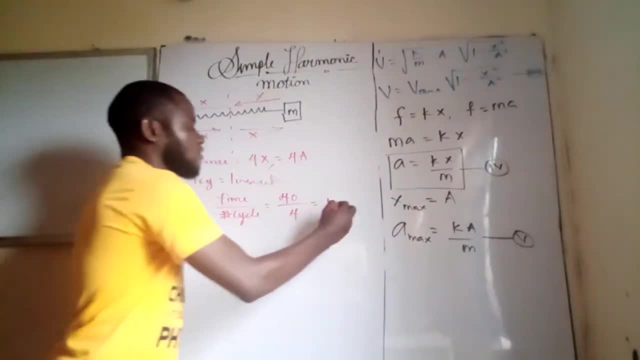 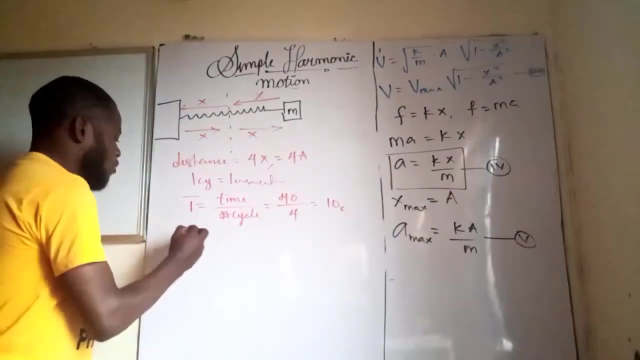 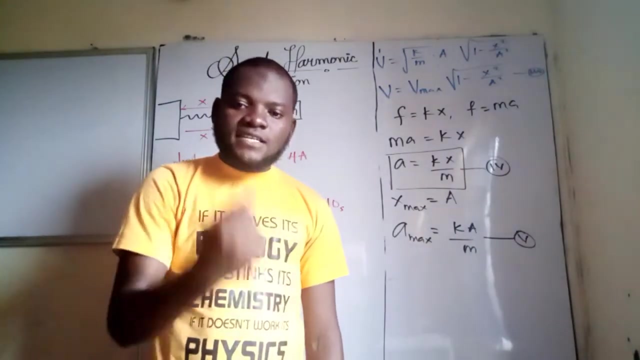 The period is going to be 10 seconds. It means it takes 10 seconds to count one cycle. Now, what is now going to be the frequency? Frequency is the number of cycles per seconds. The number of oscillations per seconds is frequency. 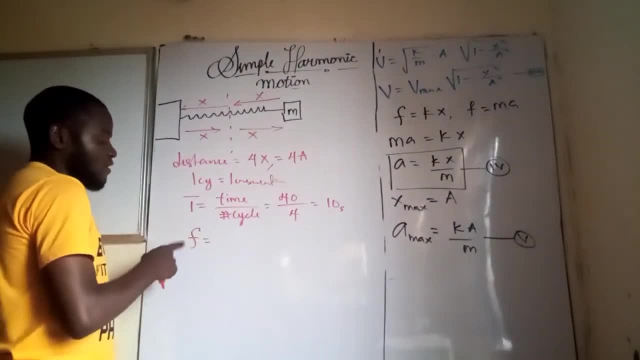 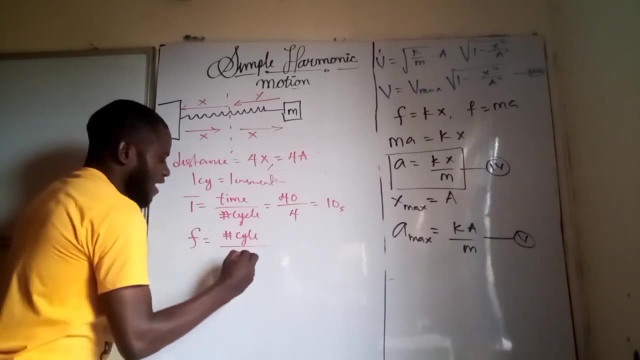 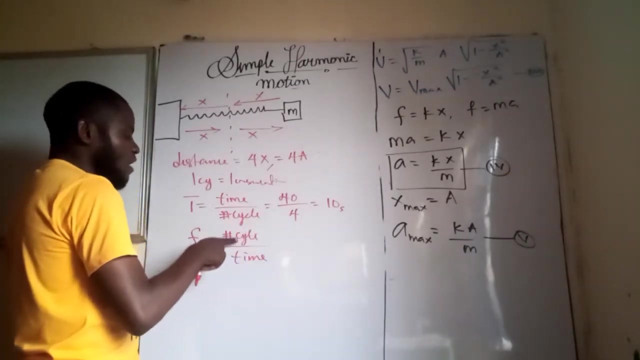 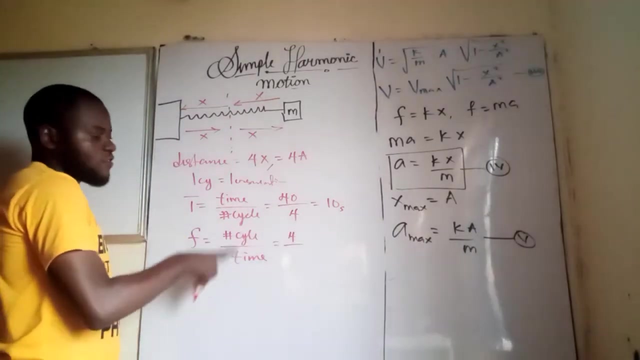 Hence, if I have frequency, frequency is going to be the number of cycles divided by the time taken. Hence, if I have this particular body, now, if the number of cycles is four and the time taken to count four is 40,. 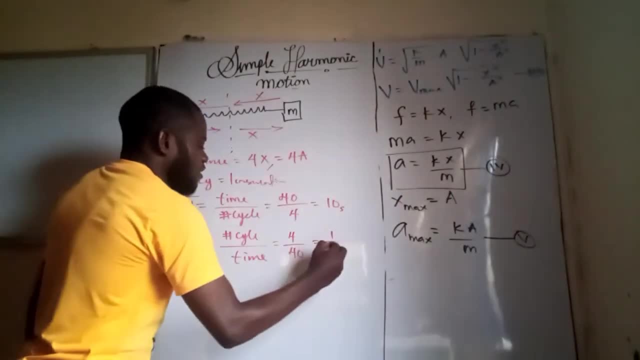 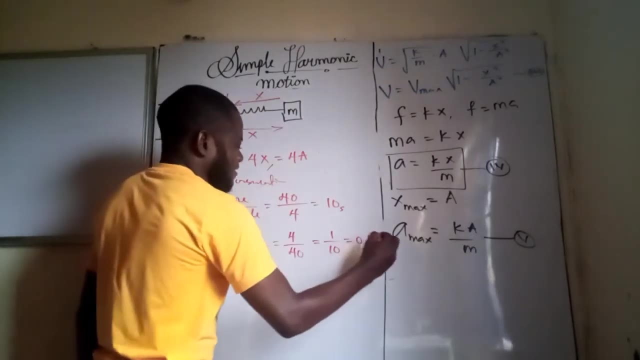 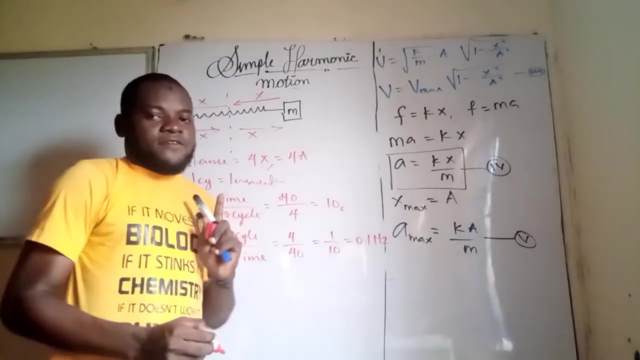 then our frequency is going to be 1 over 10.. Hence this is 0.1 hertz. It means for every seconds, you complete 0.1 second. I believe we understand that. Now. this is just this. 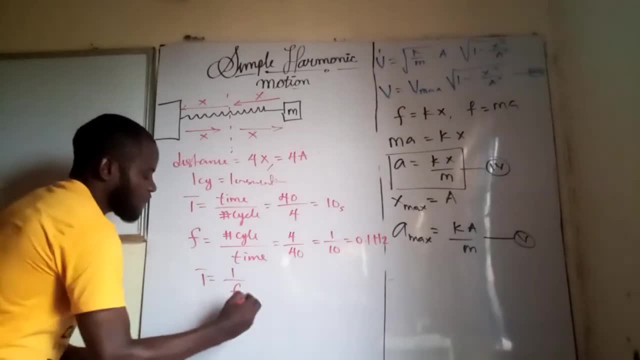 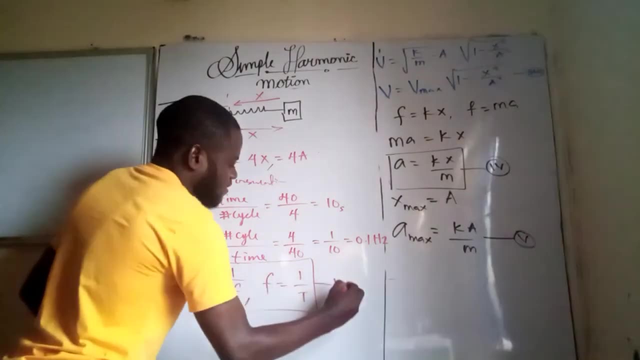 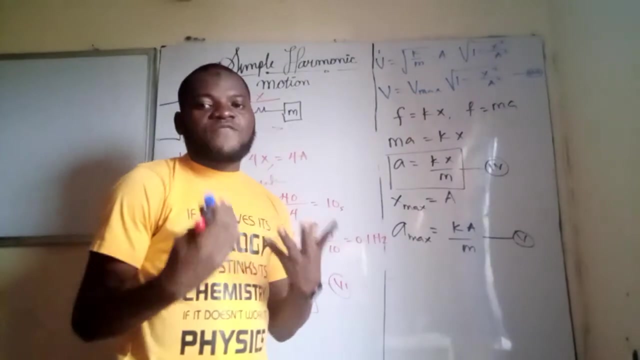 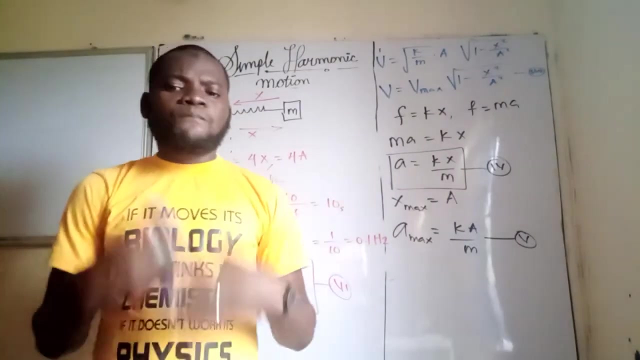 It shows that period is 1 over frequency and frequency is 1 over period, So let's call this equation 6.. Okay, Since we have been talking about acceleration and velocity in terms of what spring constant and the mass, Now let us also talk about what period and frequency 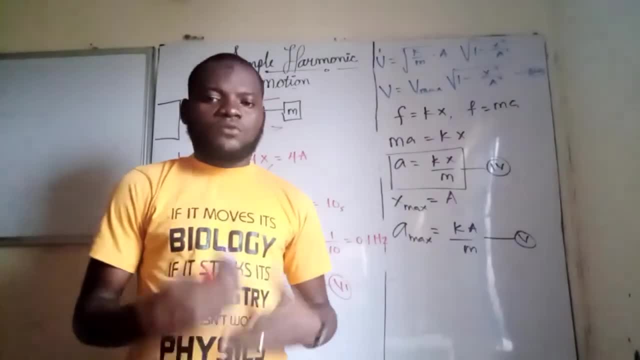 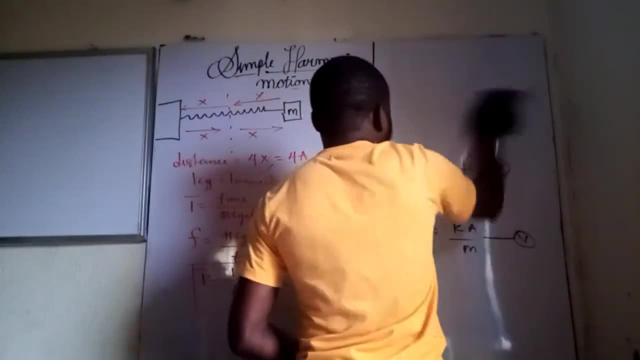 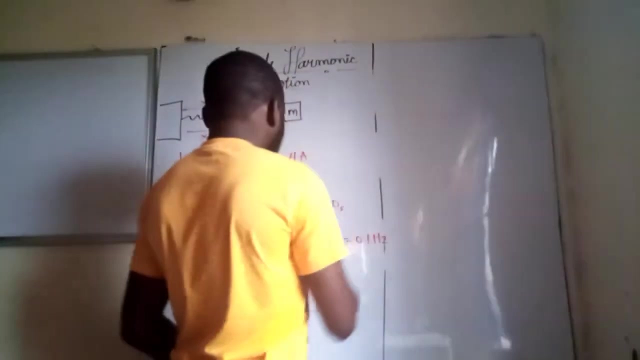 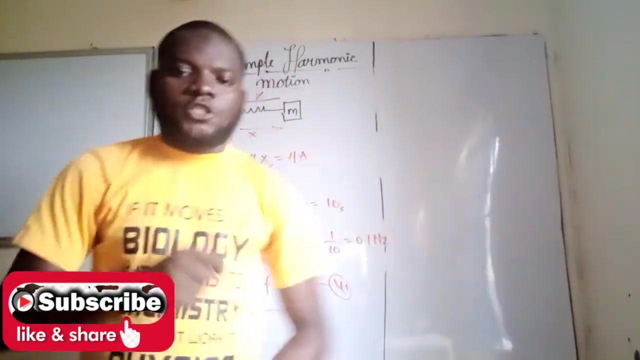 in terms of what the spring constant and also the mass of the body Pay attention class. Okay, if you are with me, I would like us to go into that. Let's consider a body that is performing a circular motion, like my wristwatch. 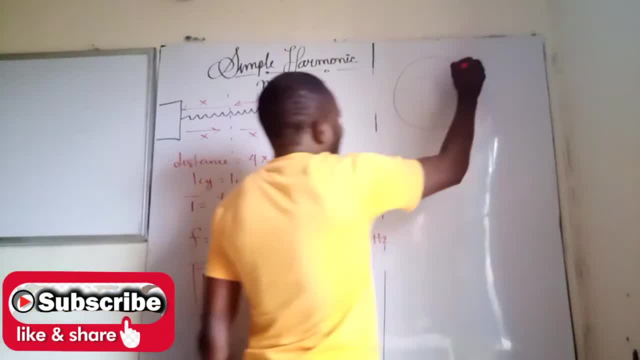 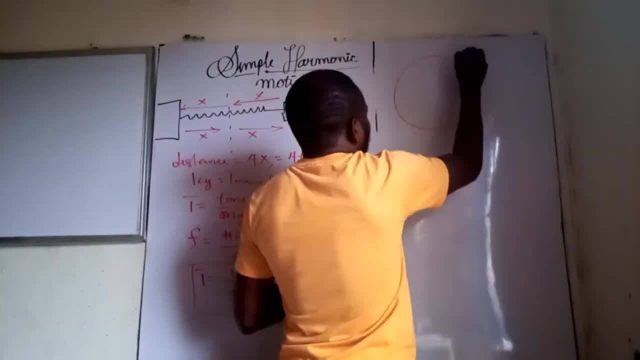 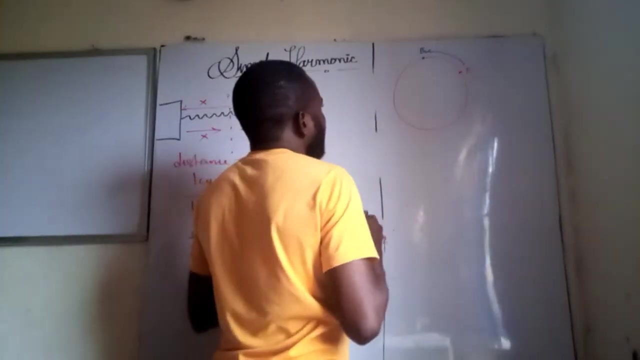 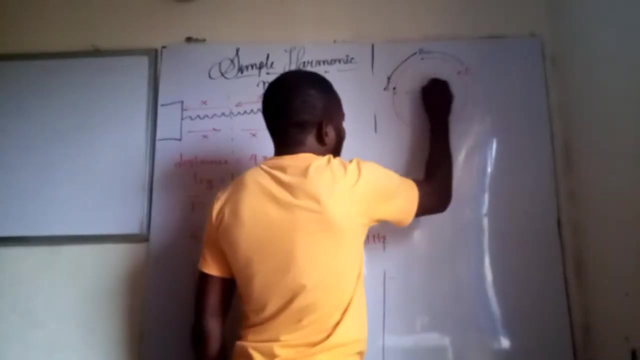 If you look at my wristwatch, if it starts to move from here, let me say this is point A and the wristwatch moves to another point B and it moves from another point B down to another point C. If you look at this, let's say this is the diameter. 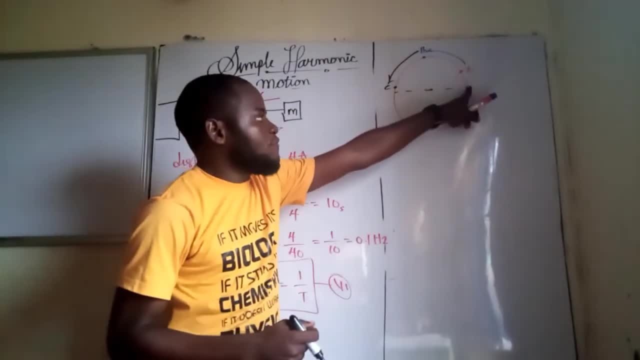 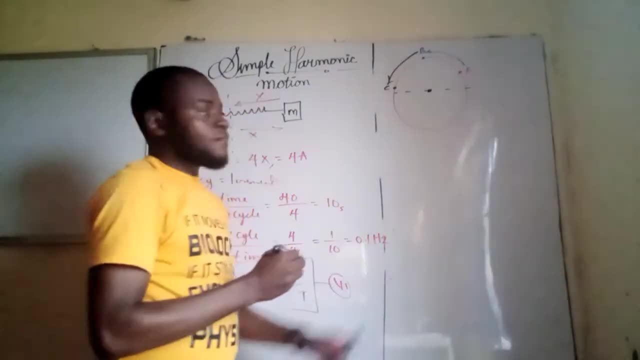 If you look at it now, it will look like this body is moving towards the negative axis of X, because if this is the center of this circle, here is going to be positive X and here is going to be negative X. So if you look, 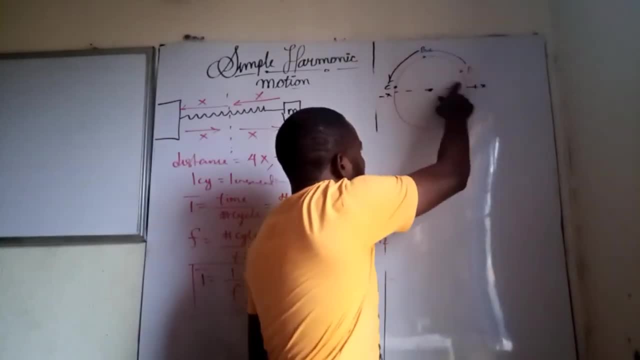 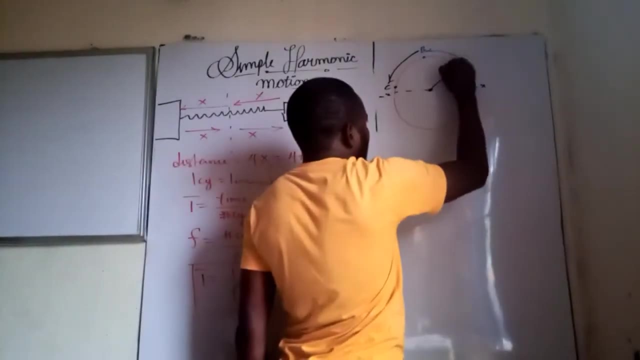 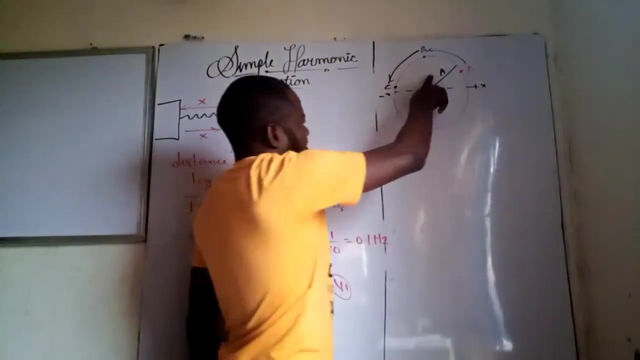 If you look at the circle horizontally, it looks like the body is moving in the X plane A bit. Yes, This will be the maximum displacement of the body, which we call the amplitude. Okay, If this is the amplitude, here is our X and here is angle theta. 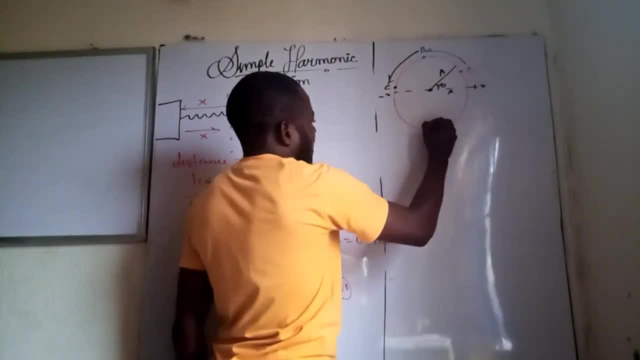 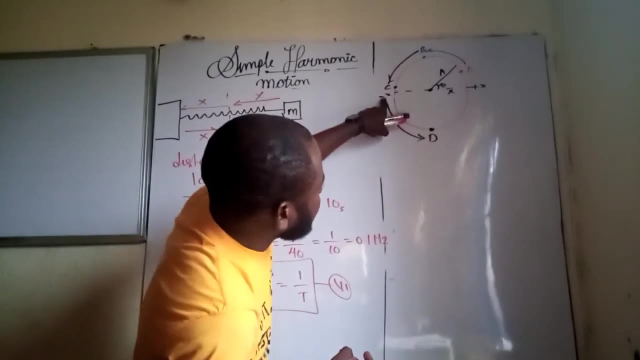 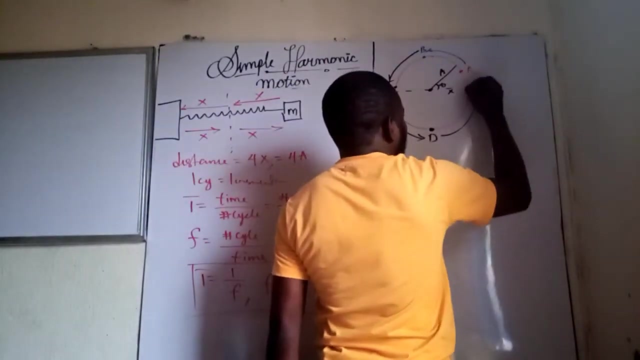 By the time this body moves to this place it's going to move down to another point D here And by that time you will see that the body has started moving from the negative axis going towards the positive axis. By the time it gets to this place also, it returns back to A. 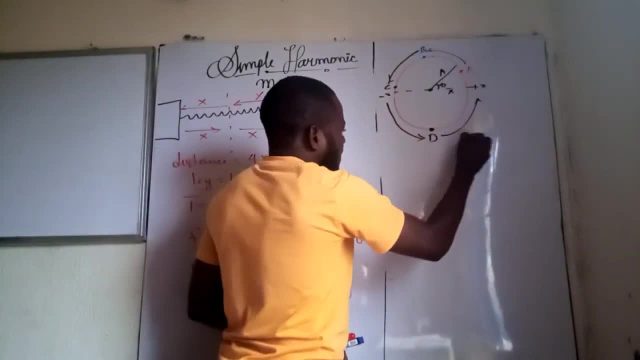 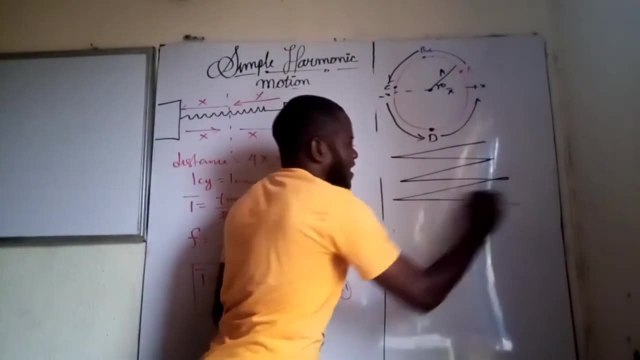 You see? So it shows that the body is moving like this and like this, So this motion will continue back and forth, back and forth, and that's why we said the second hand of this wristwatch is also a simple, harmonic motion. 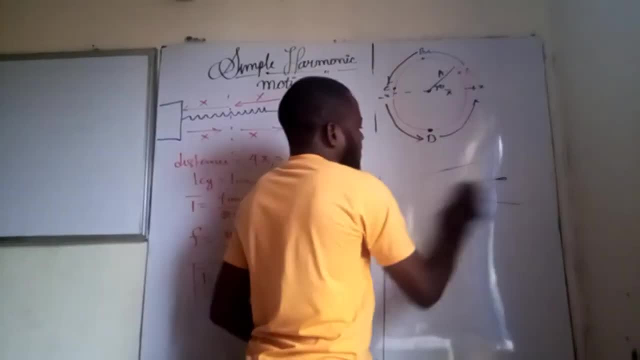 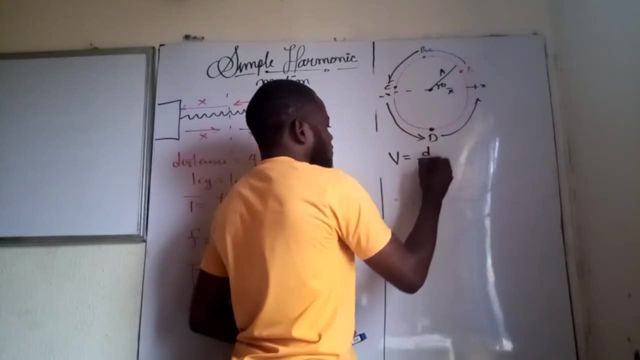 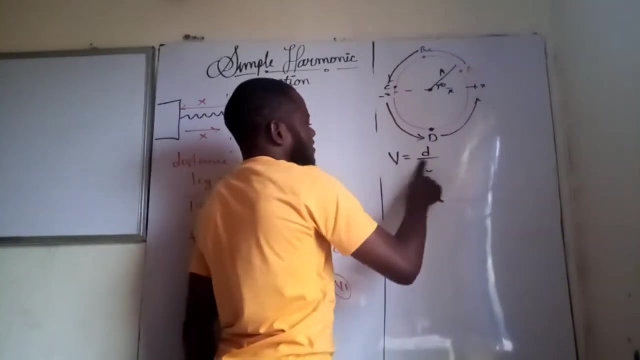 Now, if this body is performing a simple harmonic motion, like we just explained, now we are going to have that the velocity is displacement divided by the time, And the time that will take this body to move from here and come back to this place is known as the period of oscillation. 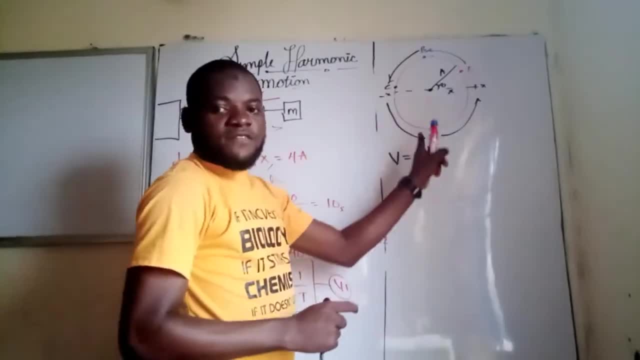 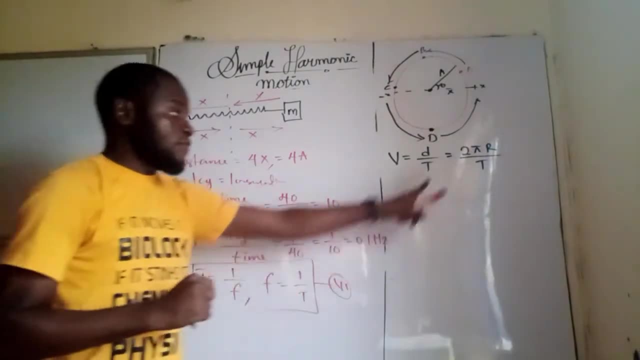 Now, the total distance covered is the circumference of this circle, And the circumference of a circle is 2 pi R or minus. The circumference of a circle is 2 pi R, so the velocity will be 2 pi R divided by T. 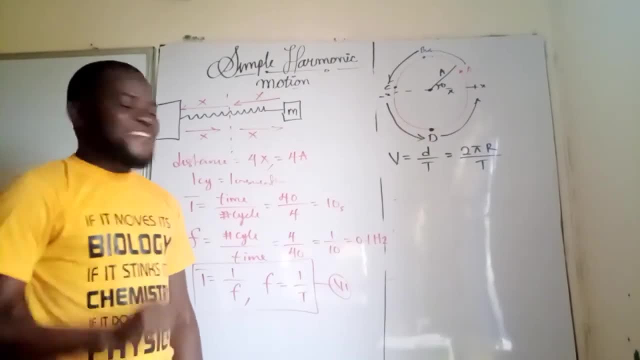 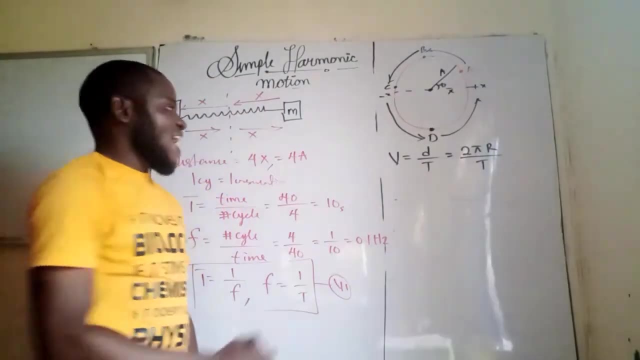 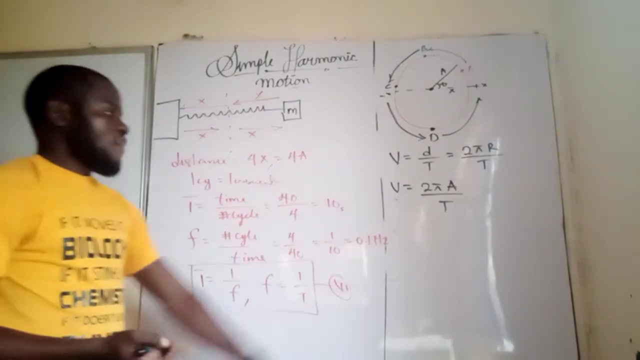 Abhi, Yes, Yes, Okay, If that should be the case, our R is radius. Looking at this diagram, our radius is our amplitude. Hence V is 2 pi A over T. So if I make T the similar formula: 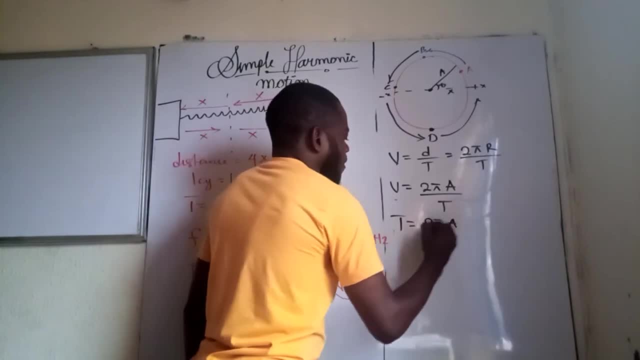 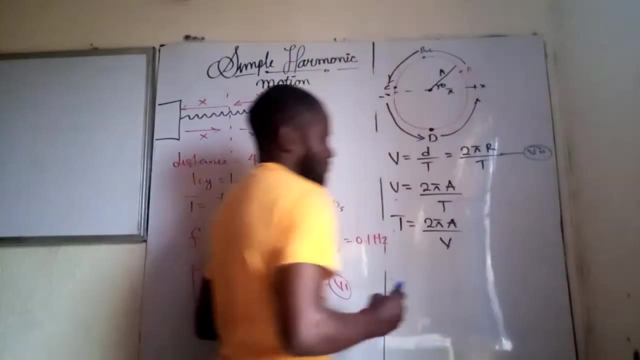 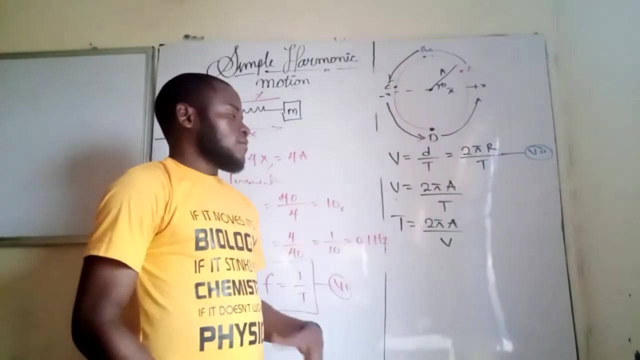 I will have that T is 2, pi, A All over V. So let's call this equation equation 7.. Now I know that velocity is expressed in terms of amplitude, So let us go back to the formula for maximum velocity. 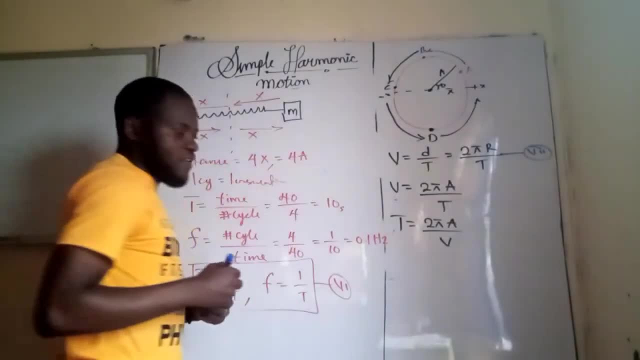 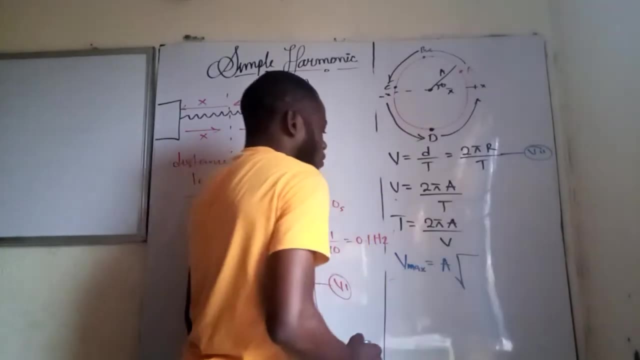 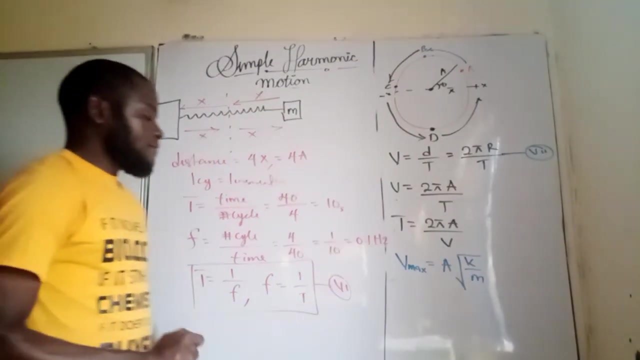 We have that. our maximum velocity, if you can recall vividly, our maximum velocity is A times the square root, which is the square root of K over M. Can you recall? Okay, If this should be the case, let's make what. 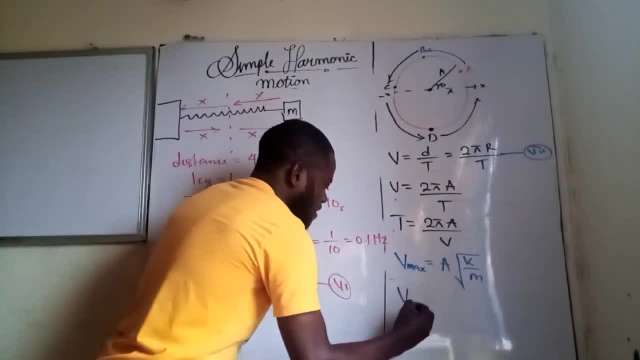 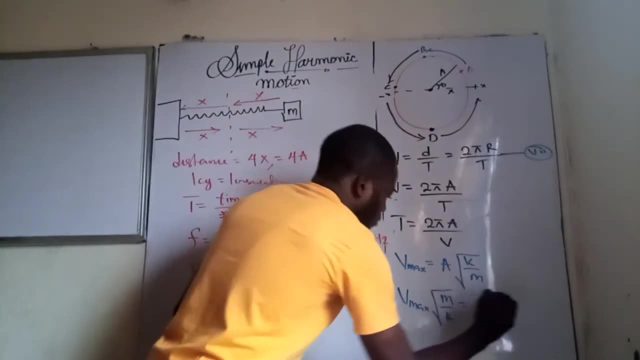 A the subject of the formula. If I do so, I will have that V max is the square root of M over K, and that equals to what A? That is, I multiply both sides by the reciprocal of A. So that is, I multiply both sides by the reciprocal of A. 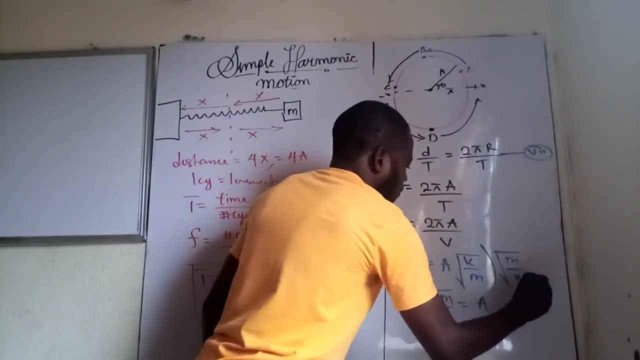 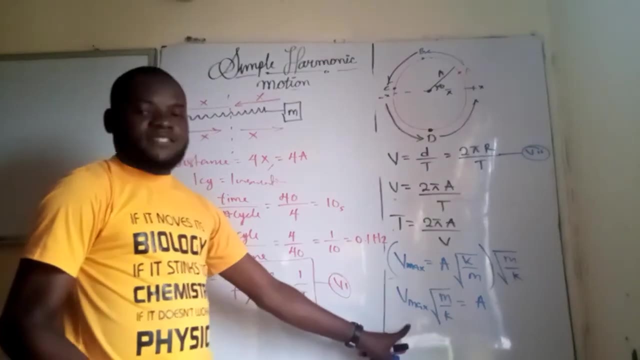 That is, I multiply both sides by the reciprocal of A, So you get the reciprocal of this, which is M over K. You know, this and this would cancel, and this and this would cancel. Why this? We multiply this. 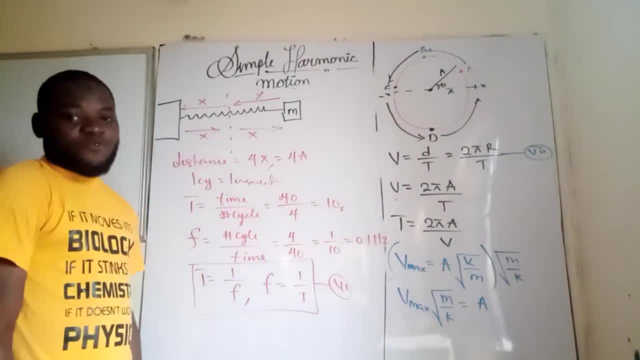 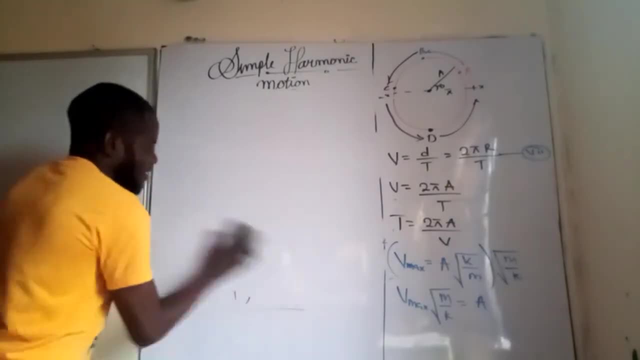 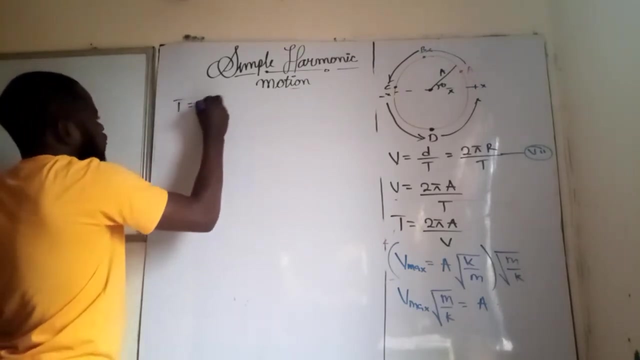 Okay, I believe you are getting what we call a symphonic motion right now. Okay, If that should be the case, let's quickly slot this into this equation. So I have that the period is going to be 2 pi, so this is gonna be equal to given. 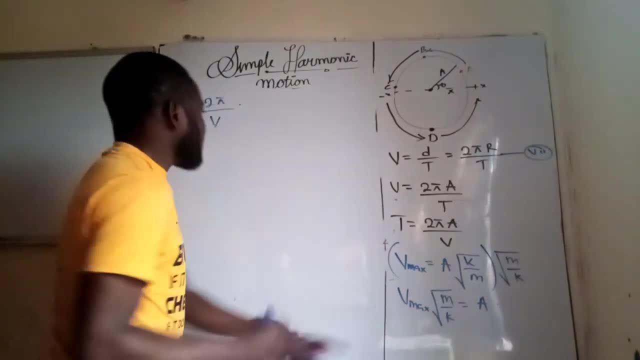 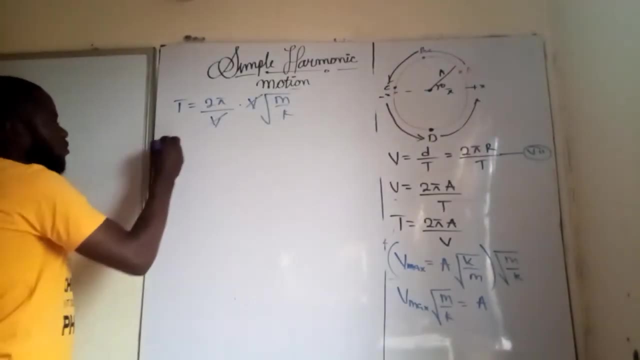 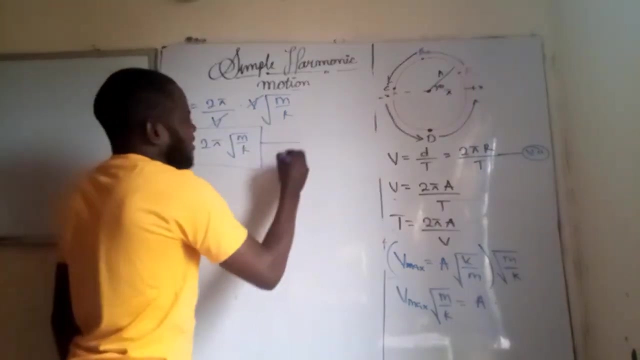 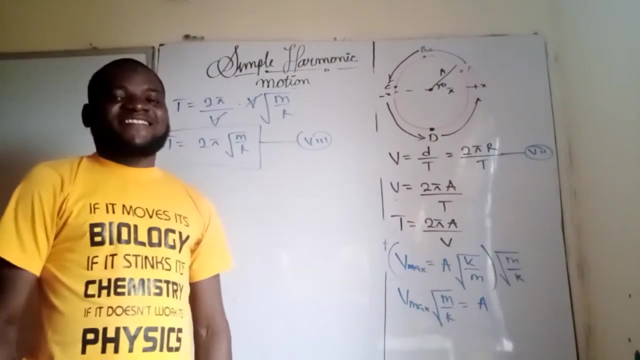 that divided by v times a, is now going to be v, the square root of m over k. v and v will cancel, so the period is going to be two, pi, the square root of m over k. so let's call this equation eight. okay, guys, you i'm happy teaching physics and i know you happy learning physics as well. 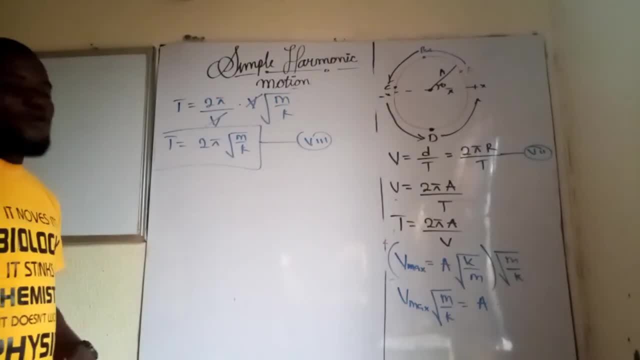 if that should be the case, let's move on from here. but before i go on, i would like to explain how this will affect the period. when the mass of a substance is very high, the period is said to be high as well. that is, if the k is small, the period is said to be high, and if k is high, the period is. 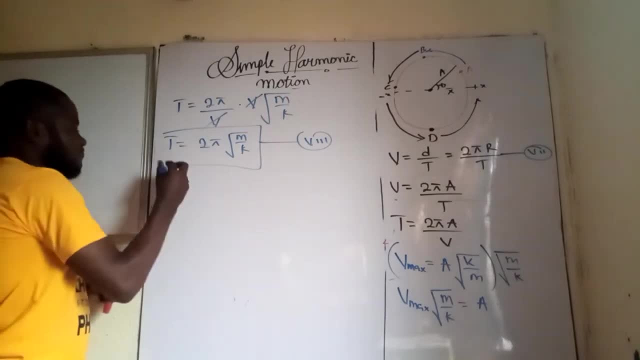 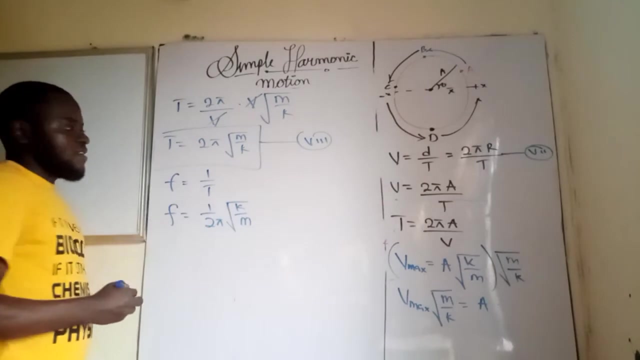 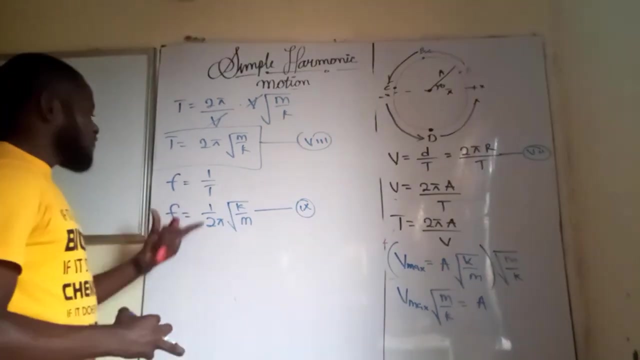 said to be small. okay, now we have that. frequency is one over period. so frequency in terms of this, we are going to have that f is one over two pi, the square root of k over m. so this would be equation nine. so we have expressed what frequency in terms of the spring. 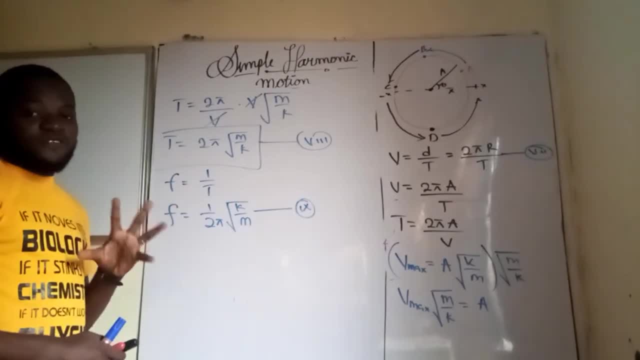 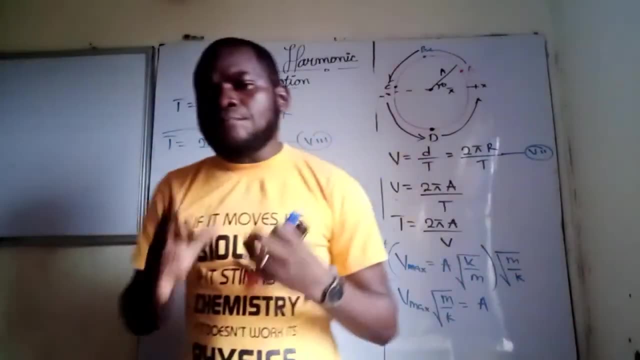 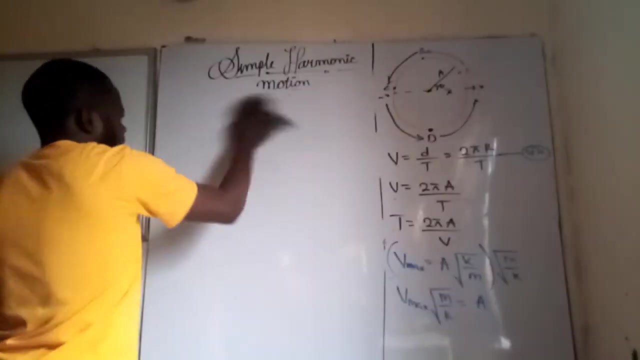 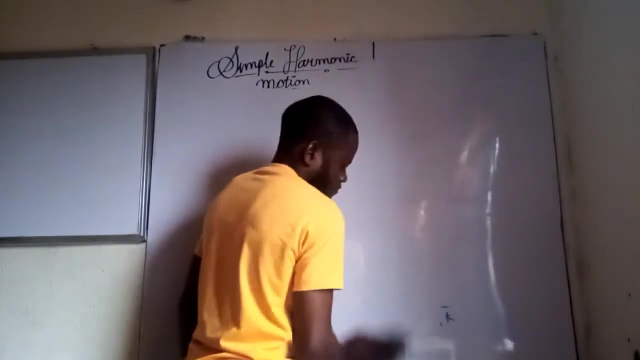 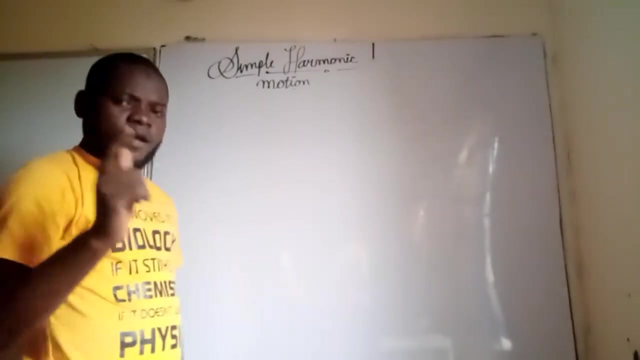 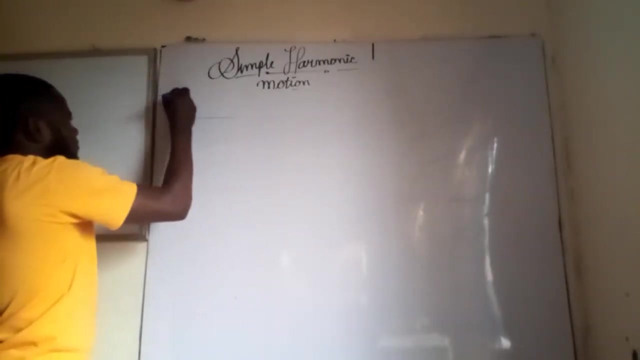 constant and the mass, likewise the period in terms of the spring constant and the mass. now let's see. what again do we need to understand about the simple harmonic motion of the spring? now let's look at something you welcome back now, if you look at this, if i have that, the string is oscillating within. 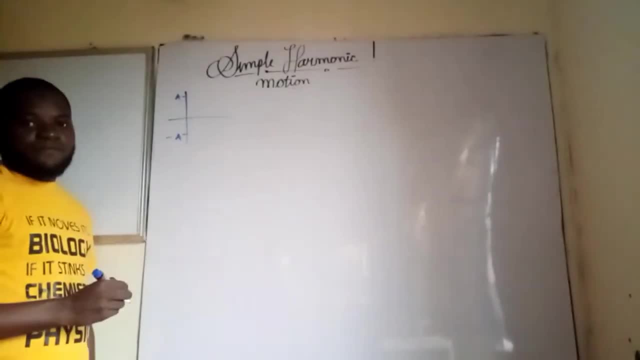 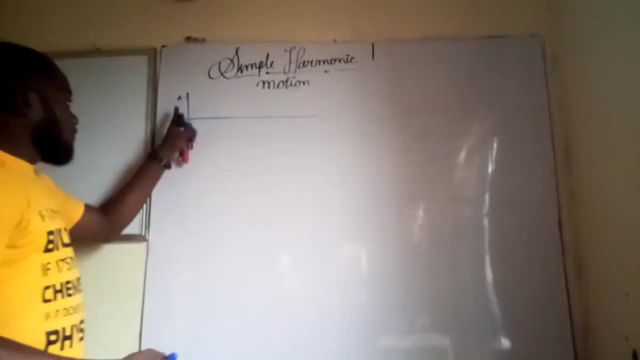 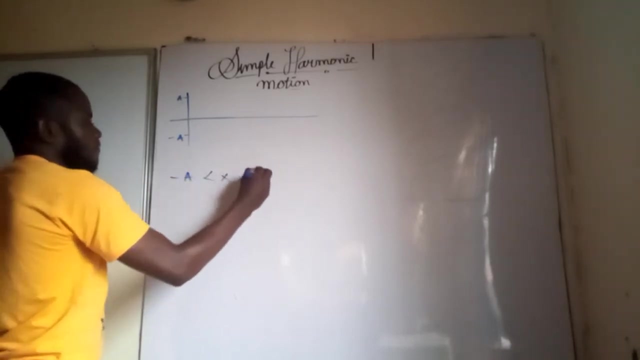 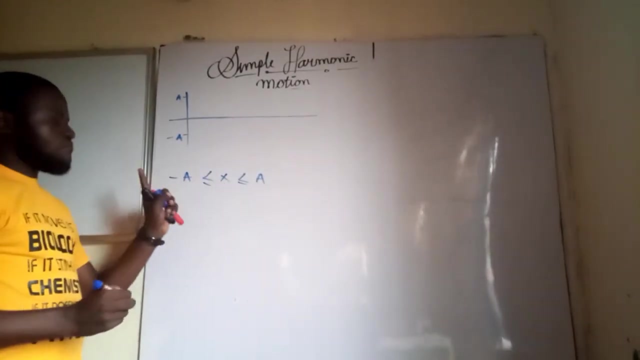 this point and this point. so if i plot the graph of the displacement, you know the maximum displacement of this motion that we are talking about, since is the amplitude, and the minimum displacement will also be negative amplitude, in other words, the value of x. the value of x range between 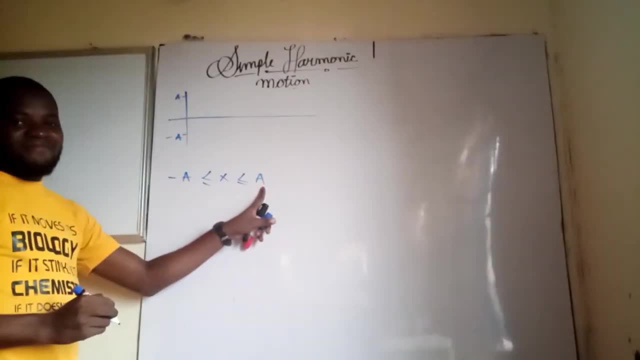 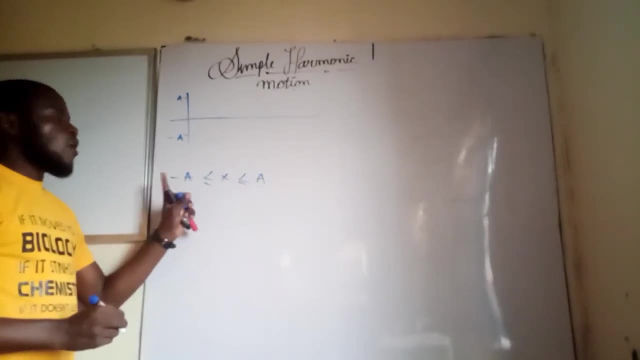 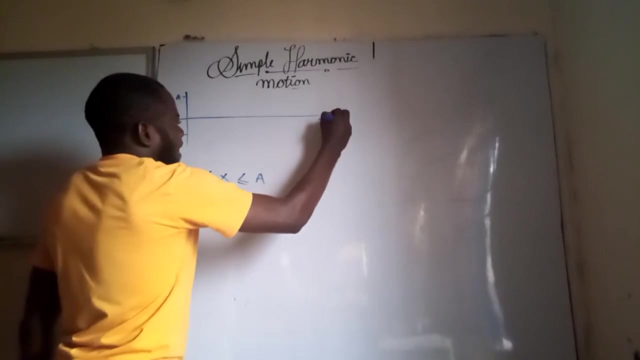 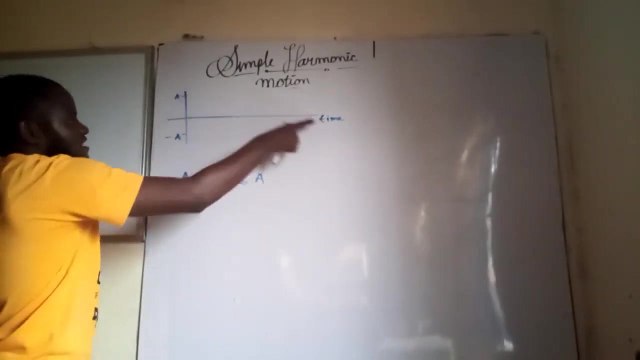 negative a and positive a inclusive, that is x can equal to a or less than a and also it can equal to negative a or greater than negative a. but it can't go beyond a. now, if i have my time at this horizontal level, if i plot the graph of a against t, that is the displacement against time. 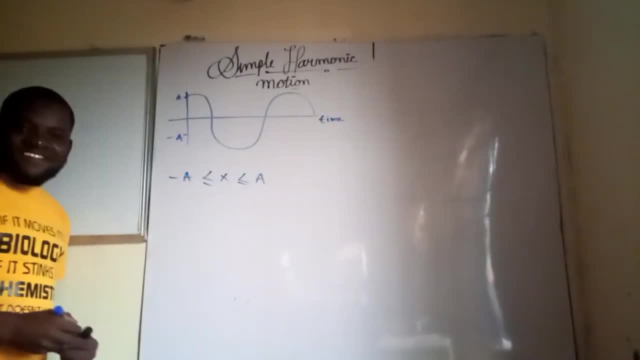 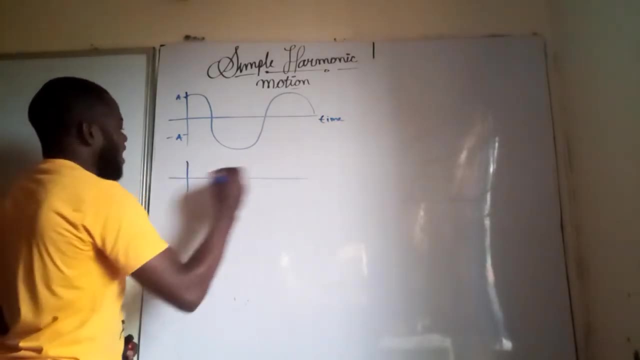 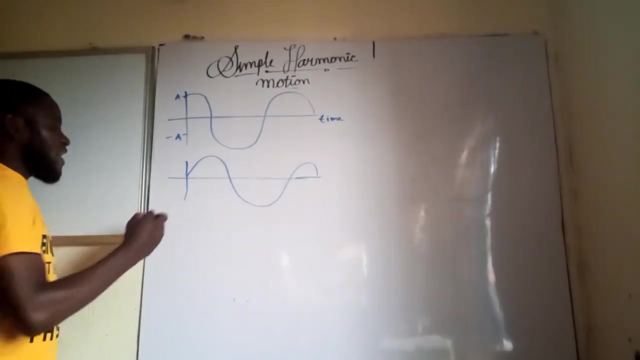 i'm going to have a cosine graph. i'm going to have a cosine graph if i start from there, but if i start from the equilibrium position, that is the middle, i'm going to have a sinusodial what graph. and i can also decide to start from this point here, which is going to give me a negative what? 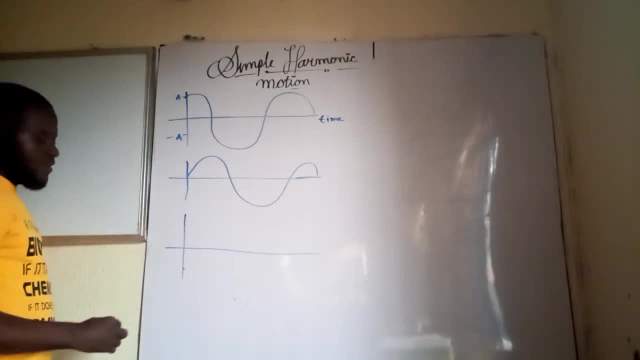 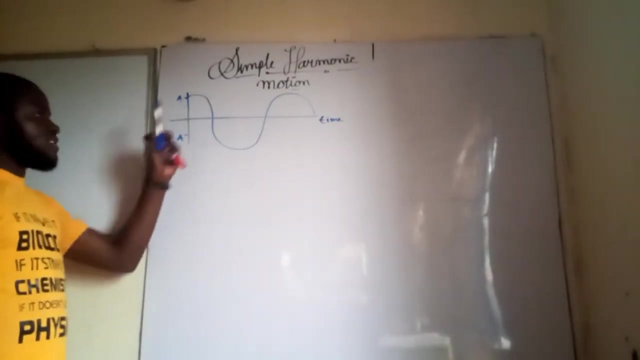 a negative cost function. so i will have this. this are we together? okay, don't let us go much into this now, just trying to show you the way we can have what this particular graph now how can we make use of this graph to find? so in case, 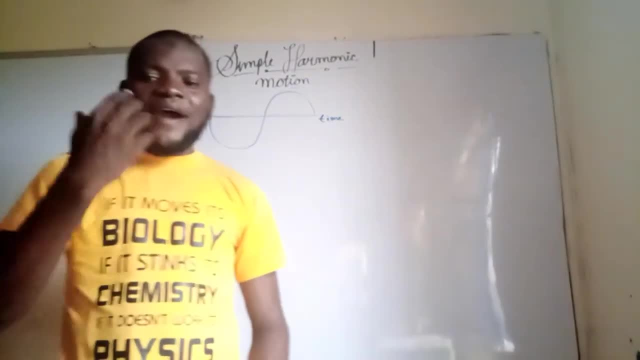 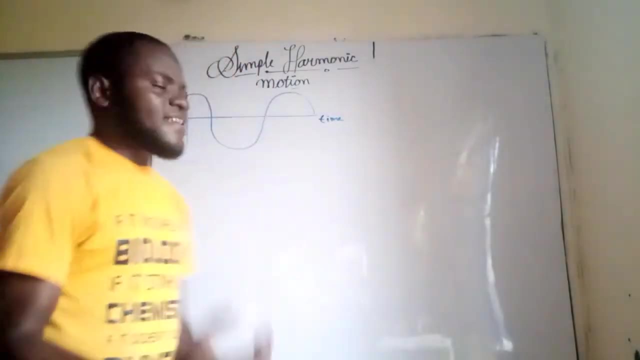 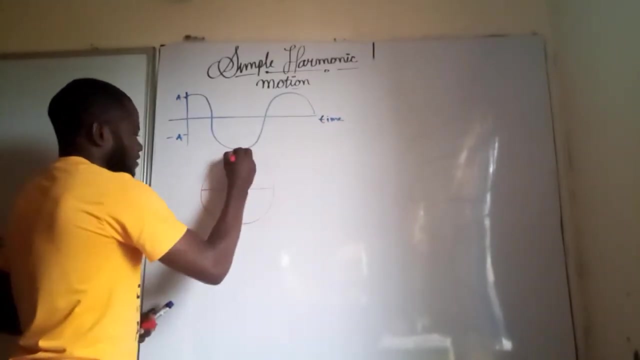 this graph is given to you and you have to look for maximum velocity. you also have to look for the maximum acceleration. how can you go about that? now, let's see. i'll quickly recall us back to this circle. remember, this is the circle we have initially, when we are talking about the period and 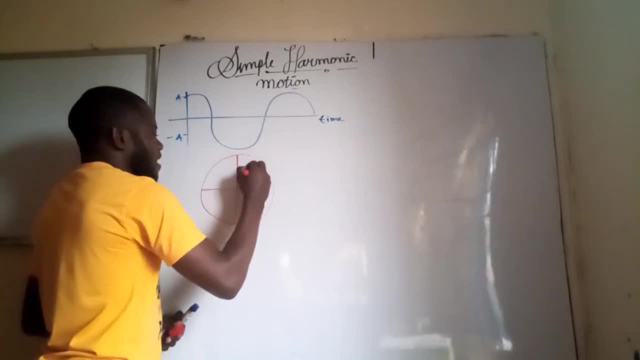 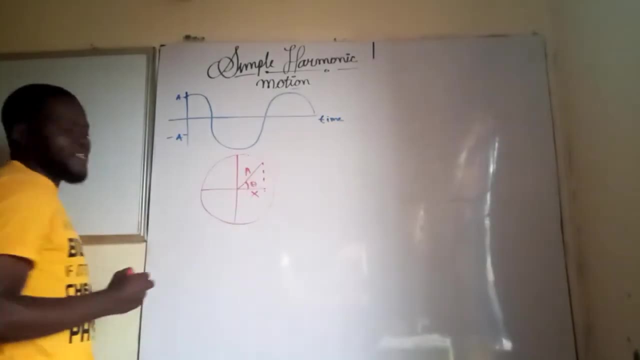 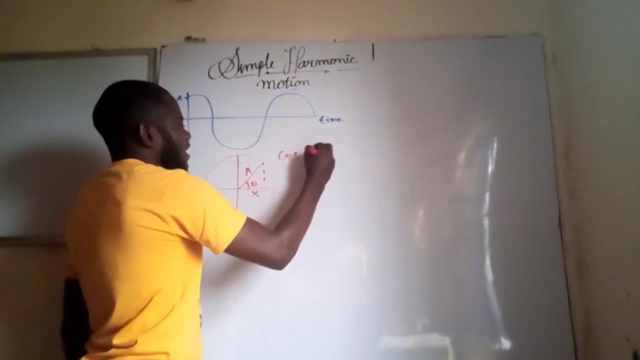 frequency, if this is our maximum displacement, and here is x. so this point here is angle theta. if i trace this down, this will be vertical axis. now from the trigonometry ratio i will have that the cosine of theta is x over a. if i cross multiply i have a cos theta. 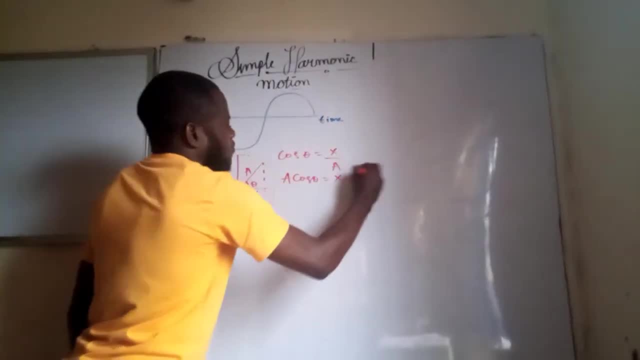 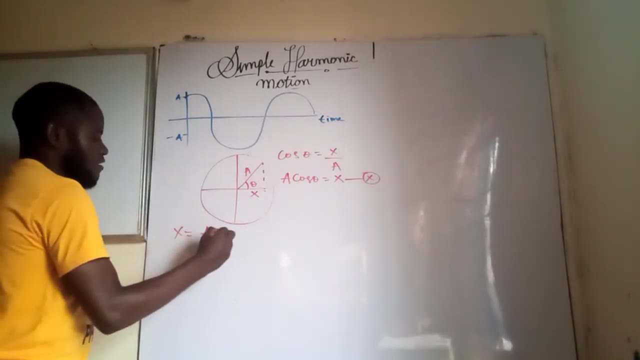 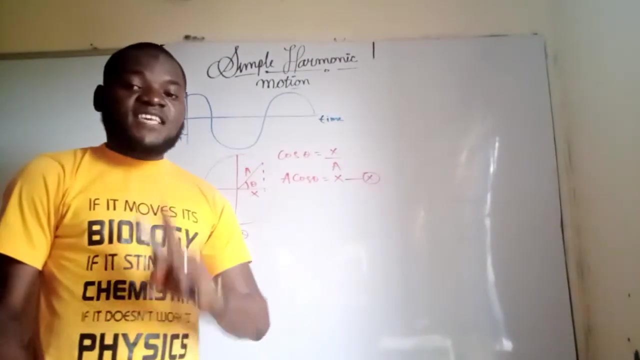 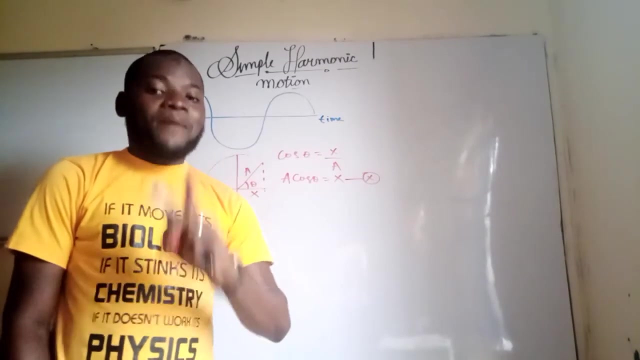 to equal to x. let's say this is our equation 10. if this is our equation 10, x is equal to a cos theta. now recall that the angular momentum is given as the angular displacement per capital, that is, the angular displacement per second. so theta is going to be omega t and our linear 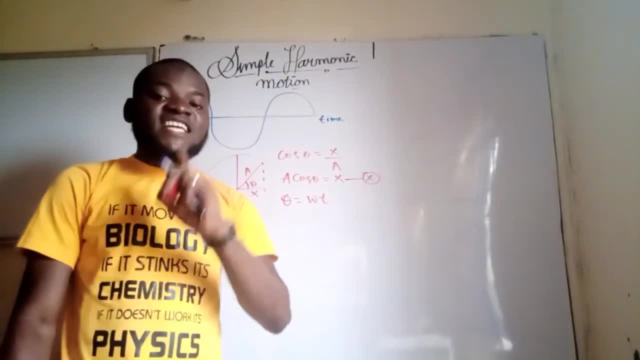 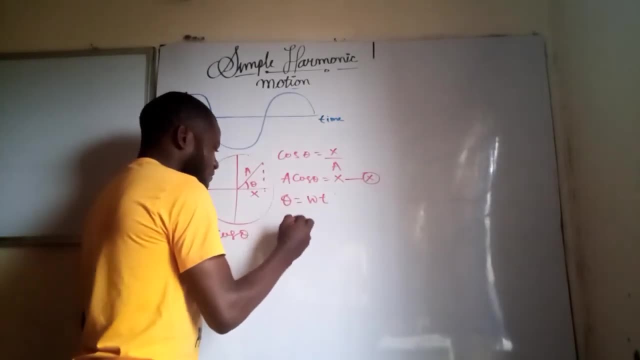 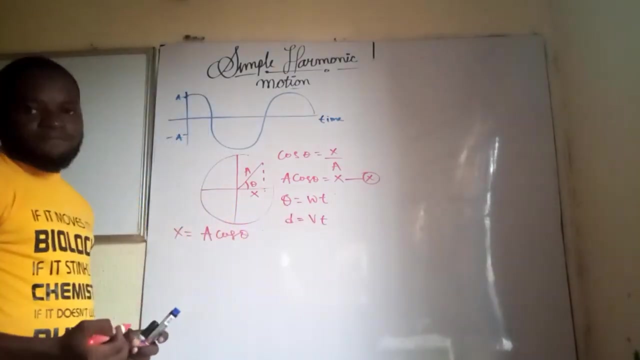 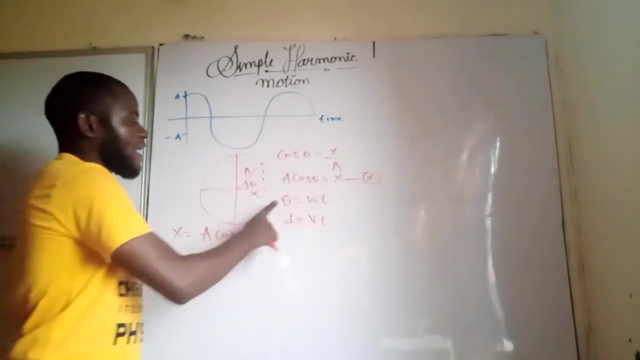 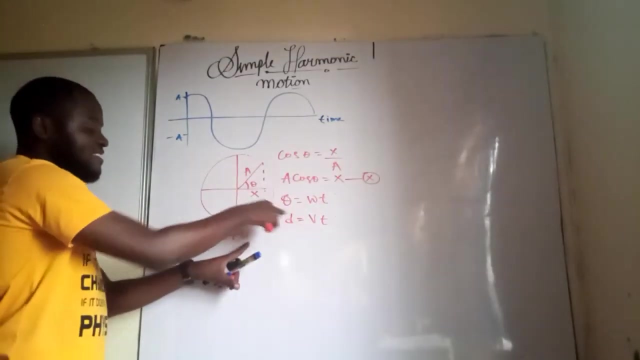 acceleration. sorry, linear velocity is going to be linear displacement per second. so our, our displacement, our displacement is going to be what vt- yes, our displacement is going to be what vt- while our angular displacement is omega t. now, if i replace this omega t, if i replace this theta with omega t, i'm going to have that x equal. 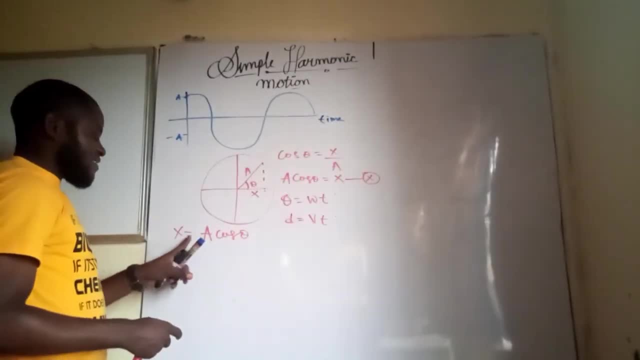 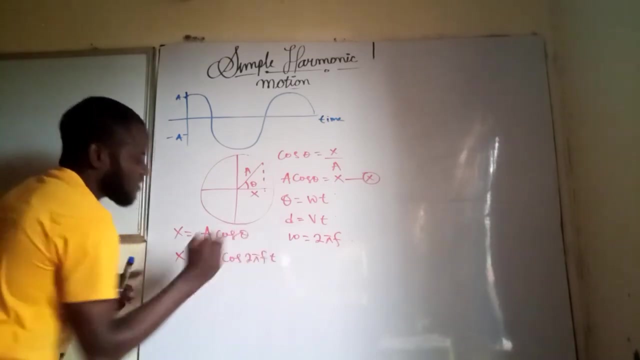 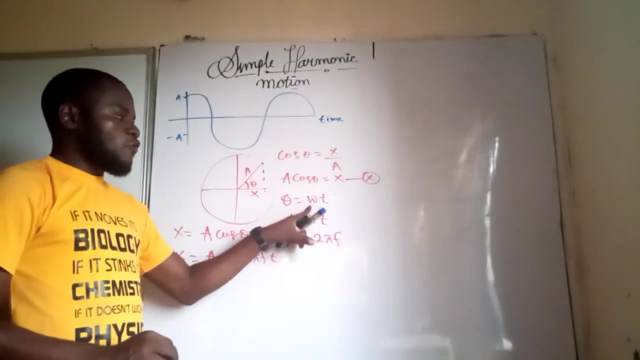 to a cos theta. instead of that i'll have x equal to a cos omega t, but before then omega is two pi f. okay, x is now a cos 2 pi F T, because theta is Omega T, Omega is 2 pi F. if you put it here, you have 2 pi F T. 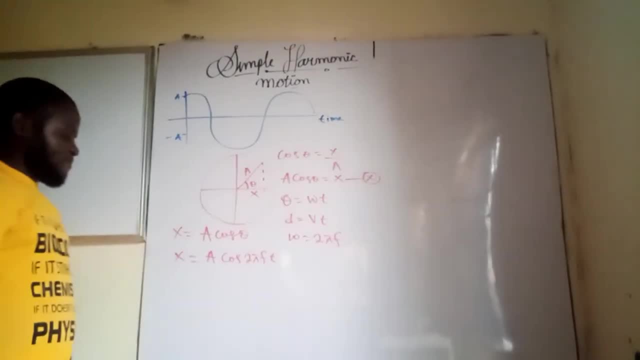 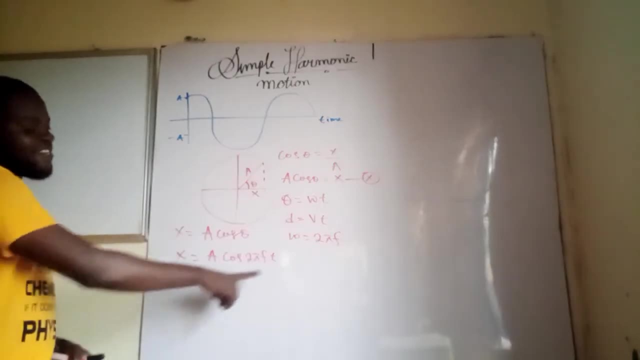 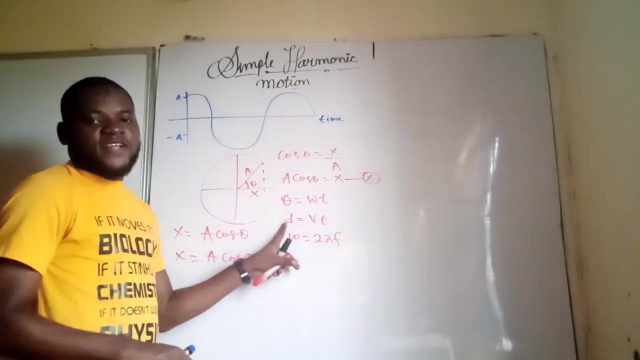 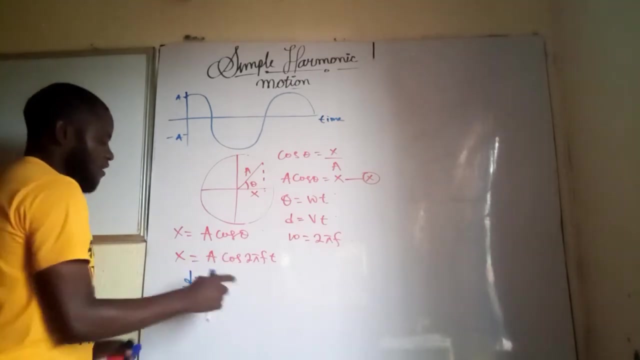 so use this to replace what theta, no qualms, okay, we are going to need the knowledge of calculus. of course, by the time you take the derivating of displacement, in respect to what time your result is going to the velocity, why velocity is equals to displacement over time. so the X, the X DT of this function, this is: 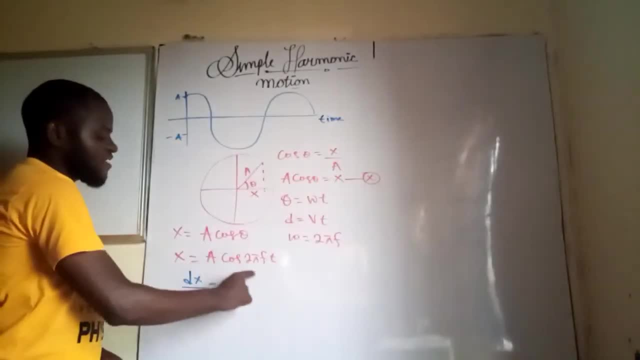 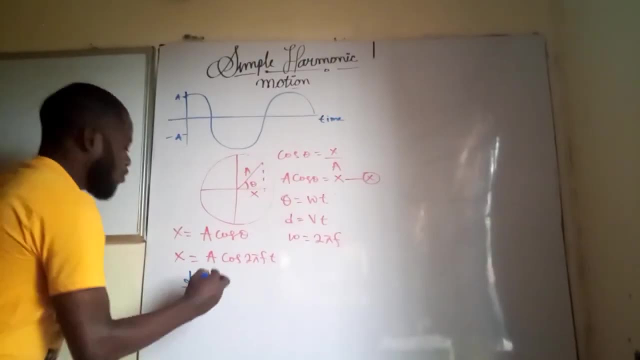 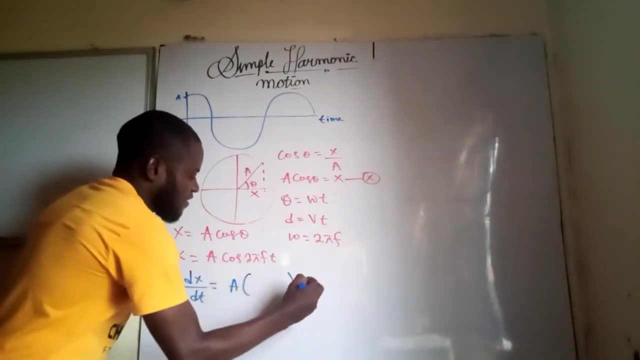 going to be a chain rule. I'm going to differentiate 2 pi F T first. when you differentiate 2 pi F T, your result is going to be 2 pi F. so I have a 2. it's okay, let me just write down. let this 2 pi F. let me bring it. here are we? 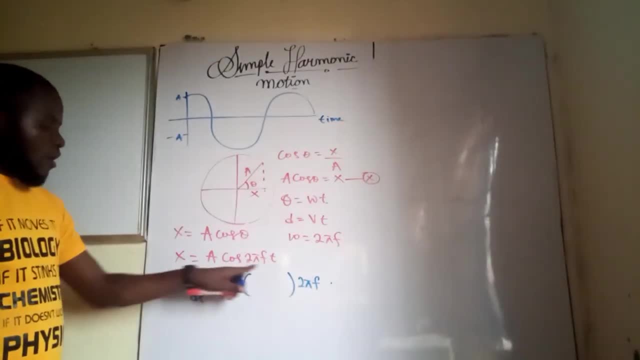 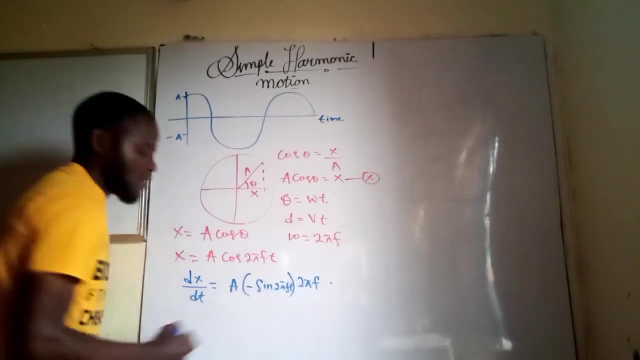 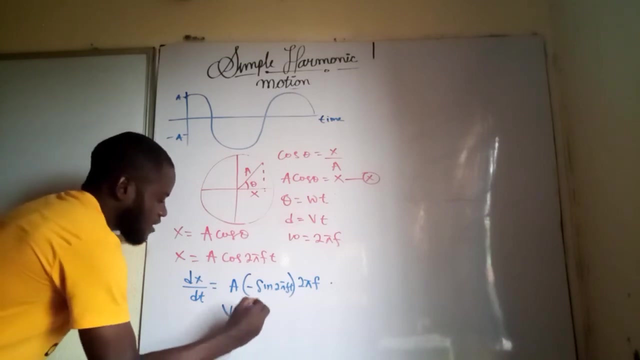 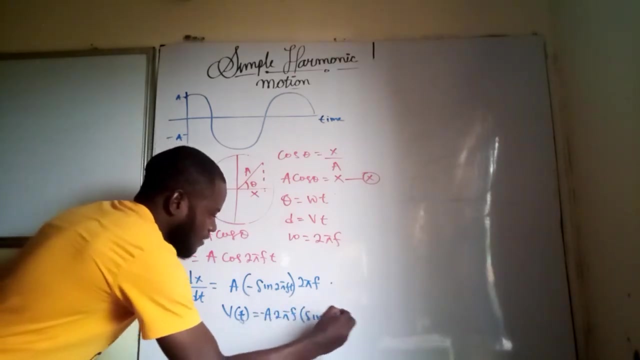 together. now I'm not going to differentiate cos of this. now the derivative of a cos is negative sine altogether. hence V, which is a function of time, is equal to a negative a, 2 pi F sine 2 pi F, T, the. we get this, but we are not done there yet. let's quickly come. 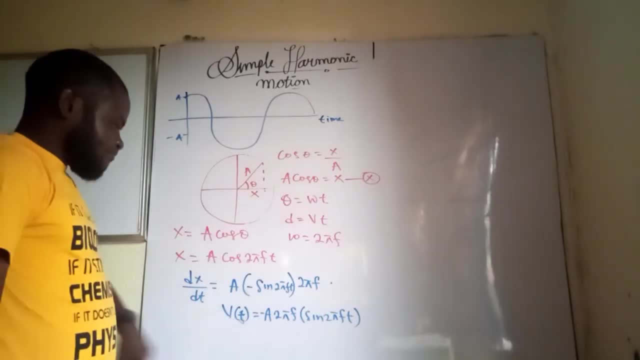 back here and see what we have here. so we are going to take the derivative of theta 0 and take theренal. you won't see it here. so everything have the heading no or be silent, nothing like that. so we are going to be here for a very long time. 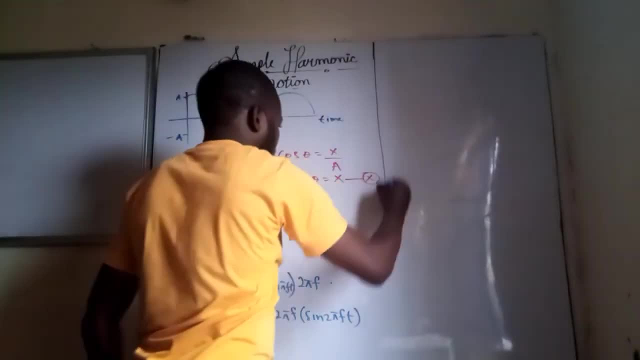 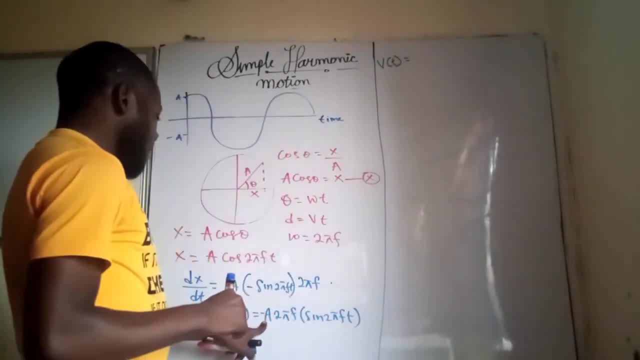 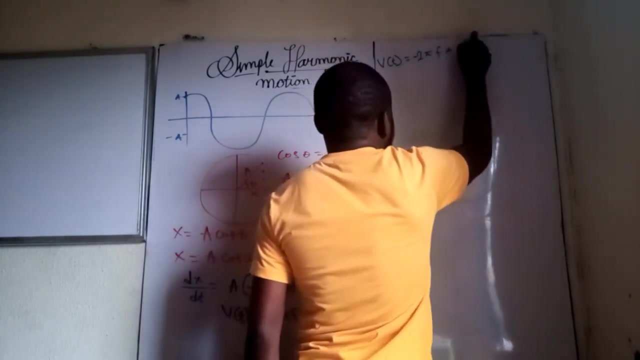 now we have the two, must throw the two measurements of f. so if aáng loves�incarnation F as an ordinary different, then the instant must die. if aang does not want of the mechanics of Whose was interview木朱? 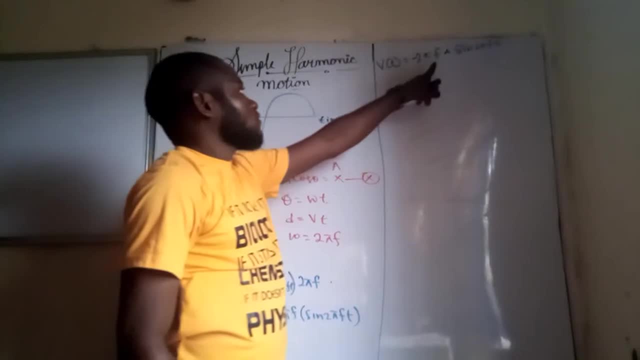 but rather we are going to. this is function is given or swap. let's see our V of E. remember a is we are less a 2 pi F negative, 2 pi F E sine, 2 pi F T. if this is what we have now, what is our f, our f? 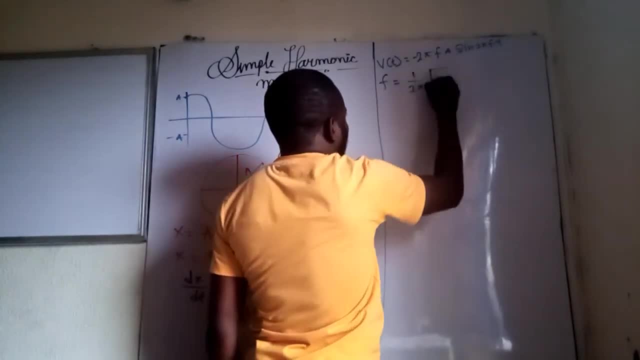 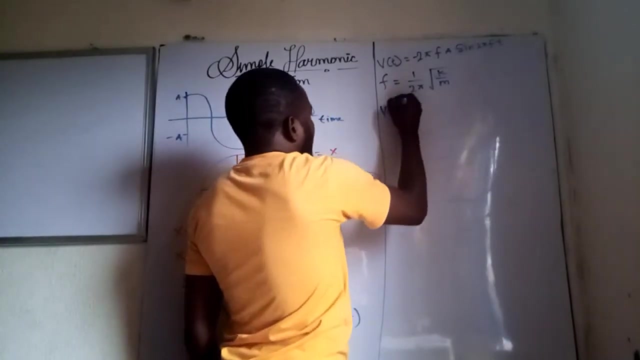 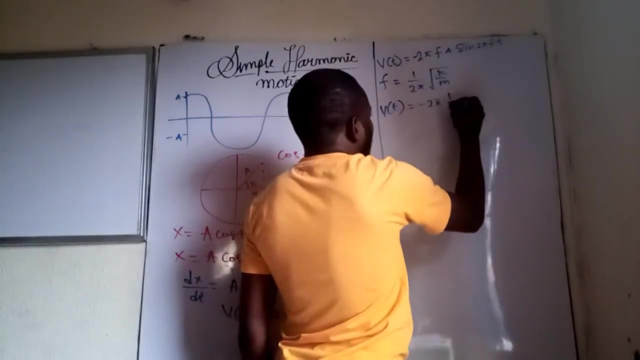 is given as 1 over 2 pi, the square root of m. sorry, the square root of k over m. that's our f, isn't it? so let's plot this into this. we have that v of t is negative 2 pi times 1 over 2 pi, the square root of k. 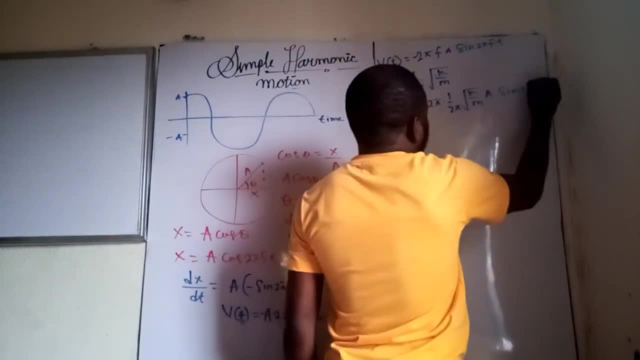 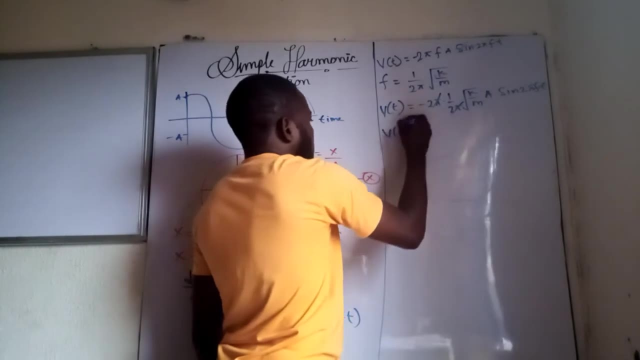 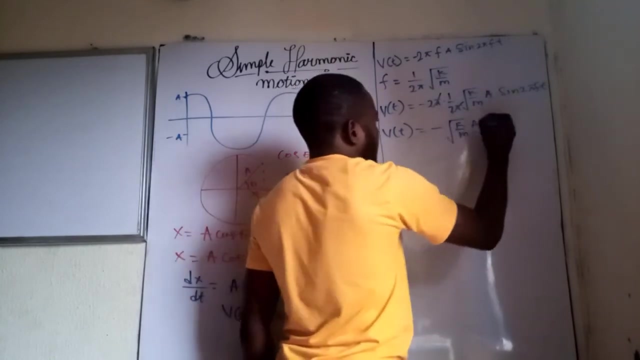 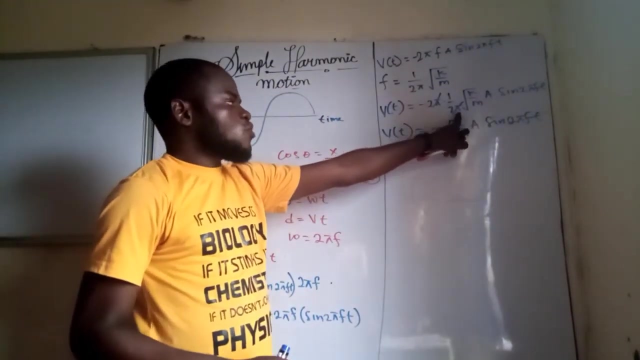 over m a sine 2 pi f t. this and this would cancel. if this and this should cancel, v of t is equal to negative. the square root of k over m times a sine of 2 pi f t. now, remember that the square root of k over m times a. 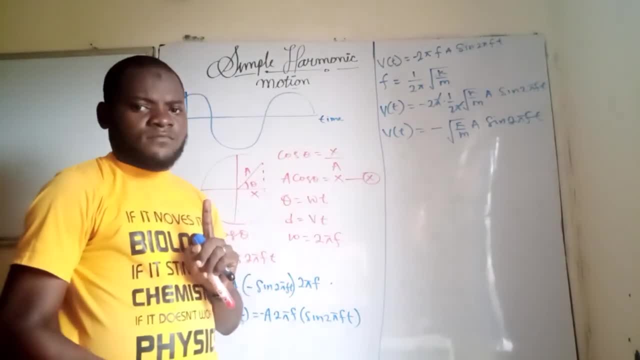 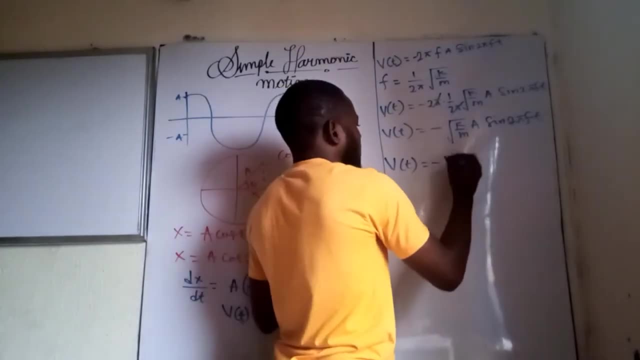 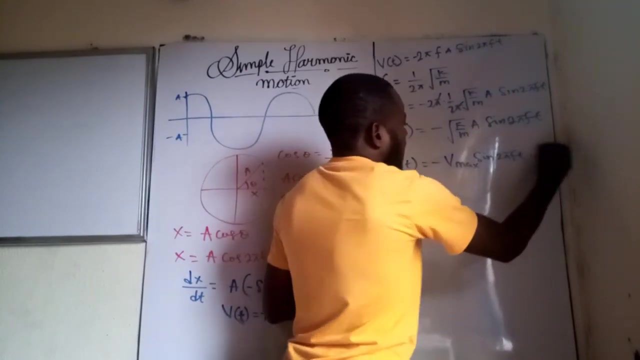 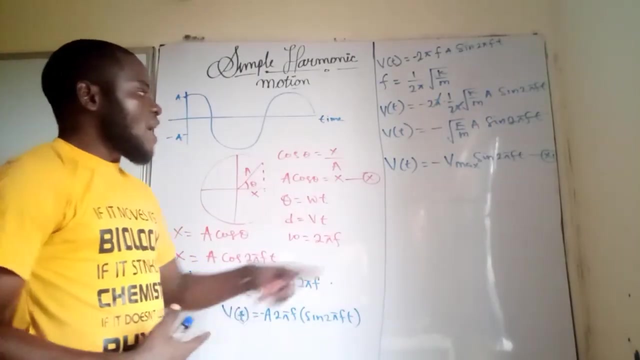 is the same thing as maximum velocity. do you agree with me? if yes, the velocity as a function of time is negative: v max sine 2, pi, f, t, equation 11.. so we cannot look for acceleration now. remember, acceleration is the derivative of velocity with respect to time. 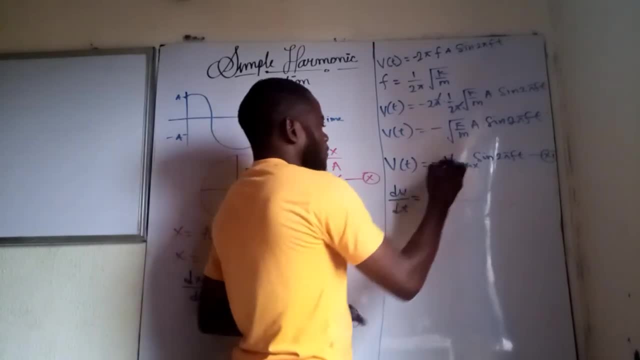 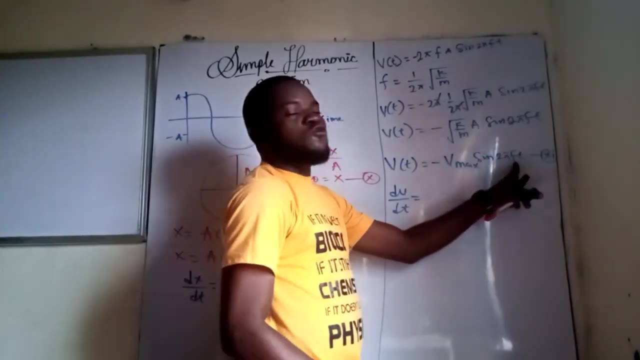 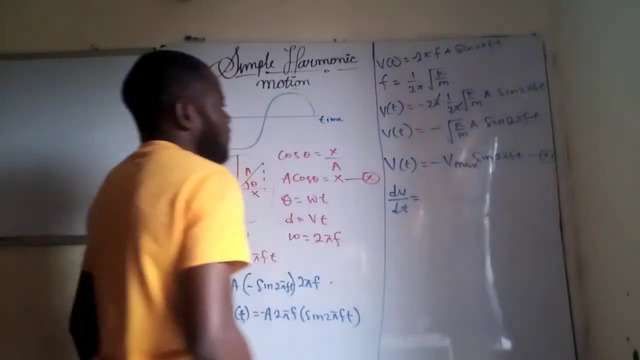 so we have dv dt to equal now at this junction. now i have to differentiate this one again. if i differentiate this, i'll still have 2 pi f, right? so okay, don't let us start from here. we are going to run into trouble if we start from here. let's just let's. 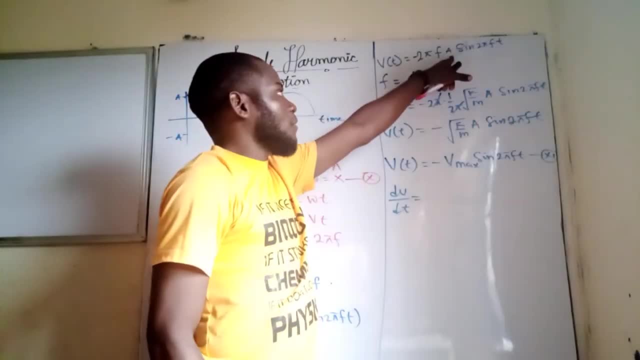 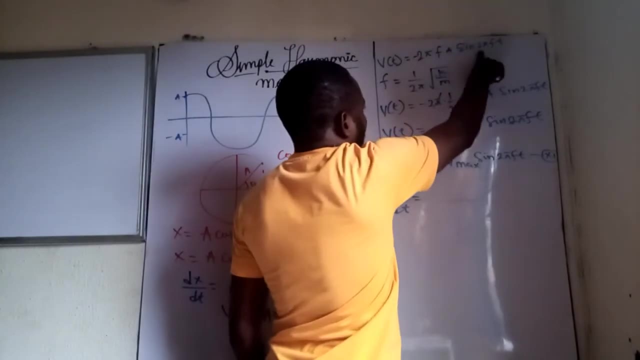 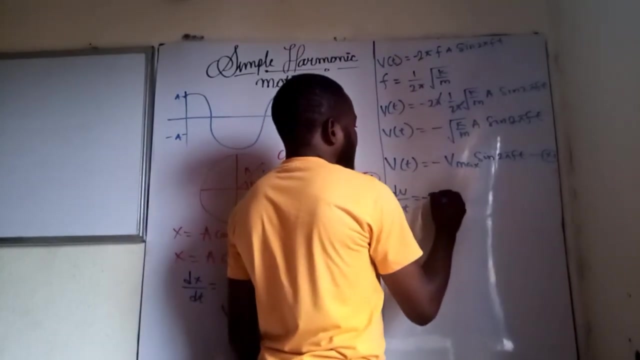 start from this point. here are we together. okay, if i start from this point here, i will have that. this now is going to be 2 pi when I different 2 pi f when I differentiate it, so it is to multiply this, i'm going to have negative 2 pi square. 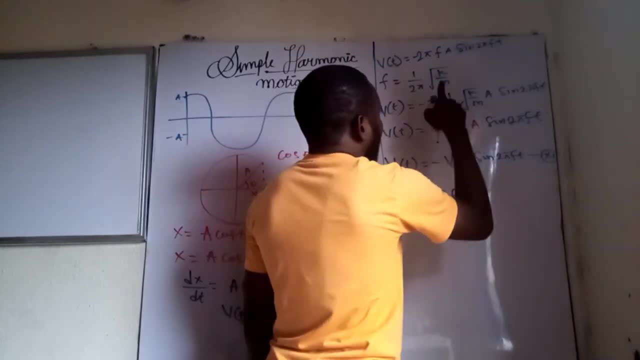 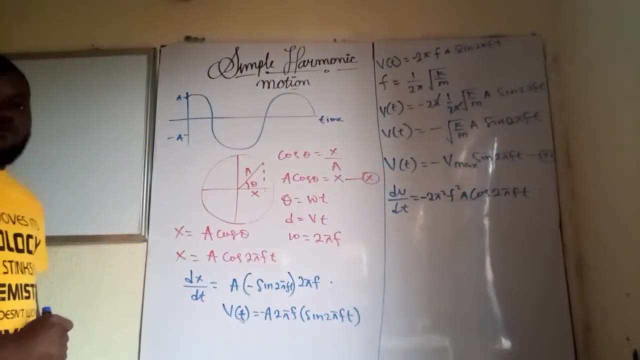 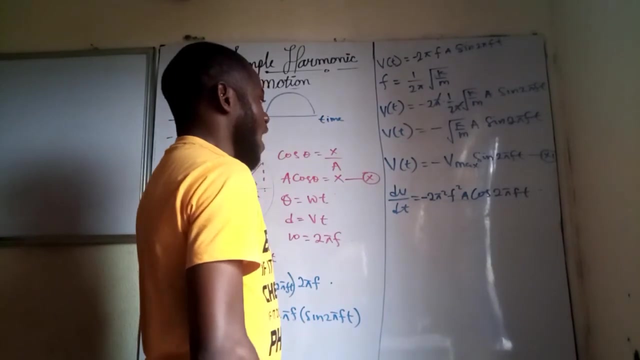 f square times a, and this is going to be cos of 2 pi f t. that's what the derivative will give me, so you can lay your hand more on calculus. okay, now let's see. let's see what will happen there. if this is F square and this is 2 PI, 2, 2 PI. 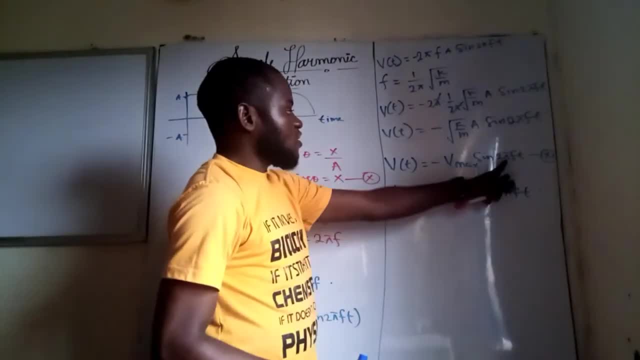 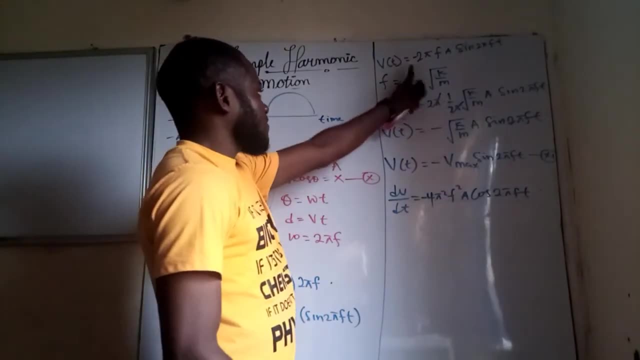 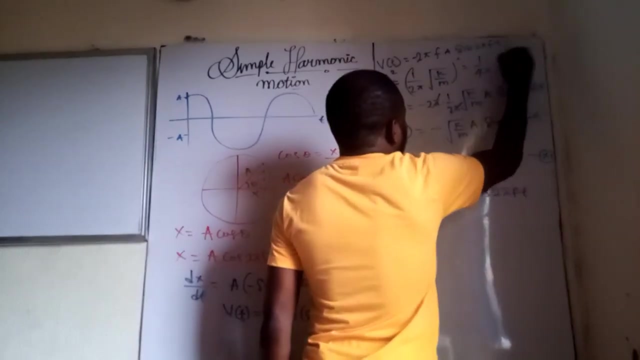 square, so this supposed to be 4 PI square. sorry, because these two will multiply these two also. yes, yes, sorry for the mistake. now, if I square this, if I square this equation there, my result will be 1 over 4 PI K over n, is that?